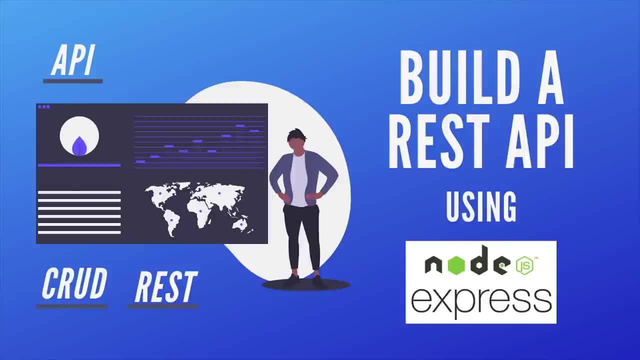 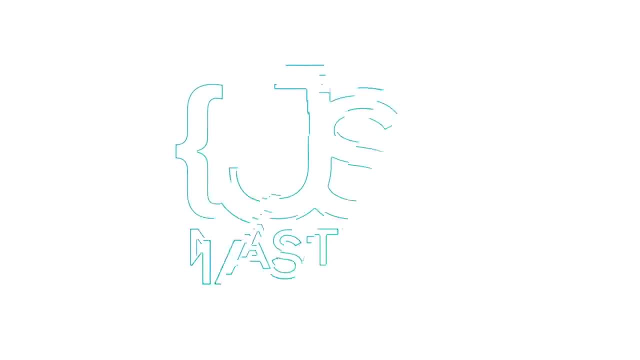 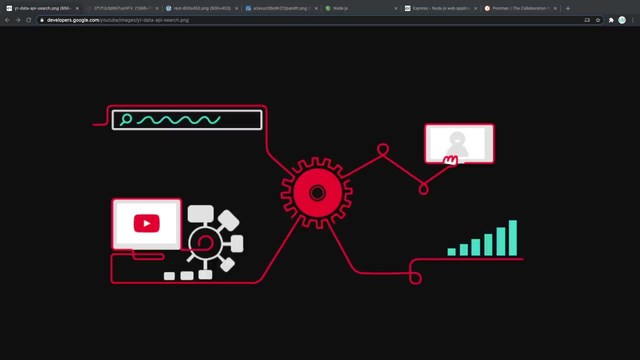 architectures and methodologies. I'm here to show you how all of that works in practice, so that you can build your own APIs. Let's dive right in. Let's say you're trying to find videos on YouTube. You open up YouTube, type something into a search. 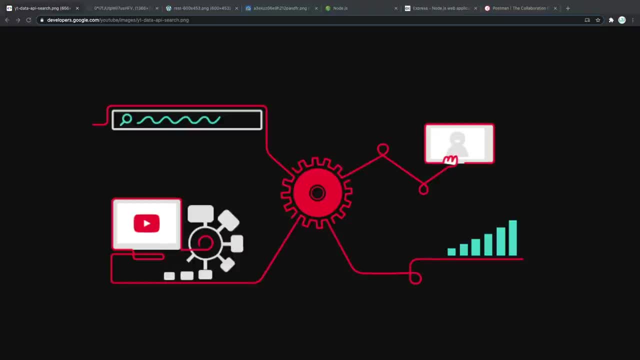 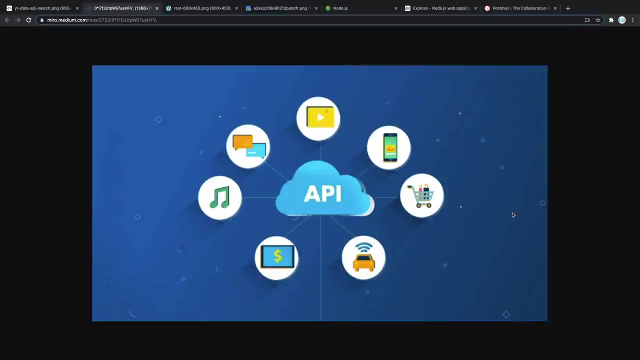 bar and hit enter, And then you see a list of videos about that search term. A REST API works in a similar way. You search for something and you get a list of results back from the service you're requesting from. An API is an application programming interface. It is a set of rules that allow. 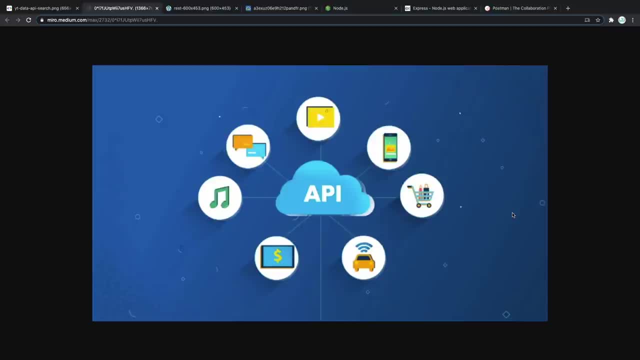 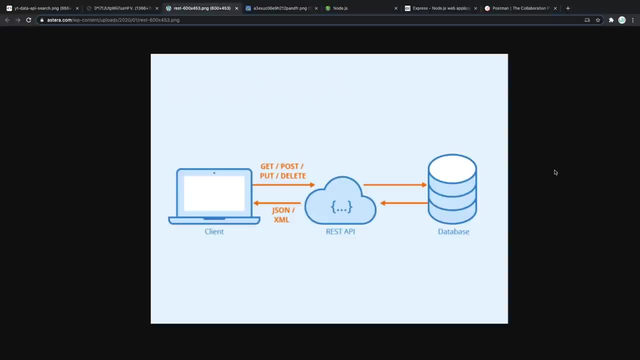 programs to talk to each other. The developer creates the API on the server and allows the client to talk to it. REST determines how the API looks like. It stands for Representational Data Transfer. It is a set of rules that developers follow when they create their APIs. 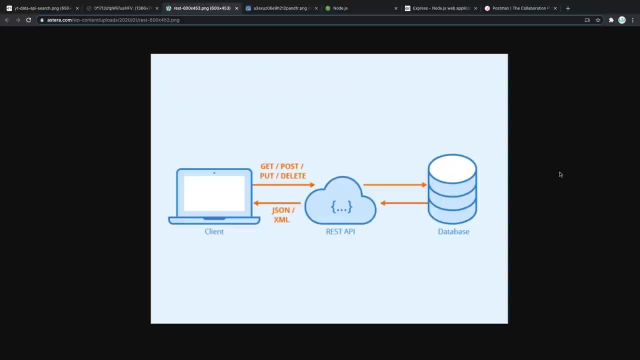 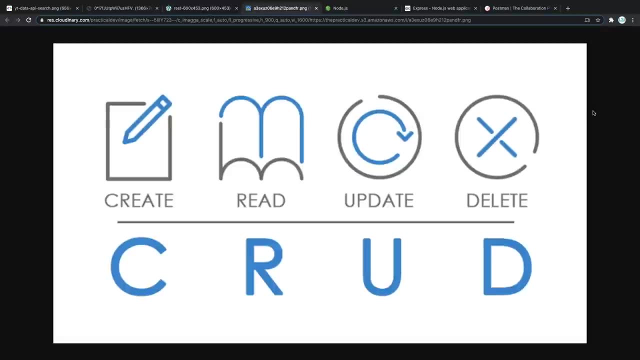 Nowadays, almost all APIs are REST APIs, so don't worry about that too much. And finally, what is CRUD? CRUD is an acronym for Create, Read, Update and Delete. It is another set of rules we are going to follow while building our API. Almost every website is a CRUD in a sense. 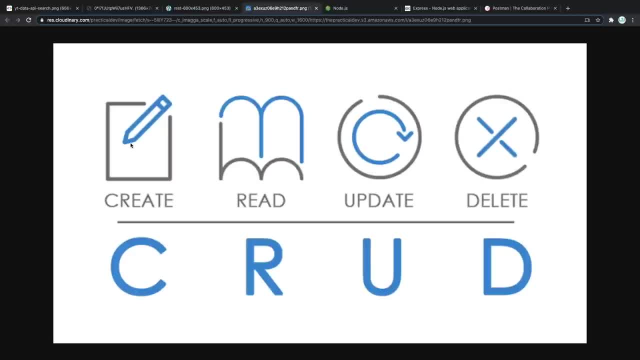 For example, whenever we have a database of users, we need to be able to create a database of users. We need to be able to create a database of users and create a database of users, We need to be able to create user accounts, get or read the profile. 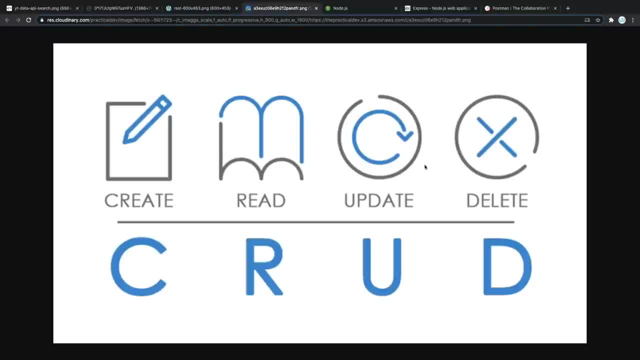 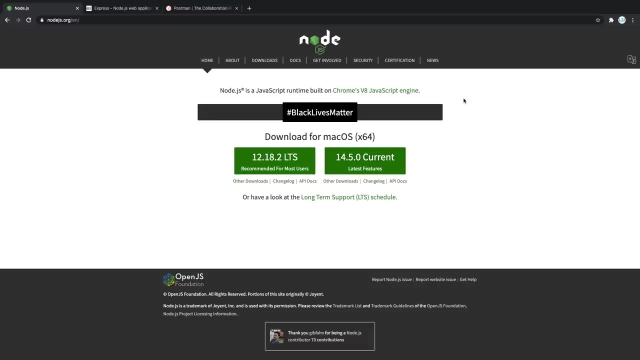 details, update the profile details and finally delete an account. This was just a short theory introduction, but, as I said at the beginning, I'm here to show you how all of that works in practice, so that you can build your own APIs. Now let's start coding. First, we need to download Nodejs. 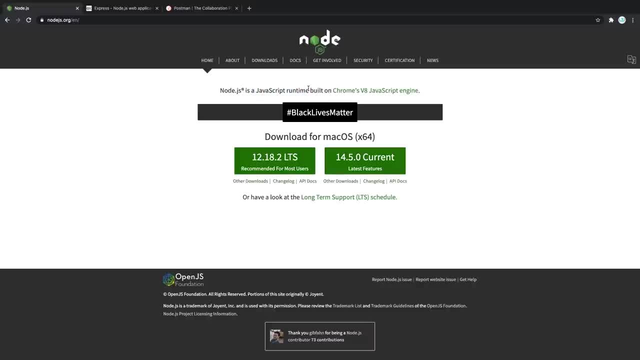 Nodejs is a JavaScript runtime and all that it does is it allows JavaScript to be run in places other than the JavaScript runtime. So we need to create a JavaScript runtime and we need to create a server-side JavaScript application. If you worked with Frontend so far, 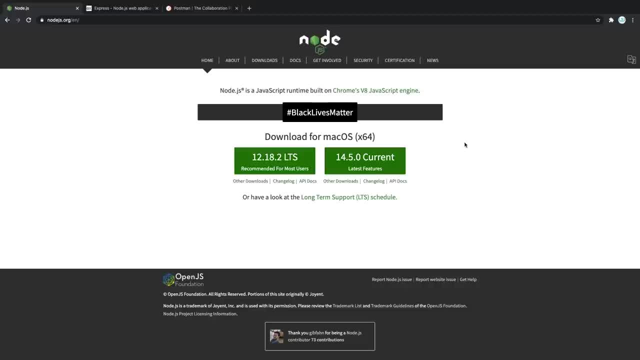 this is going to be something that's completely new to you, But don't worry, this video is for everyone who is just starting with Node and Express and has never built their own API before. So now, how do we download it? Well, 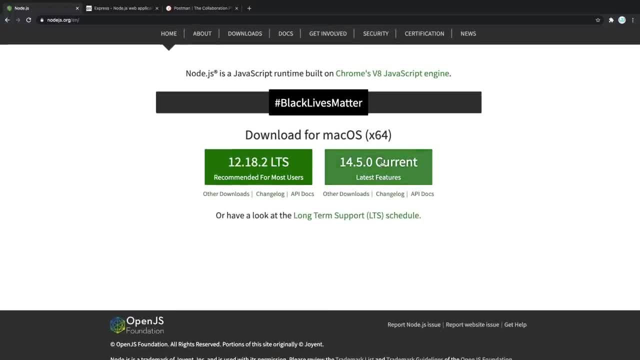 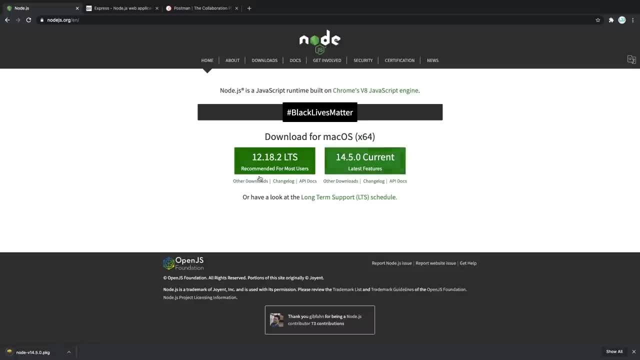 we just click this button. I would recommend downloading the new current version, because there we can use imports and exports. So just do that. Even if you do have it installed already, just install it one more time and then you can check for your version once we go to Visual Studio. 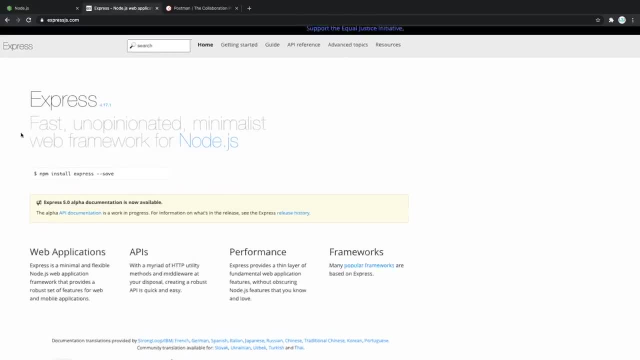 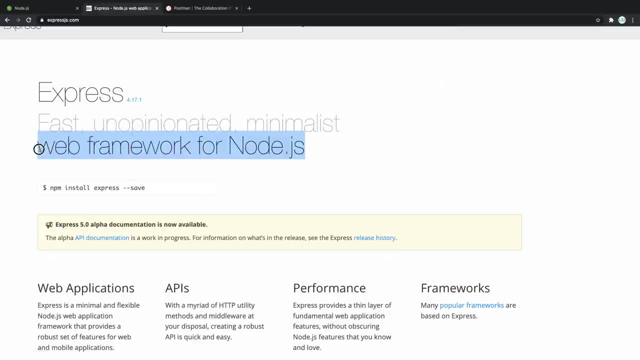 Code. Secondly, we'll be using Express. Express is, as you can see, fast unopiniated, minimalist web framework for Node- Just keep in mind these last words. So it is a framework for Nodejs. Express is going to help us create different routes for our API. And finally, 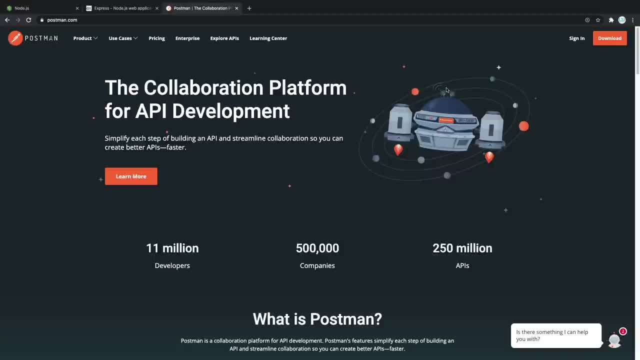 we'll be using Postman. Postman is going to help us make different requests to our APIs so that we can test all of our endpoints. With that out of the way, let's move to Visual Studio Code. Right now I am inside of Visual Studio Code in an empty folder. It's called Node Express API. 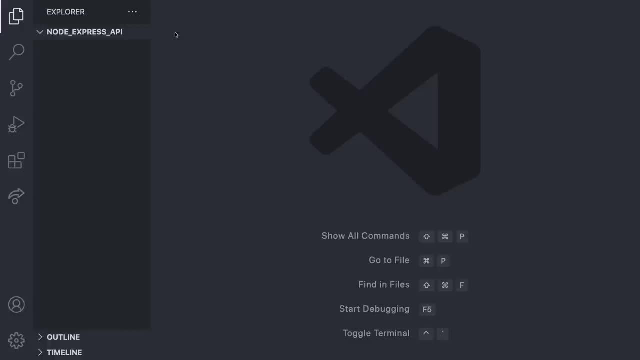 You can create your own empty folder and just drag and drop it into Visual Studio Code and we should be good to go. I prefer Visual Studio Code because it has a nice built-in terminal we're going to use. So if you go under View at the top, 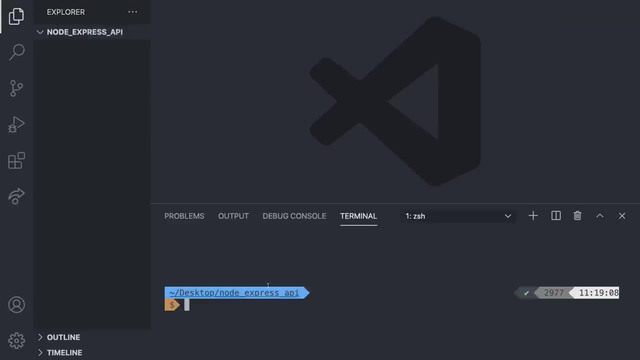 and then Terminal. the terminal is going to show up and then we can run some commands right there. So what do we need to do to initialize our back-end JavaScript application? You can run npm init and then put a flag of y, just like this, and then click enter. This is. 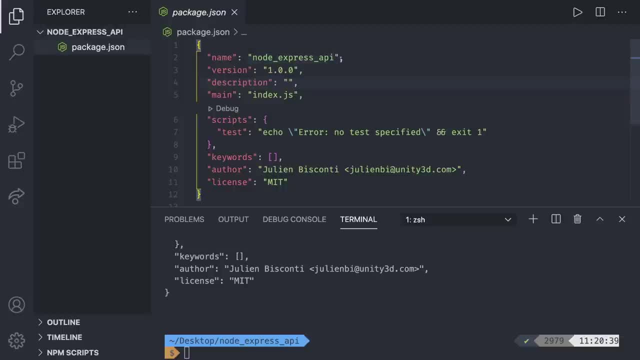 going to create an empty packagejson with barely something in it. We have the name, we have the version description and the main file which we are going to create right away In here. you can see that we do have some scripts. Later we're going to add our own. 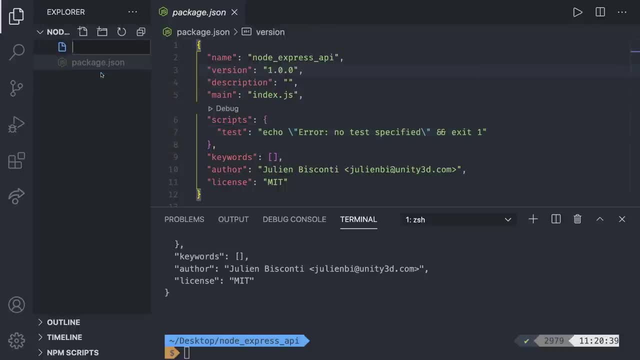 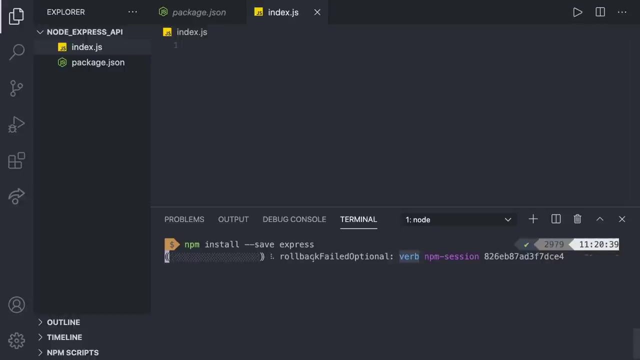 starting script. With that out of the way, we can create an indexjs file which is going to be the starting point of our server. Inside of here we'll be using Express, So let's install it right away: npm, install, dash, dash, save and just express: like. so It's going to install and then 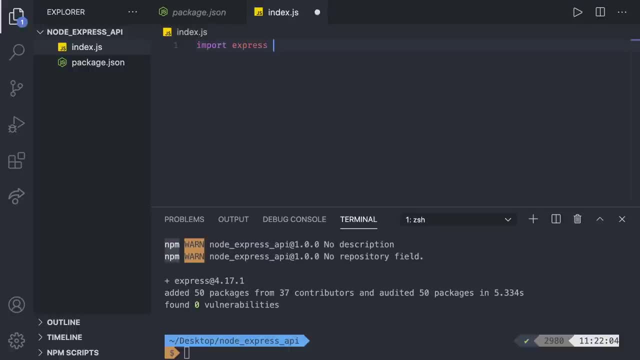 we'll be able to do import express from expressjson. Before we had to do something like this. const express is equal to require and then in here we put the express. These two are equivalent. Right now you should be running the latest. 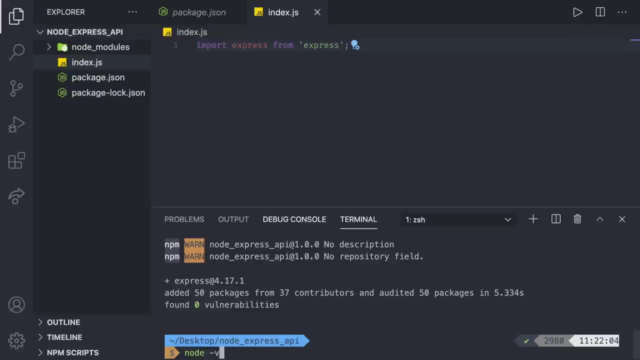 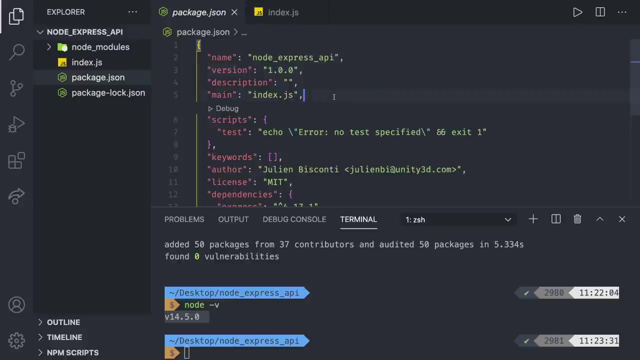 node version So you can type node and then dash v in the terminal and you should be getting 14.5.. If you have that installed, then we can go back to the packagejson and just add one simple thing that's going to allow us to use the imports That something is going to be type. make sure to use. 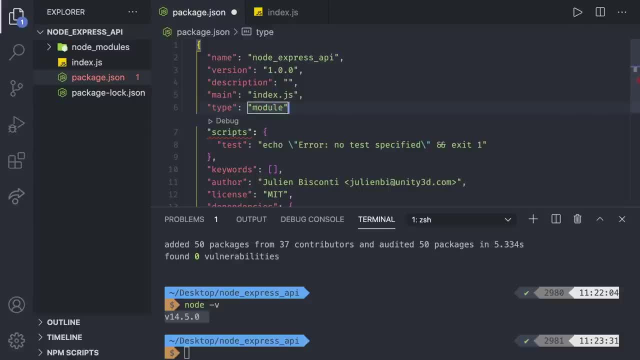 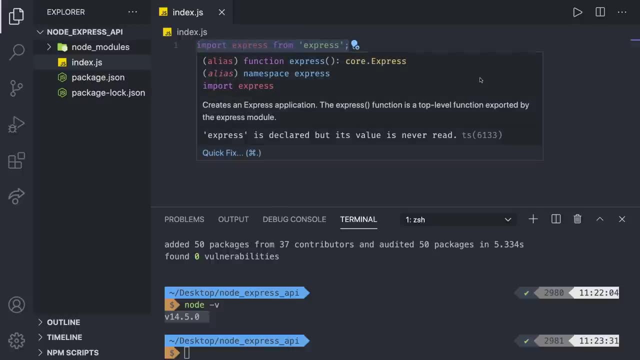 double quotes equal to module. As soon as you add this, we'll be able to use normal, or let's say, newer, import statements like this, Great. The second thing we're going to need is going to be import body parser from body dash parser, Just like this. This allows us to take 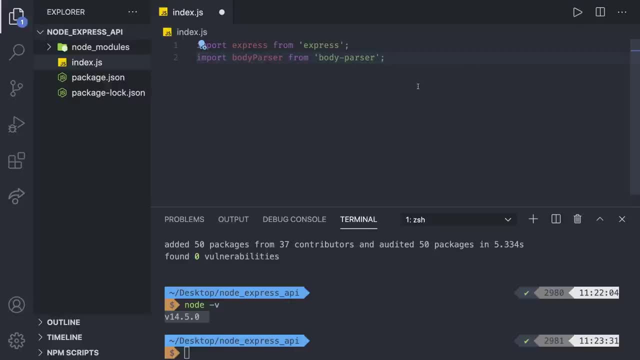 in incoming post request bodies. Again, that sentence maybe doesn't make a lot of sense right now, but you're going to see it in action really, really soon. Then we need to initialize our express application by doing const. app is equal to express and we call that express as a function. 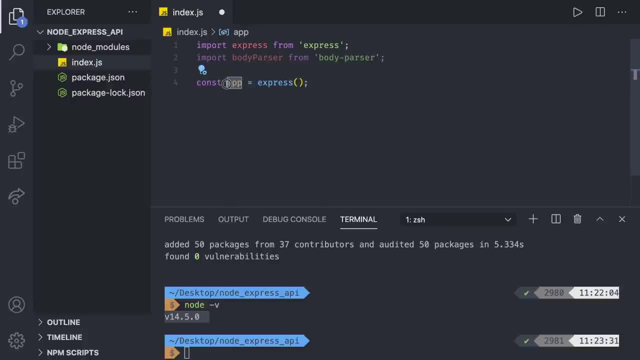 Now our whole application lies in this little variable. Below that we can specify the port of our application. We can use capital letters because we are never going to change this port, Since frontends are often on local host. 3000,. 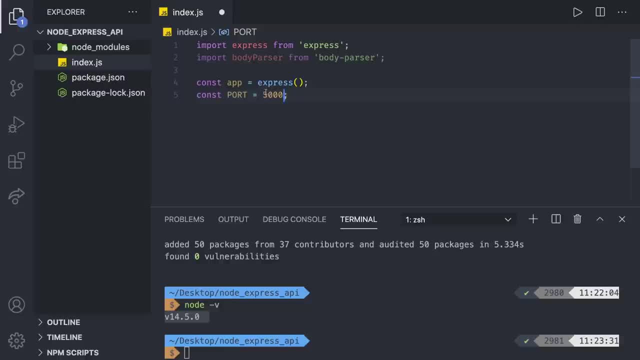 let's use 5000 for backend. Of course this can be any number. Then we can initialize the body parser middleware by doing something like appuse. Then in there we do body parserjson, We call it as a function. This is just going to say that we're going to be using JSON data in our whole. 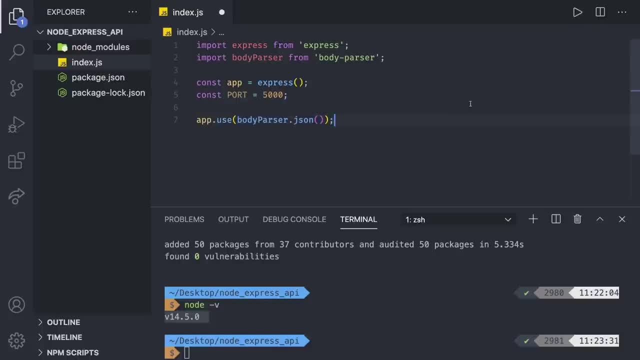 application. This is just going to say that we're going to be using JSON data in our whole application. JSON stands for JavaScript Object Notation and it is a common format for sending and requesting data through a REST API. Don't worry about the syntax, because a JSON object looks like a. 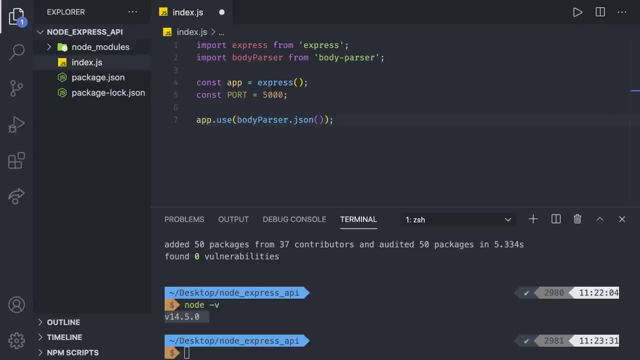 JavaScript object, so you're going to be completely at home with this. There are some small differences, though, In JSON: each property and value must be wrapped with double quotation marks instead of single quotation marks, but that's just it, And finally we can make our application listen for. 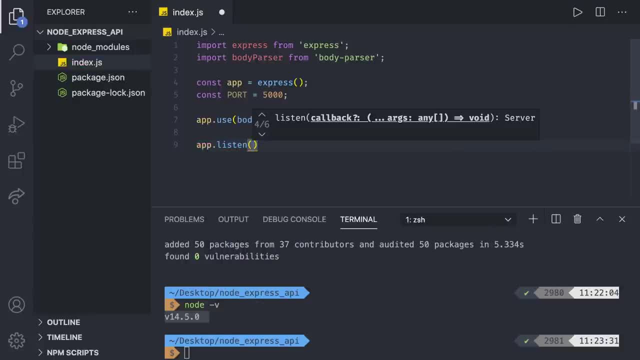 requests by saying applisten. In here we specify the port we want to listen on and then we create a callback function which is going to be executed once we run the server. Okay, in this case we're just going to have a simple consolelog, consolelog- and we're going to say server running. 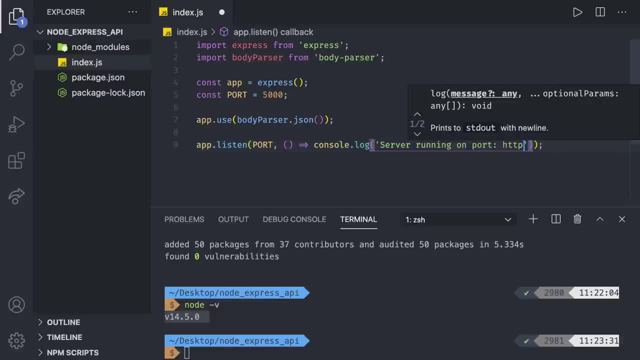 on port and then that's going to be HTTP. Make sure to do HTTP and not HTTPS: Forward slash, forward slash localhost and then in there we can use the template strings to put the port in inside like this, but make sure to change this from regular strings to template. 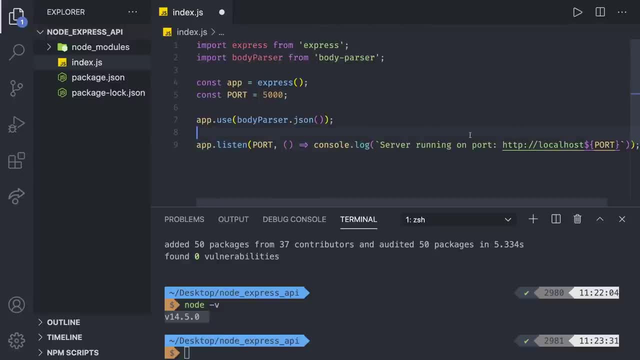 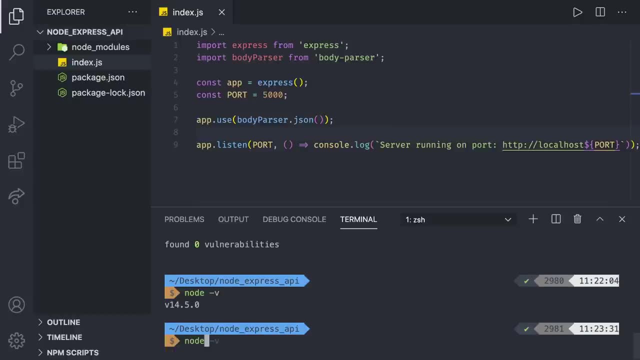 strings using the backticks, just like this: Okay, now our server is ready and we can actually run it. So right now, if I do node and then run our indexjs like so, it's gonna say: server running on port is equal to localhost 5,000,. and I just noticed we are missing a small detail right there. 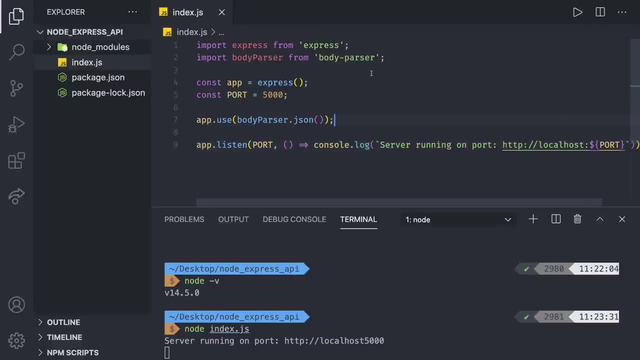 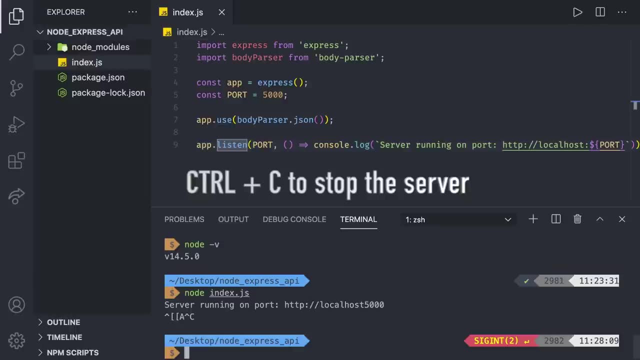 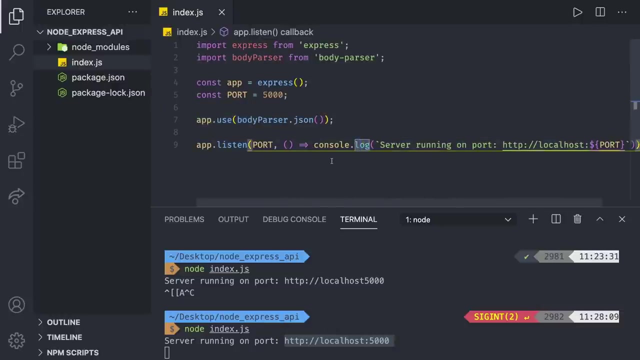 it should be localhost with a colon just after it. So now, if we save, notice how nothing is happening in the console. That's because once we run it, we need to rerun it one more time every time to get the changes, as you can see right there. Now we can click it. That's the problem. we don't want. 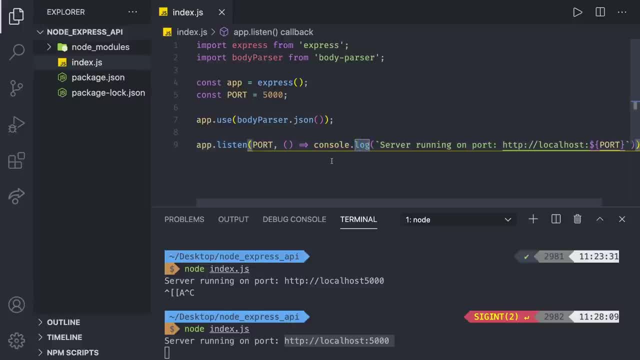 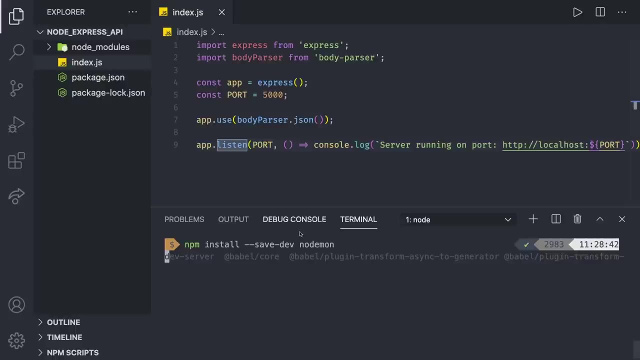 to save the file and then every time close the server and then run it again for changes to occur. why we have a package called nodemon. we can install nodemon by typing: npm, install dash, dash, save dash, dev, and then we can say nodemon. why did we use the dev? well, because when we push or 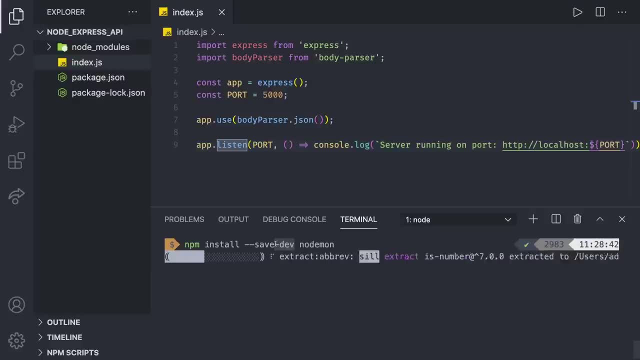 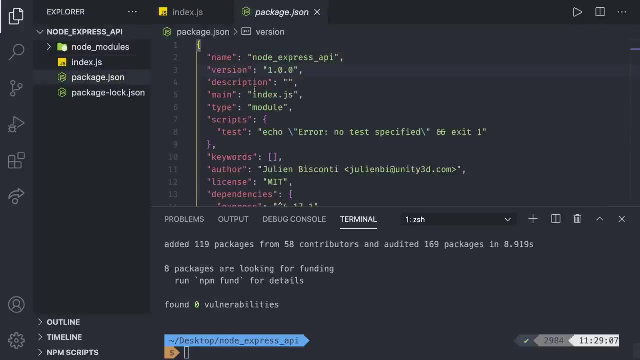 publish our application. no one is gonna be running our server, so we are installing this dependency only for our own development purposes. it's not gonna be used later. that's why we have it as a dev dependency now. if you go back to our packagejson, you should be able to see dependencies. 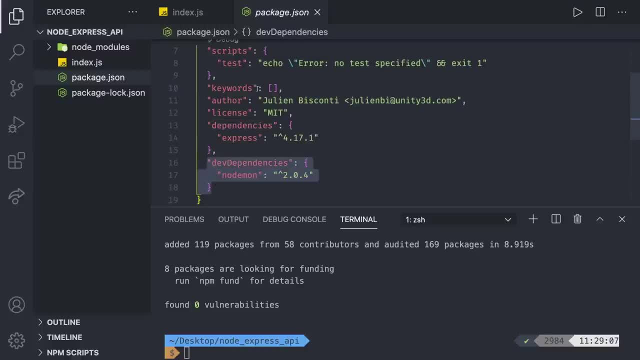 express and dev dependency, nodemon- great. so how do we run our application with nodemon? well, let's set up a script. in here we're gonna remove this test script, create our own start script so we can say start and then just after it we need to use double quotation marks, and in here we'll just do nodemon. 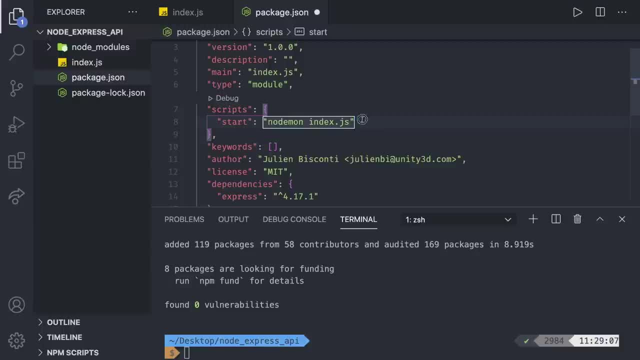 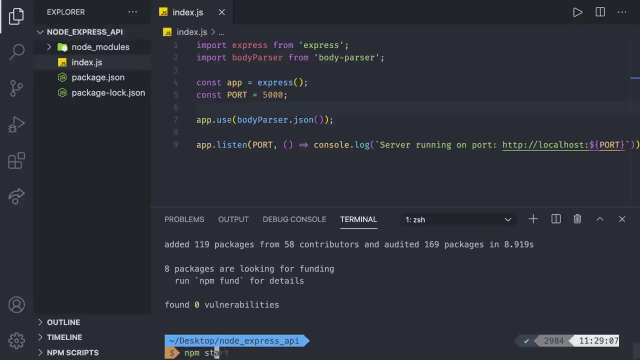 in indexjs. this is going to make sure that we start our application using nodemon and, as i said, nodemon is going to keep making changes whenever we save a file. so if we now save this, go back to our indexjs. let's try running our npm start command. okay, great server running on port localhost. 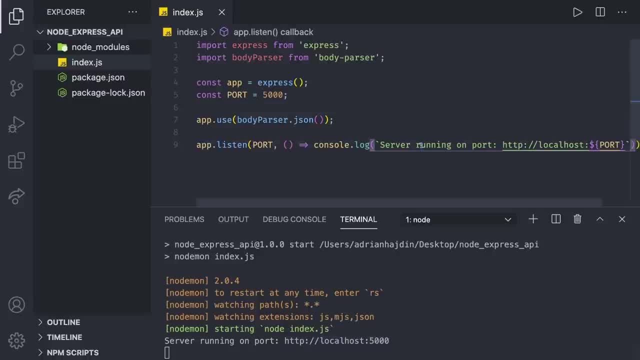 5000, and if i was, for example, to change this r to capital r and then save the file, you can see nodemon restarting due to changes and then starting the server again and we do get our change right here. that's amazing. we just set up a basic express server, so what can we do with it? 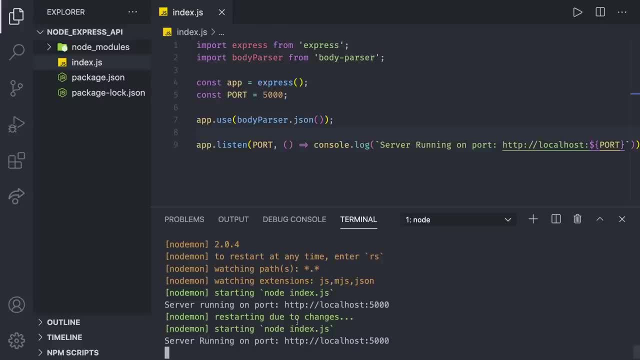 now that our application is running, we can visit our api by going to http, localhost 5000. you can control or command: click this or copy it and paste it into a url bar. if we go there right now, we do get some kind of an error. cannot get forward slash. 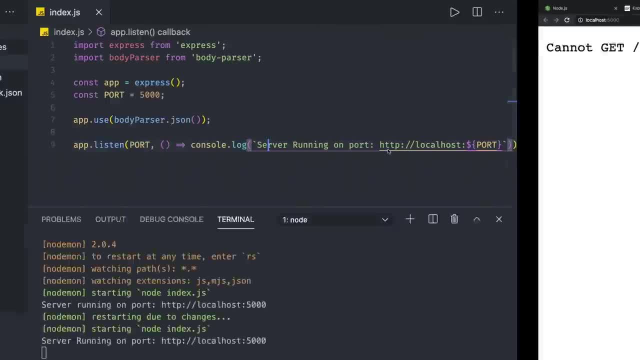 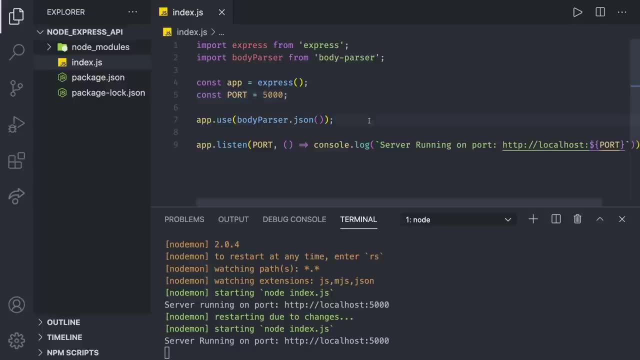 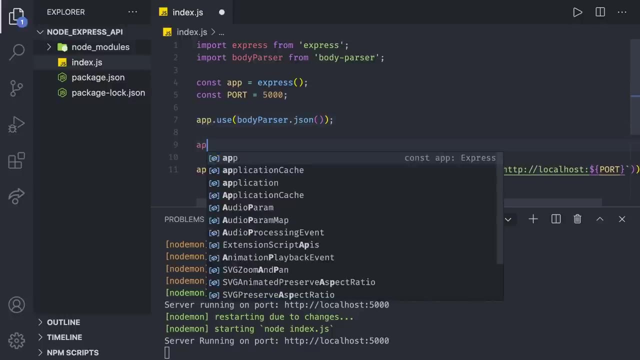 slash. why is that happening? well, if we go back, node and express, primarily, are all about routing, so we need to create some routes which we can then visit with our browser or we can send requests to. so in this case, we're going to create our first route that's going to be appget, as you can see. 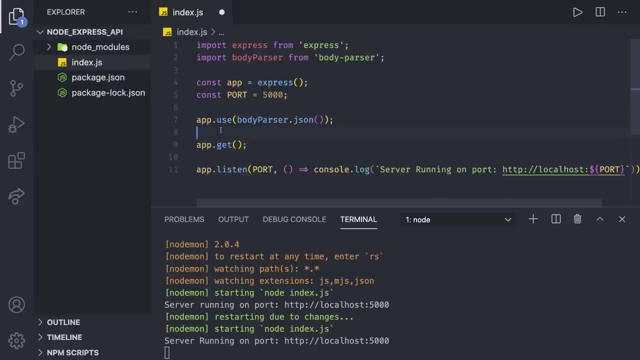 we can create different routes of different types right there. if we do dot and then something- in this case we are expecting a get request- and then the first parameter is the path we are expecting that request to. in this case, this is going to be a get request to the forward slash or the home page, then the second: 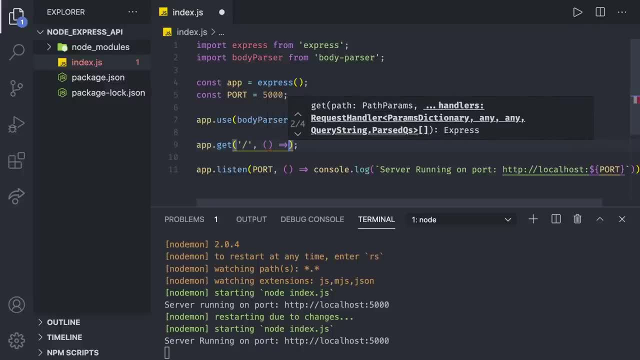 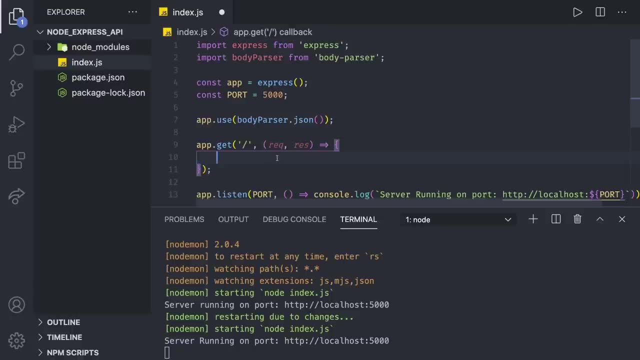 parameter is the callback function. we can do it like so, callback function. it accepts two parameters- request and response- in here let's do a simple cons log, just so we can see if it is running. so let's do, um, let's just do this test just like, so it's really noticeable all uppercase. and then also let's do rest that send. 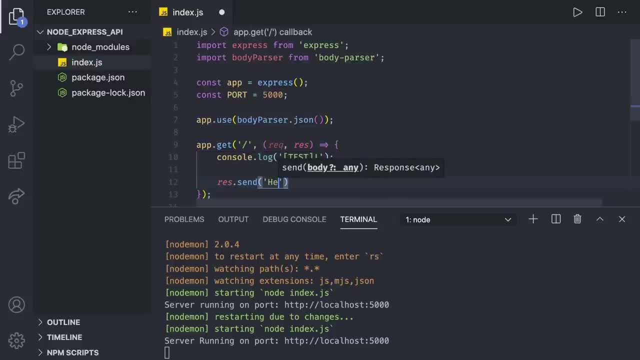 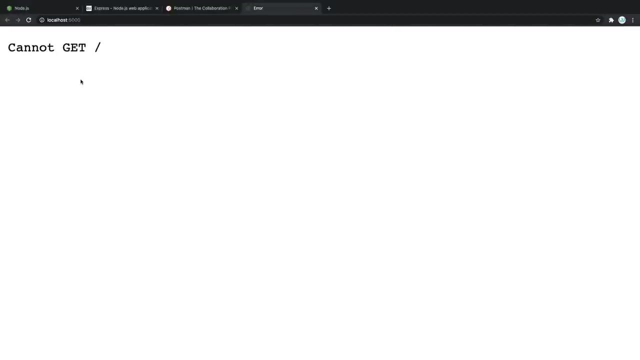 so we'll do rest that send and we will say hello from home page, just like that. whenever we have just a root page- this one here- that usually means that it is a home page. so if you now save this and we go back to our home page, feel free to refresh, and we do get hello from home page. 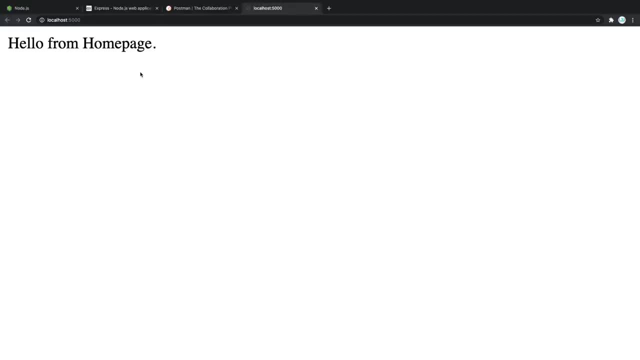 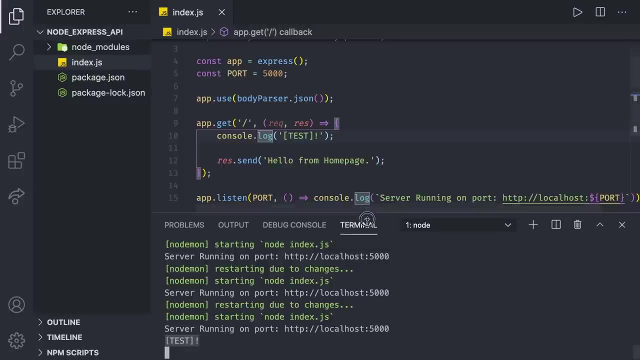 that's not the only thing that happened. the console log is not going to be in the chrome's console, rather it's going to be right here. as you can see, we do get console log of test with an exclamation mark, which means that the code from this callback function was ran once we visited the 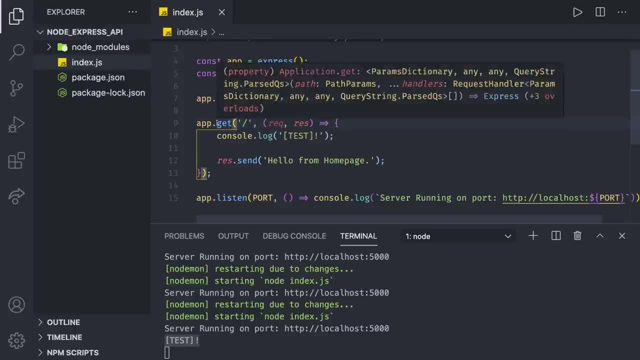 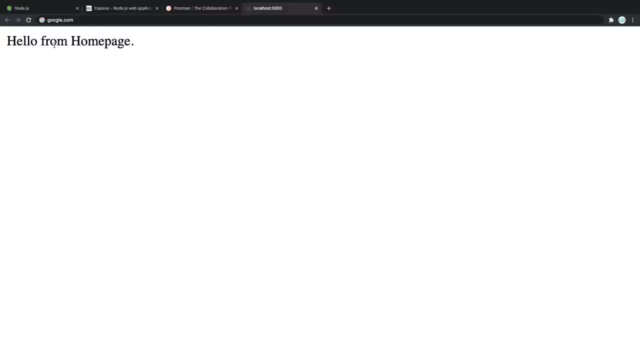 forward slash. when i say visited, i mean we made a get request to the forward slash. remember, browsers can only make get requests. for example, if you visit googlecom, you are making a get request to the googlecom domain. the same thing happened here. we visited localhost 5000 and that made the get request to the slash. 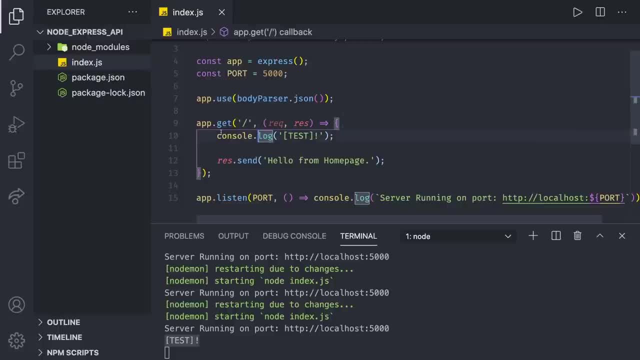 or just to the home root route. of course, our api is going to have many more routes, so right now we can delete this, we can just have the ressend and since this is only one thing, we can immediately leave it in a short arrow function syntax, amazing. so let's go ahead and let's go ahead. 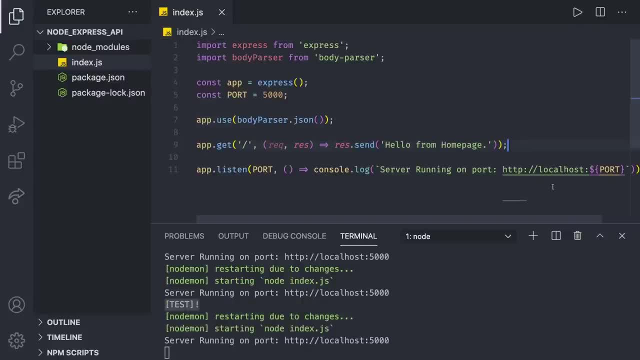 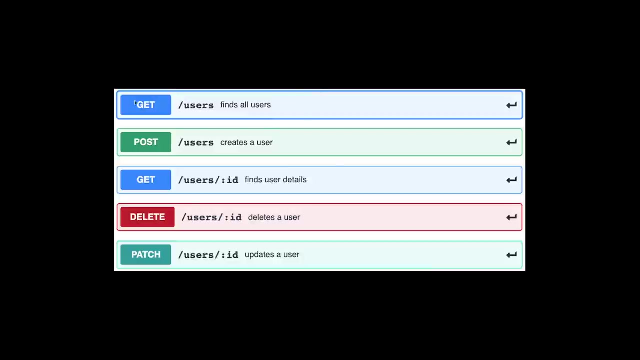 and let's do that. so what is our api going to do? well, we will be handling some users. handling users in a database is a great example, because that is something you're going to be using in each and every application. this is how it's going to look like. we're going to make five different routes. 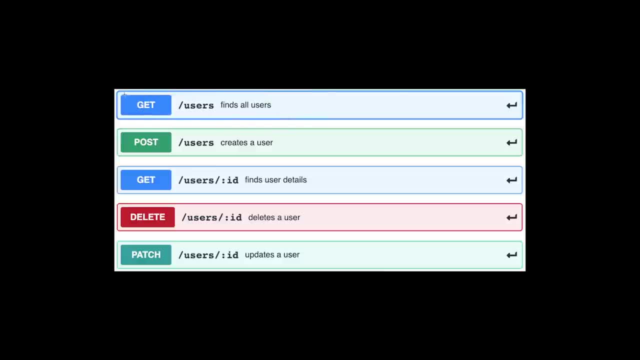 the first one is going to be the get route to the slash users. this is going to find all the users in our mock database. the second thing is a post request to slash users. it is going to create a user. then if we want to find user details for a specific user by id, we're going to make a get. 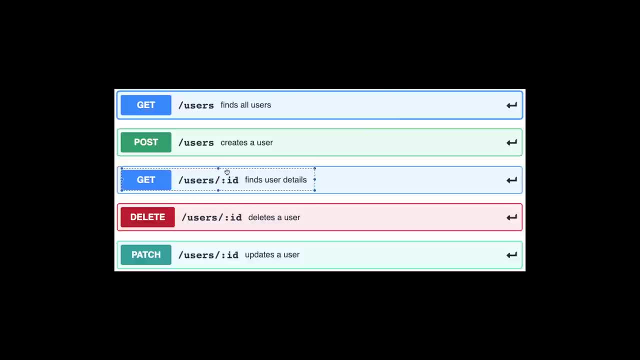 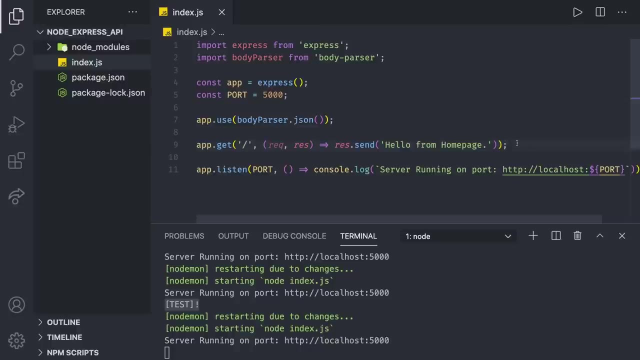 request to slash users and then slash the dynamic parameter of id. we can also delete a user by id or update user details by id. so now let's start with creating the routes. so now let's start creating routes for users. we mentioned that this indexjs file is only going to be for the setup of. 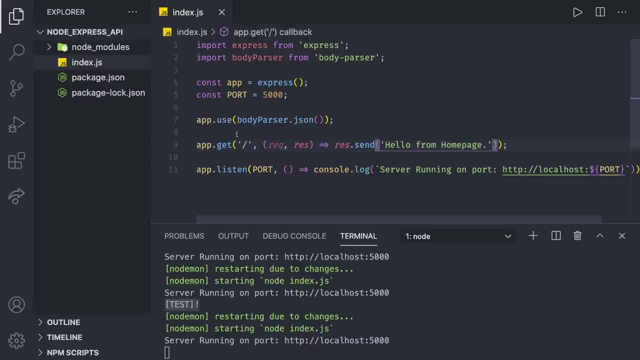 the server. we don't want to add 10 or 20 different complex routes here. so how are we going to do the routing? well, we're going to create a folder called routes and then inside of there we can create the name of the file, and that's going to be something which all of our routes are starting with. in our case, 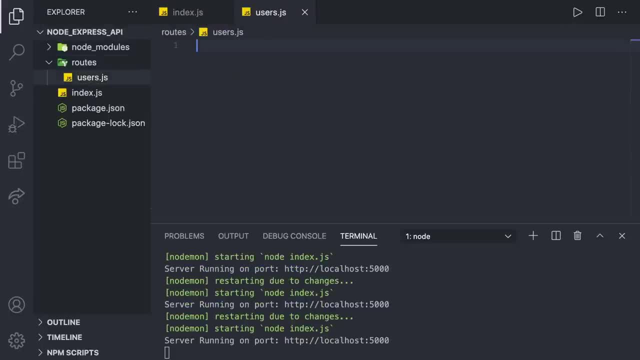 that's going to be usersjs inside of here. we'll also use express from express, so import express from express. so we're going to create a new route and we need to use something called a router coming from express that router. watch out, there is a capital r here on express that router. with this we 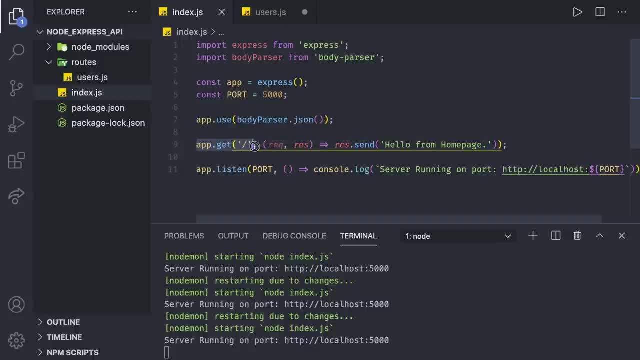 initialized our router in the similar fashion to this thing here: app that gets something in. here we'll use the router that get something, or router that delete, or router that post. you'll see in a moment why are we doing it this way. if we do the route method in the browser, you'll see that i started indicating that ui is uploaded. 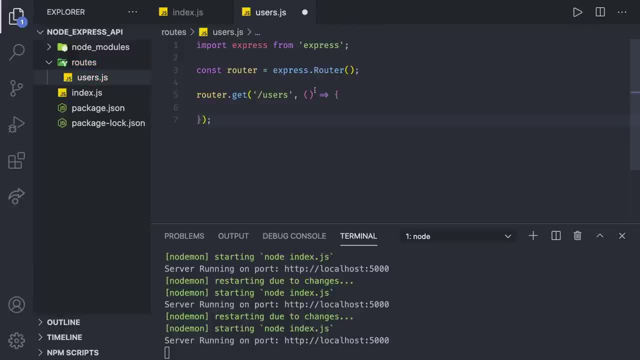 here so that you're adding that. what do you have to do if you have your router along with the backup thing i also have to do is to throw it into id flow, okay, so i want to be sure that this router is actually on the website. 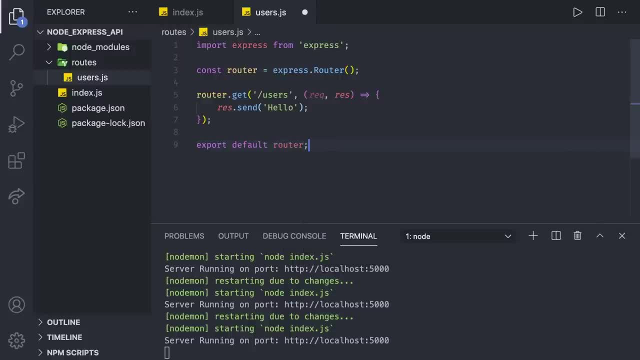 default the router so that we can make use of it in the indexjs file. so export default router once we go to the indexjs file. we can now import that. so let's do that like. import users. routes from dot- slash routes- slash users, dot js. make sure to include this js extension and we named 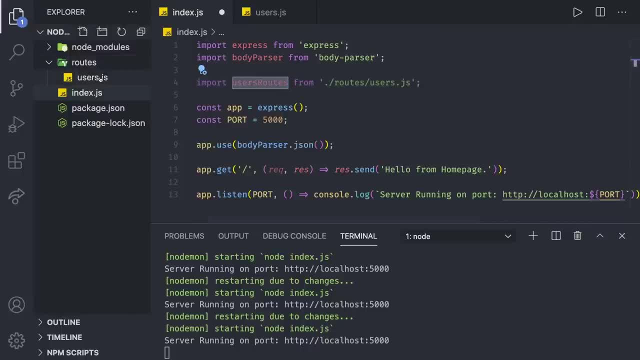 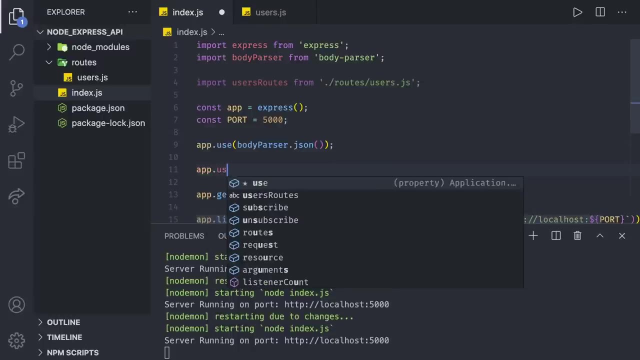 it user routes, because, as you can see, the file is called users. when using default imports, we can name this anything we'd like, but users routes is really descriptive. and then how do we make use of that? well, just below this body parser, we'll say appuse. and in here we set the starting path for 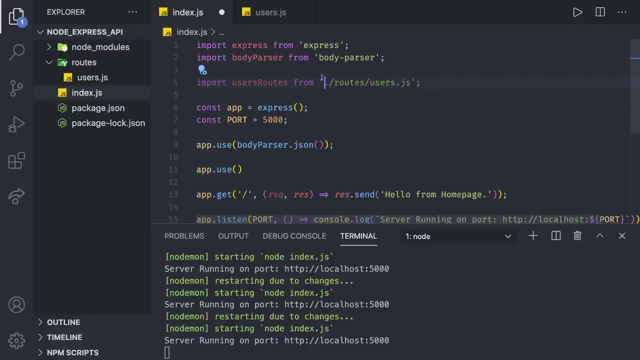 all the routes in the user's file. what do you think that's gonna be? if we go back to this picture, you can see something that's going to be in the user's file. so we're going to go back to this picture and we're going. 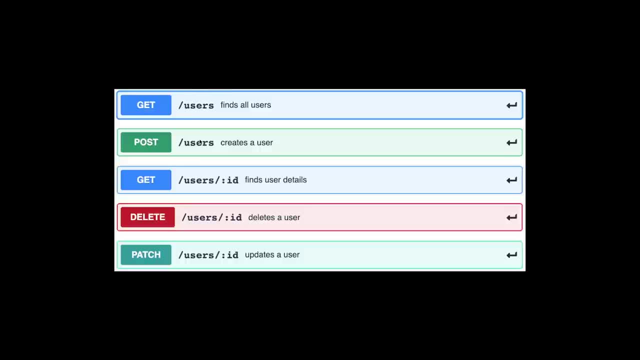 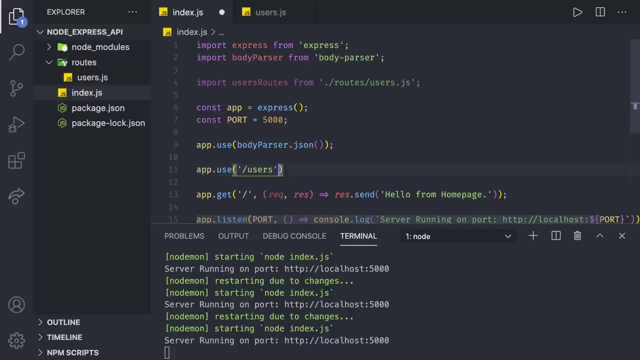 all routes have. they are all starting with users. so in here we are going to specify the path of slash users and what's going to happen when people visit slash users. in here we're going to run these routes. so users routes, the routes we just imported from the users file in the routes folder. so how? 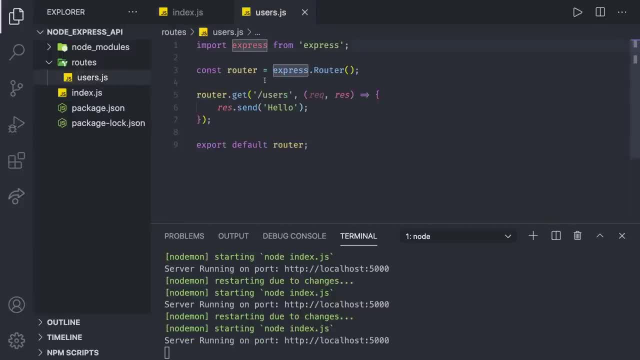 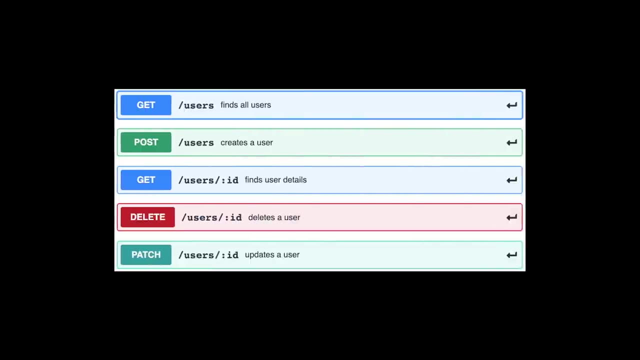 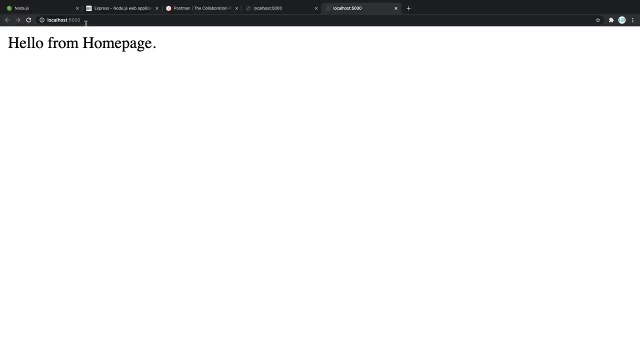 does this work if we now go back to the slash users and let's try to actually reach this? we said we want to get the get request to slash users right here: slash users. if you now go to the browser, you should be able to see that. of course we have the home page. we had that before, but now 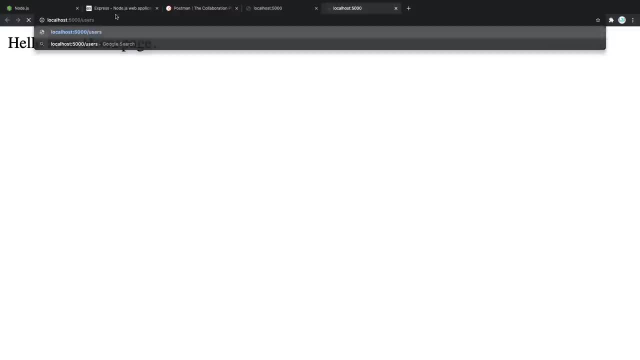 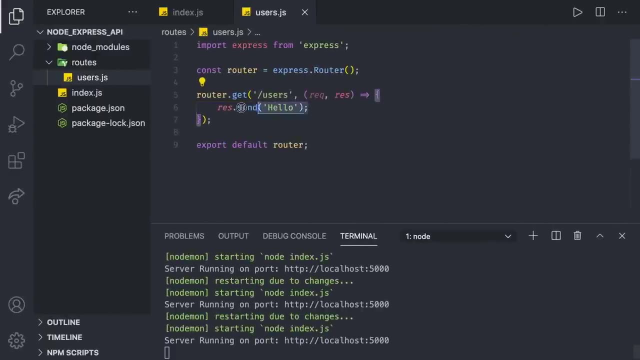 in the url bar if you type slash users, you see, cannot get slash users, which means that our request is not correct. we are not getting the hello. why is that? so? that's because in the indexjs file we specify that all user routes are already going to be starting with users. so in here we're getting. 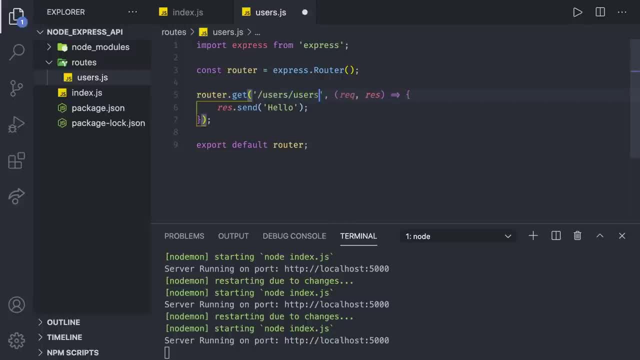 kind of redundant. this is actually pointing to slash users- slash users, which doesn't make any sense. so in here we just need to have the slash. all routes in here are starting with slash users and then whatever we add on to them. in this case, we don't want to add anything, as you can see in. 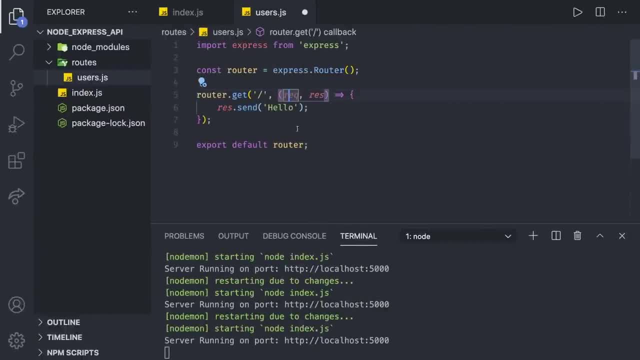 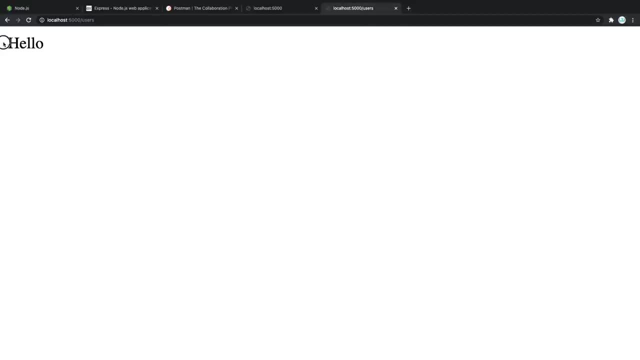 the image here, great. so now, if we do that, we're going to have the user routes in here. we're going to use the underline. so if you do that, if we save it and go back to the browser, we should be able to refresh and see: hello. as you can see, there it is. that means that our route is correctly set up. 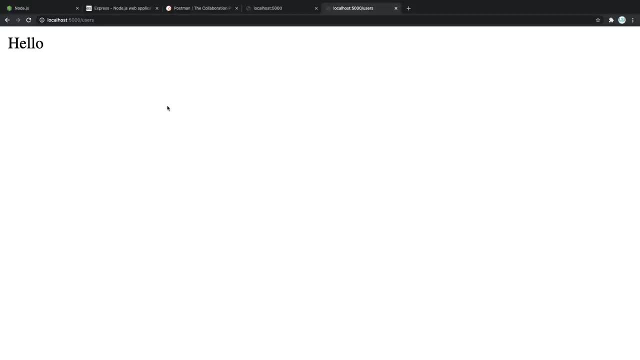 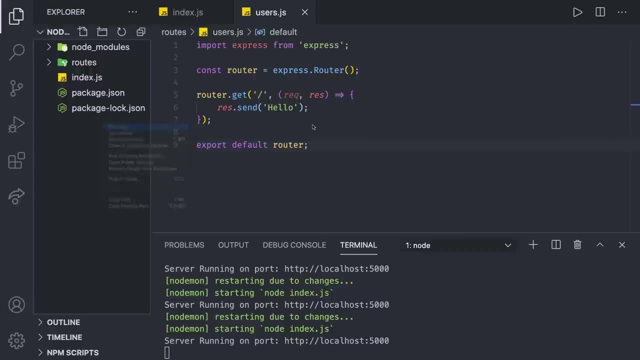 and now we can actually move to the logic of creating different users. let's create a mock representation of our user schema. so in here we can create a new file and we can say user dot json, just for example. in here we can create a representation of how our user schema looks like. 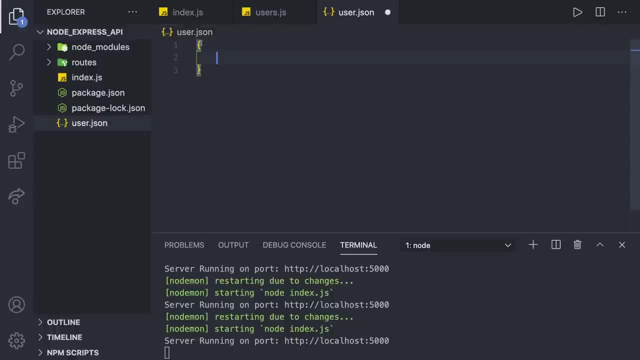 just for example, in here we can create a representation of how our user schema looks like user document should look like. it's going to be a pair of curly braces and then inside- remember, this is json, so we need to use double quotes- we're going to have a user that's going to have. 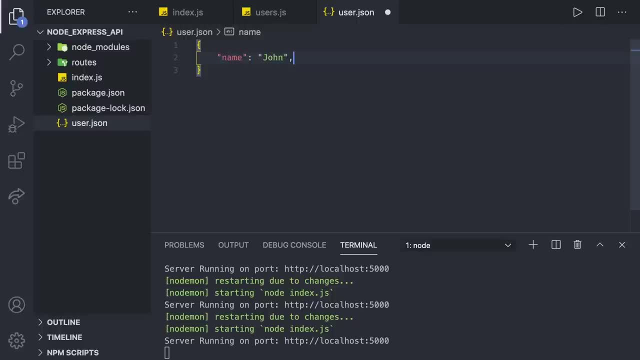 a name. let's do john for the first one and then let's say last name. of course we can then do this to be the first name, last name, john doe. you're gonna see john doe popping often in tutorials. that's just a generic name. and then let's also do age, for example. let's do 25, as you can see. 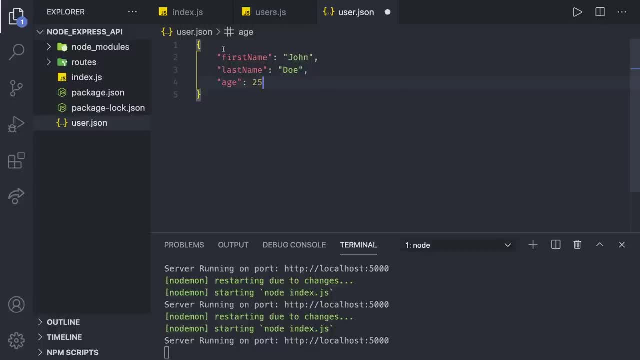 it's really similar to normal javascript objects, but there is only one thing: that you need to have double quotes. you also cannot have so-called trailing commas. you need to do it like this. okay, so now we know how our person object is going to look like. let's try to create our mock. 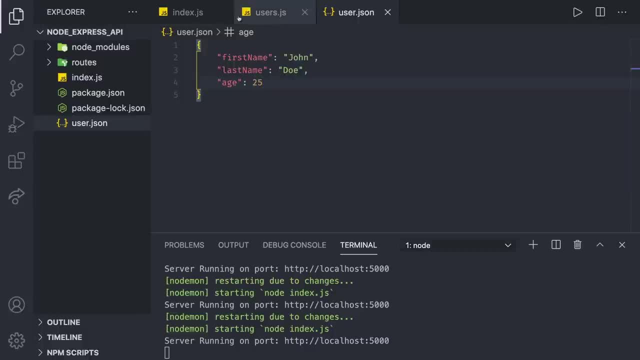 database containing two different users. inside of the user's route, i'm going to create just a normal array, so just array, and we're going to call it users. const users is going to be equal to an array and then inside of there i'm going to copy our 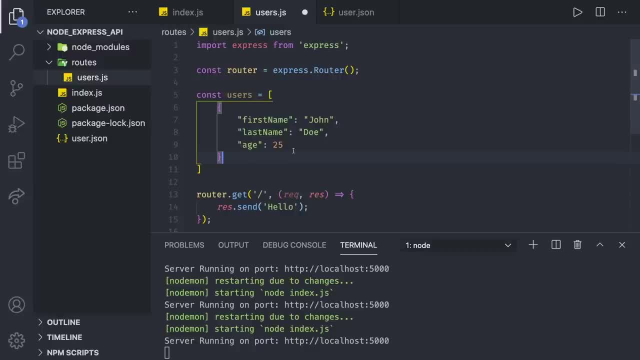 john person and just paste them inside of here. now our users array has one object with the first name of john, last name of doe and the age of 25. great, since this is not json, we can also remove the string signs on the keys of objects- great. so now, if we do that and save the file, let's try to console log. 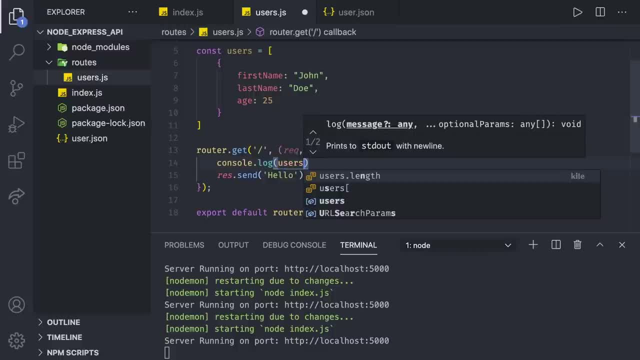 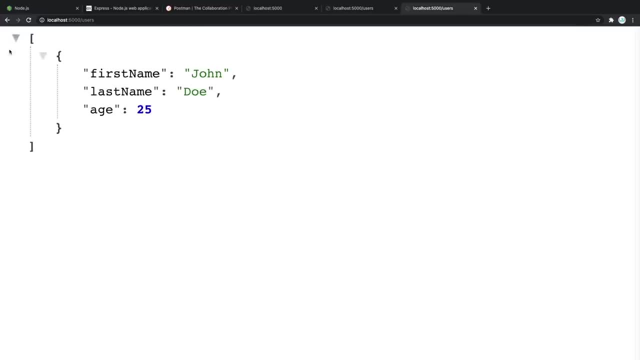 our john right here. so console log users and let's console log all the users, although we currently have one. okay, when we go to slash users, we get some json data, as you can see, we can collapse it or uncollapse it. maybe this looks just like a plain text for you, just a plain empty black string. 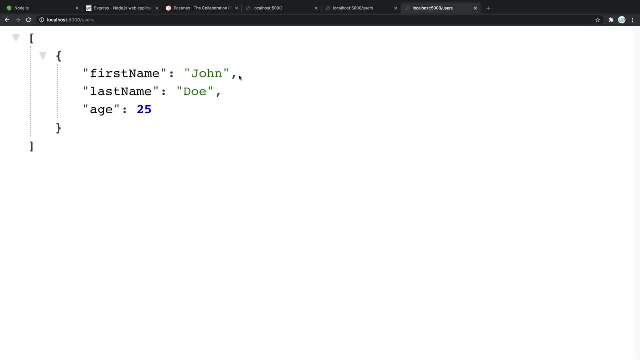 if that's the case, go to your chrome store with the extensions or any other browser store and download something called json formatter. as you can see here, with json formatter i can see the text raw or parsed. so if i click raw, this is how our json file looks like, but of course it's much nicer having it parsed. so feel free to download that. 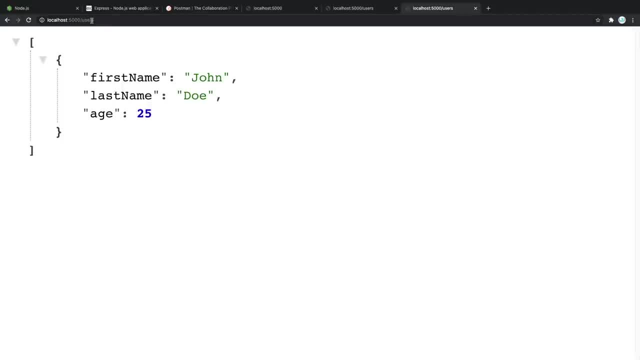 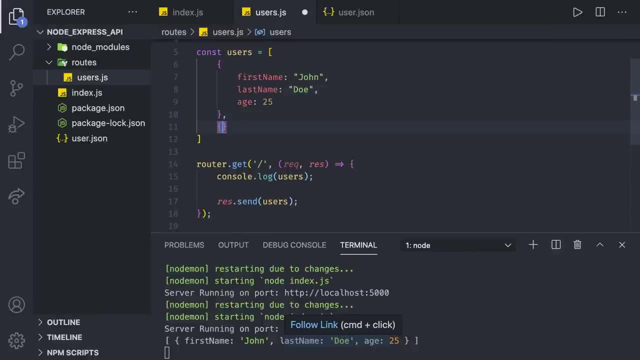 and that's it. as you can see, we already have our get route for all the users. let's add one more, just so we can have two. for example, let's do first name, that's gonna be um jane, and then we can do the last name also, though, and the age is. 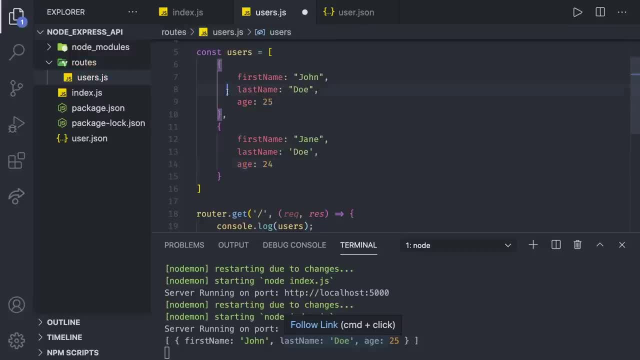 gonna be, for example, 24, just like that. if we save it, go back to our browser and also, as you can see, here, we also got our users in the console log once we visited that route. if we go back, save it, we now do get two users. that's great, and in here we have our. 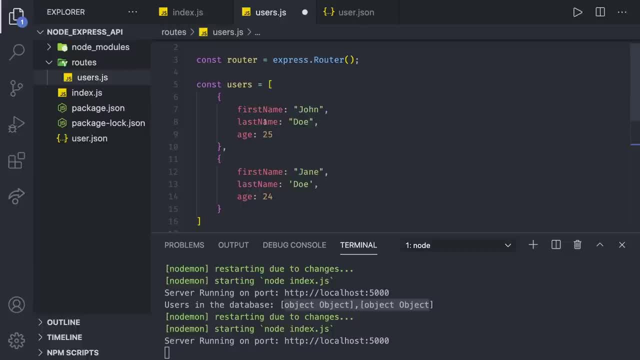 users. now we need to add the functionality of adding users to our database. we're going to go below this routerget and we are going to create a new route. this time it's going to be routerpost. it can no longer be a get route or get request, because we need to send some data from the front. 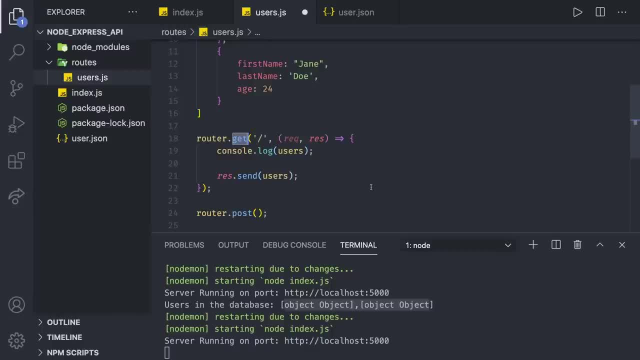 end to the server, that data being the values in the forms user inputted. for example, whenever you see a sign up or login form there, you have username, first name, age. these are data values that we need to send from the client to the server for the user to be created, so that's why we are using a routerpost method. 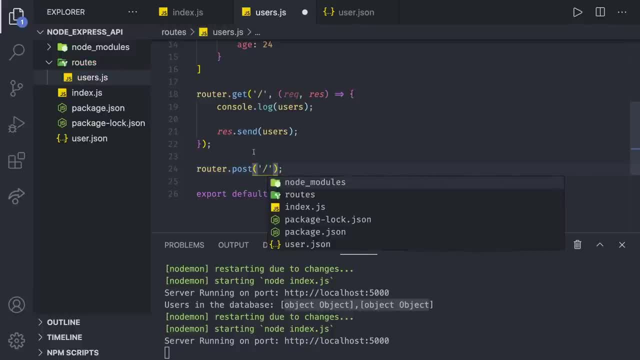 in here. the path is going to be again: just slash users. we're just saying slash and then we have the request and response callback function in here. now we'll have to deal with some actual data we'll be sending in for testing the post route. we can no longer use chrome or any browser for that matter. why is that? 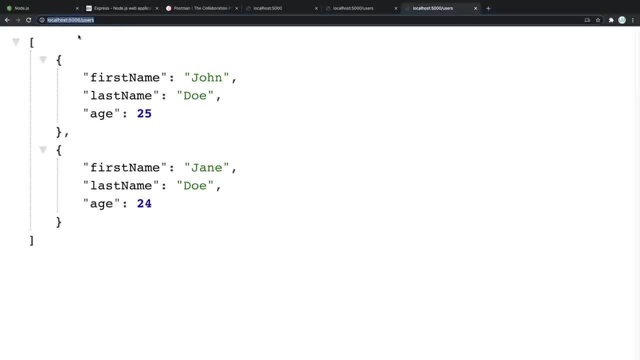 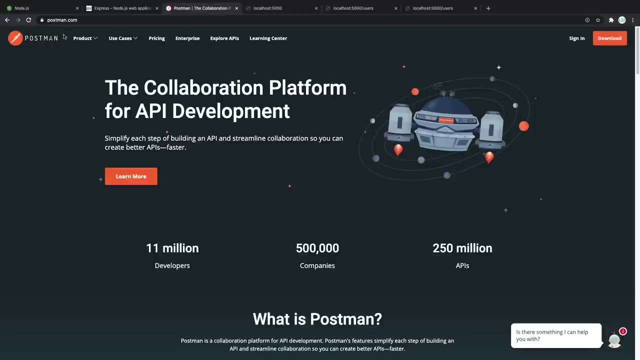 so because whenever you type something into the url bar, it's making only a get request, so browsers can only make get requests. that's why we need a software which can help us test our api, and that's where postman comes in handy. you can just go to the postmancom and then to the download page in. here. you can just click download, install it your device and now you can get your app. that will be running. grab your device and then just click the download button. click download, go to your device and you're ready to go. download- upload your app to your device. just click download, upload and then you. 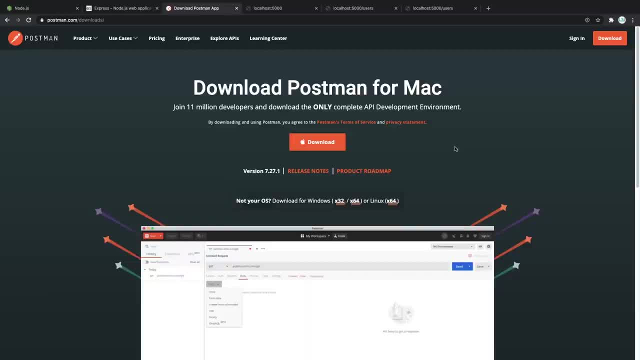 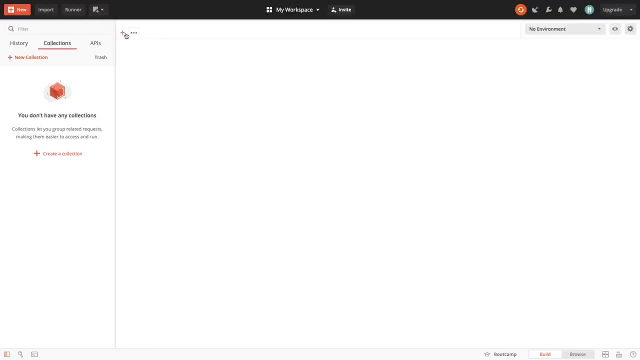 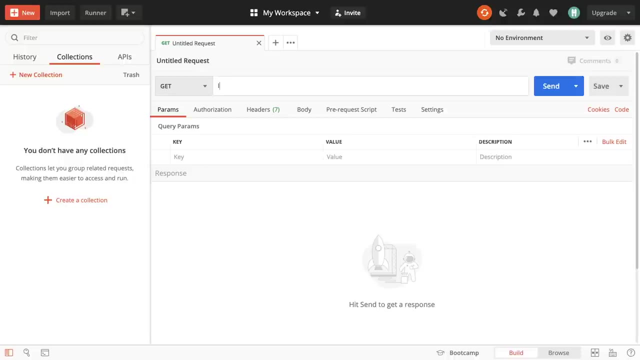 then open it. Once you do, you should be having something like this. So how can we make different requests with that? Well, we go to this plus icon on the top, And in here you can see that we have something similar to the browser's URL bar. In here we can say localhost and then 5000. And 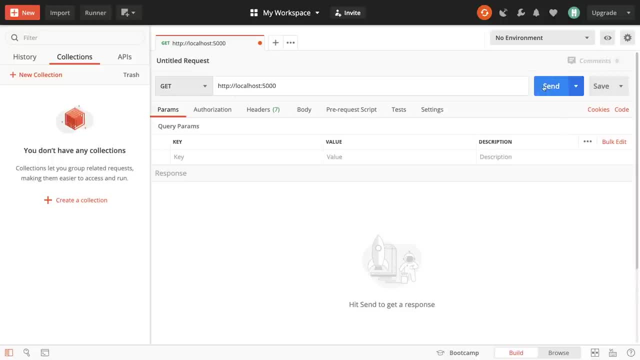 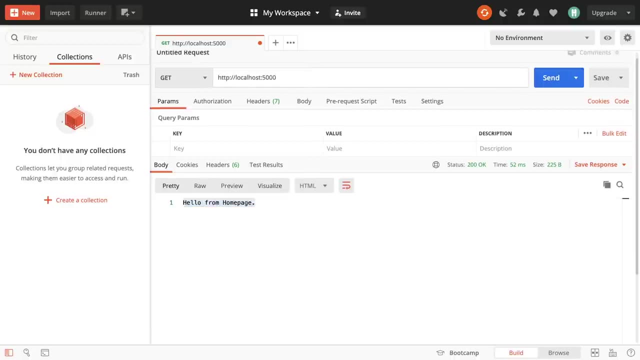 right now. let's try making a get request to localhost 5000 to see if we get anything. And we do get, we get hello from homepage. Let's now do localhost 5000 slash users. we know that that's going to give us some JSON data, as you can see here in a nicely formatted way, even with some. 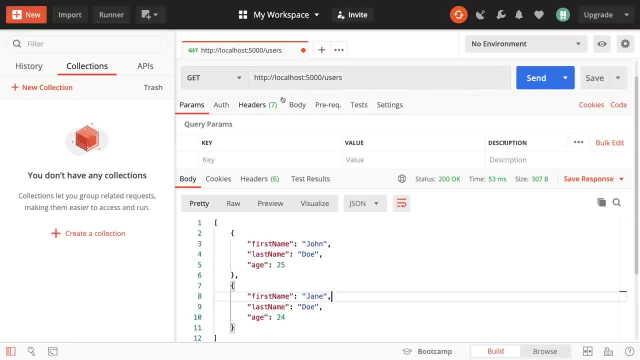 line numbers. And now what we can do here, but what we cannot do in Chrome- is we can change the type of the request, So in here we can make a post request to the same or different route. So how do we send some data in? Well, you need to move. 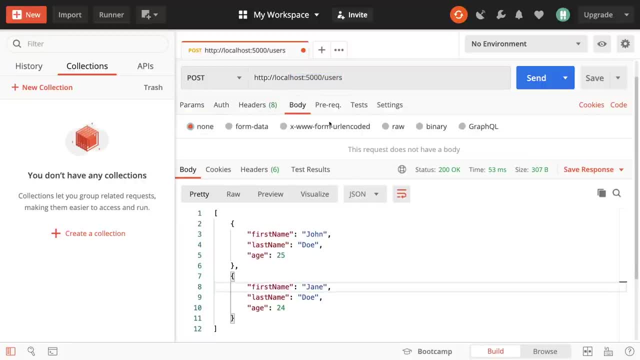 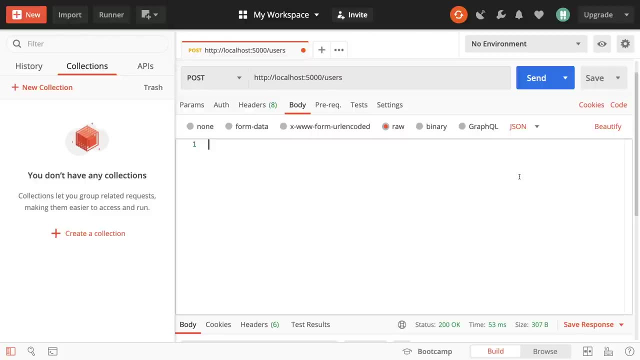 here from params to the body tab, then need to go to the raw and then change the text to JSON, So we'll be sending data in the JSON format. So what data do we want to send to the database? Well, we want to create a user, of course. So we are going to create something similar we created in the mock. 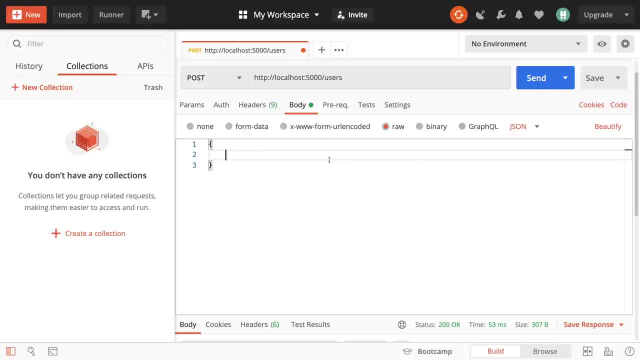 user JSON file In here. of course, the user needs to have a first name. keep in mind that this needs to be wrapped in double quotes- And then we're going to create a new user. So we're going to create a new file in our place the name, and let's say Johnny this time. then we have the last. 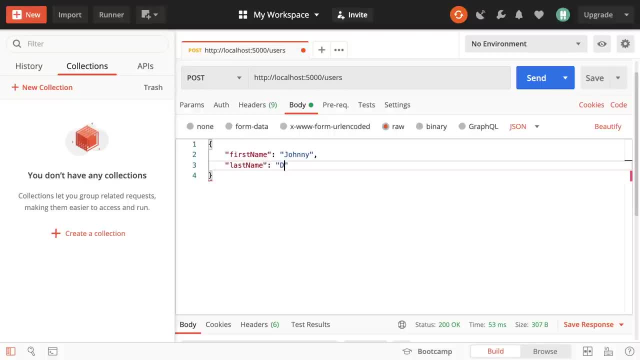 name that can be a son. So let's do, though, one more time, And then let's do the age of 10.. That's it. So if we do this, we are sending some data to our host route. How can we see that If we go back? 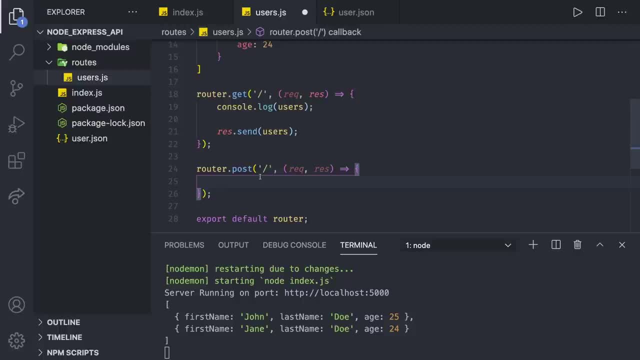 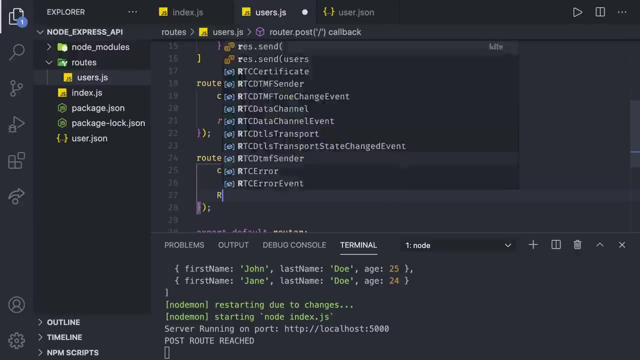 to our Visual Studio code in here. let's do a simple console dot log and we'll say route reached, or let's add post route reached, so that we can know if this callback function was fired. along with the console log, let's also add the rest that 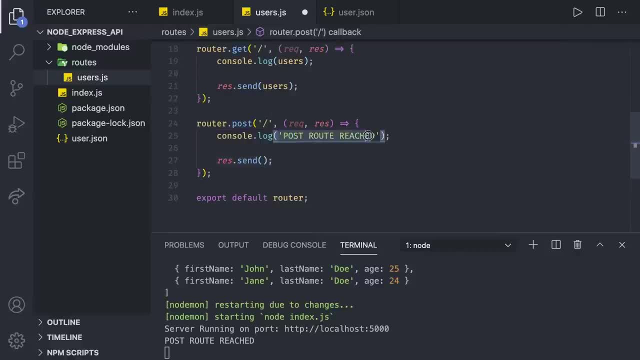 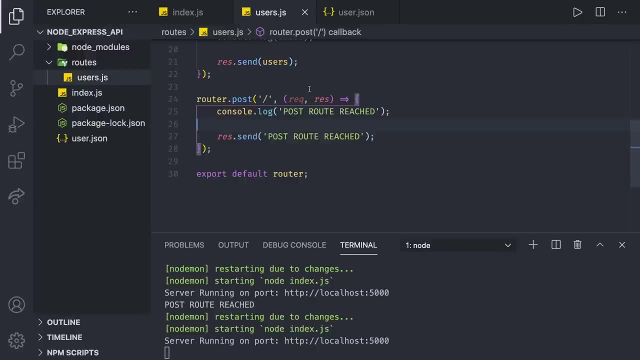 send. that's something that's gonna be sent back to the client side and we can say the same thing post route reached just for now. so if you save the file and then go back to postman, you should be able to click the send button and, as you. 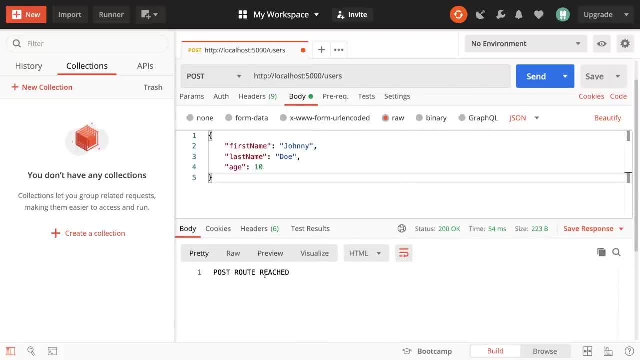 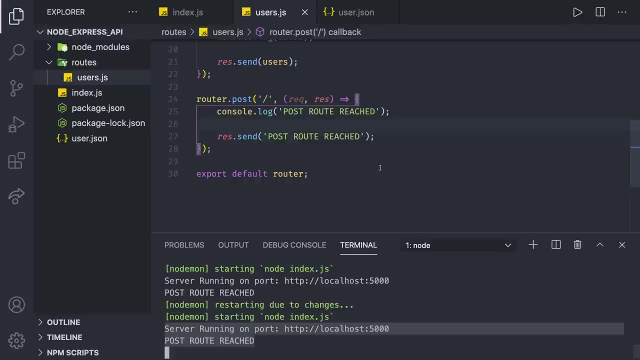 can see. the response is going to pop up right there. it says post route reached and also in here in the terminal you can see post route reached. great, so how can we actually add the user to our database? well, in this case we are using a mock database, which is just a single array with some objects. it's not going to be. 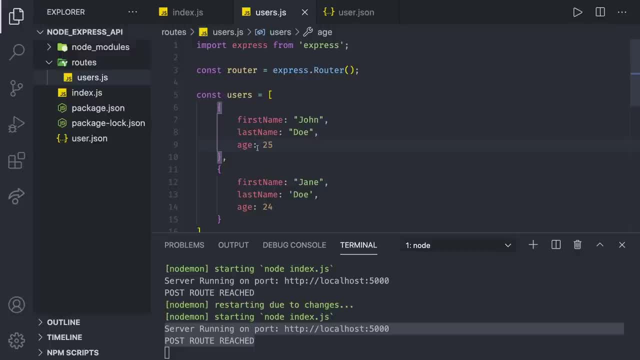 stored once we add the user. every time we call a new server or we refresh a server, it's gonna be changed and go back to the previous one and then we're going to add a new server and we're going to just two users. so if you want me to create a new video where we are going to 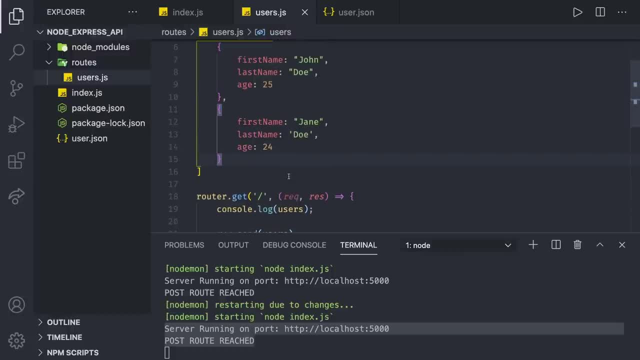 interact with real database, MongoDB in this case. just let me know, and that's going to be the topic of the next video, but for now, let's keep working with the mock database. of course, the point of this video is to learn Express and node. so just think about it. how would you add a value to the array? just a push method. 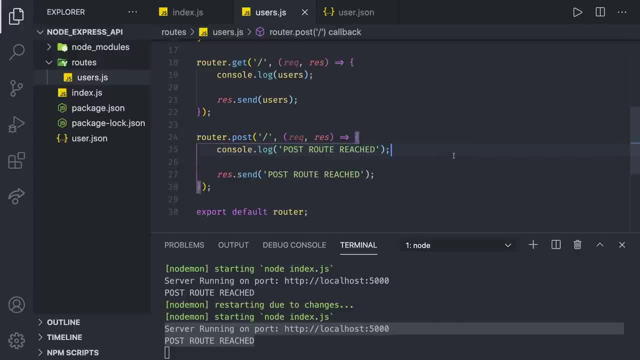 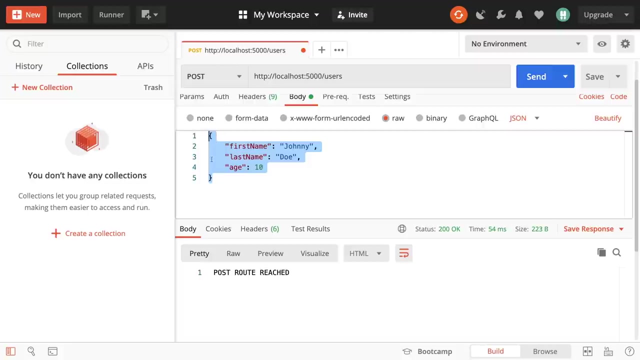 right. so let's do exactly that in here. we're going to call the users and then do the push method. what do we want to push? that's the great question. we want to push what we send from here. this is the user. so how do we get to that data when we are working with both requests? 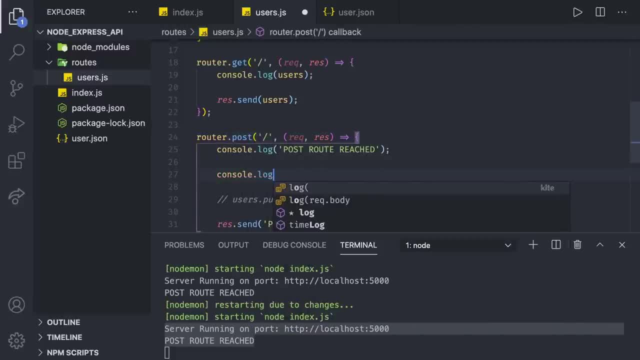 we have something known as a request dot body. so let's console log the full request that body so we can see what's hidden inside of it. if we save the file one more time, and we're done we, when we get to the end of the session, let's just 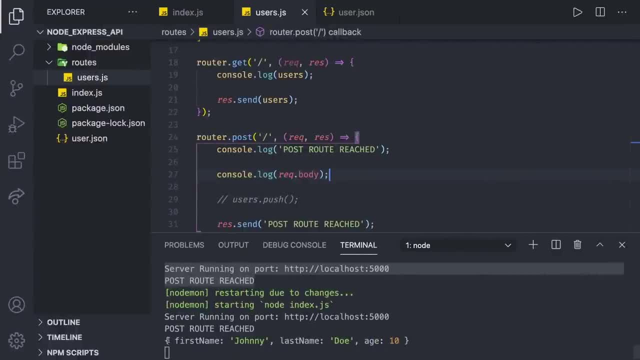 and restart this request. now you can see we do get the full object right here. it's being stored in the requestbody. now we can put that into a constant, so let's do. const. user is equal to recbody and now that we have the user, the easy thing to do is to just push that user to our 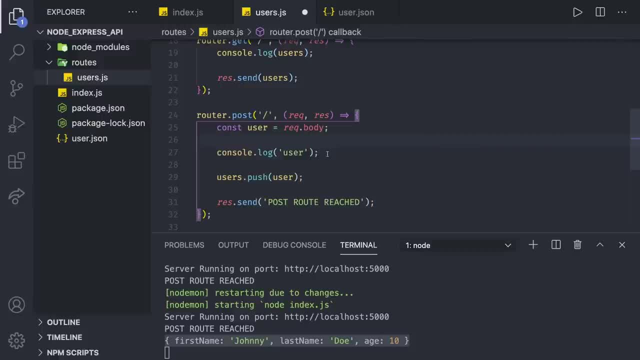 current users array. the other thing that we can do is we can provide a useful message to the client side once they make the request. so let's remove these console logs and this one as well, and let's just send something useful. we'll send a template string which is going to say um user. 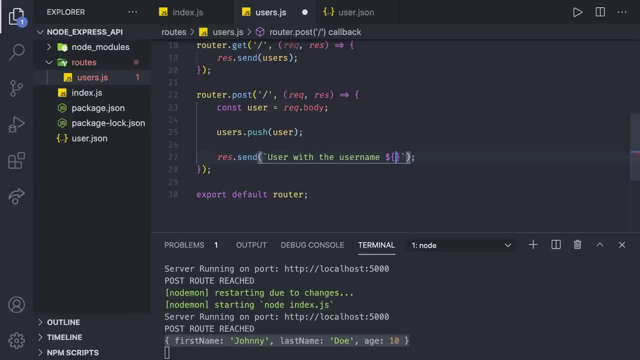 with the username and then in here we can use template strings: user: that first name. sorry, it's not going to be username. it's going to be the first name user firstAA and it's not going to be all the one. that's going to be the. 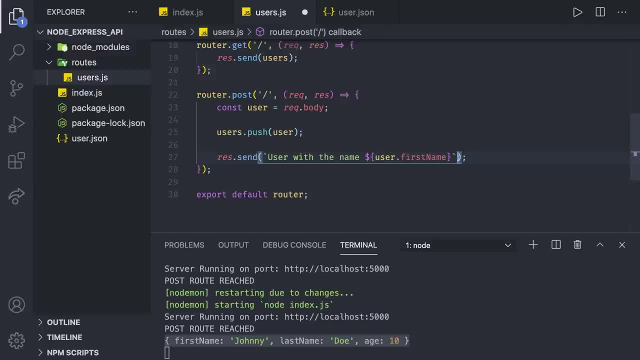 username. you're might want to Hang on because you are going to need the template, because the next thing that we're going to need it is the user, and then I'm going to pull this end up to the end be: user with the name, something added to the database. That's it. So now, if we save this, 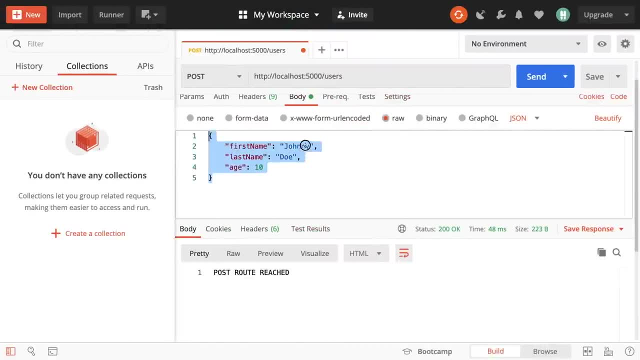 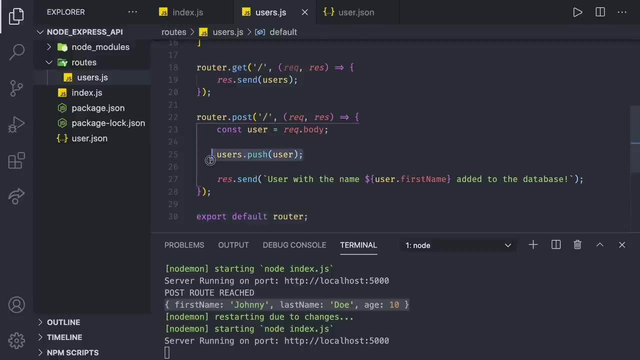 if we go back one more time and let's try adding Johnny again, save it user with the name Johnny added to the database. That way we can be sure we added Johnny, Great. So now, why is this special? What did we do? We just push the user, but can we somehow see the action of our doing? Well? 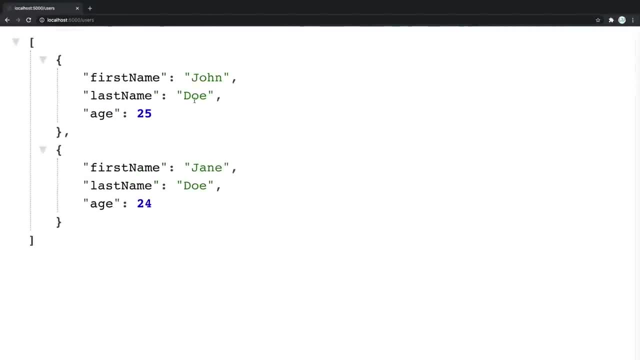 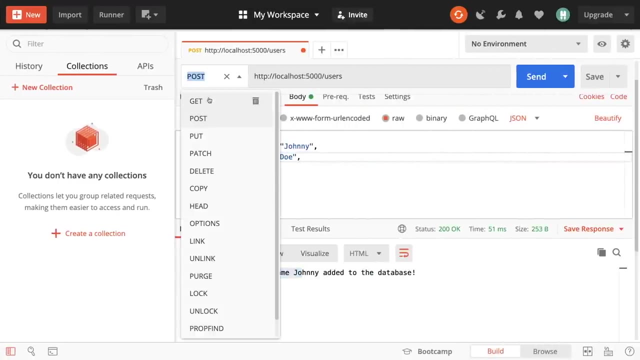 if we go back to our browser right here and now, refresh the page or rather make a get request to the localhost 5000 slash users, you should be able to see that now we do have three users. We can also check that out if we make the get request to the same route using postman right here. 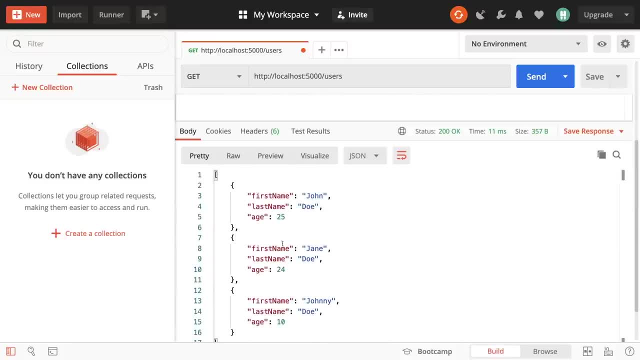 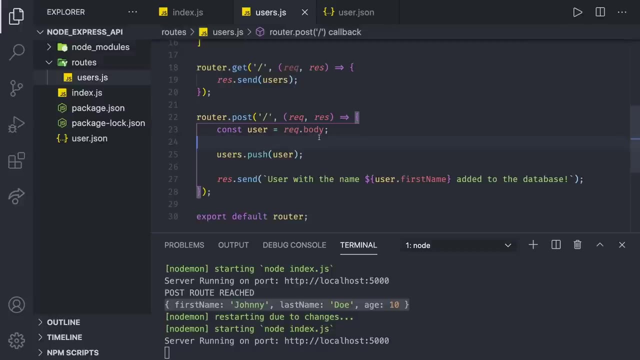 Send And, as you can see, we do get three values. That's amazing. You just created the get route to get all the users, And we also create the post route so that we can add users to our database- Amazing. The thing that we need to do next is we need to be able to get the details of only one. 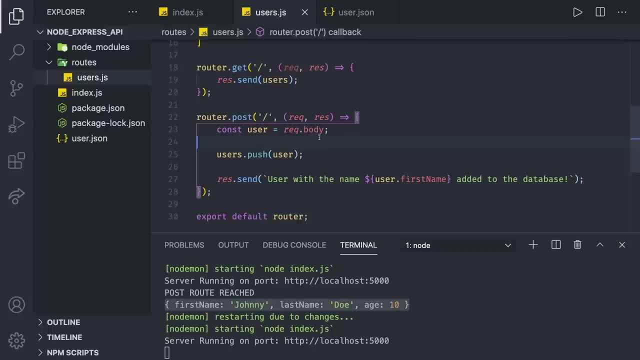 single user. For example, if we are logged in as John, we need to get back the details about John's profile. So for that we need some kind of an ID, some kind of difference From which we can differentiate all the users. Right now, of course, the name John only shows up. 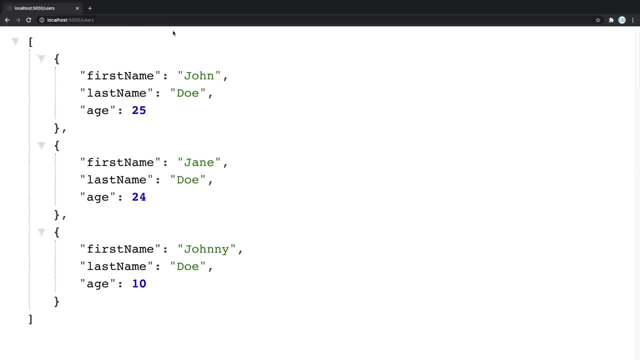 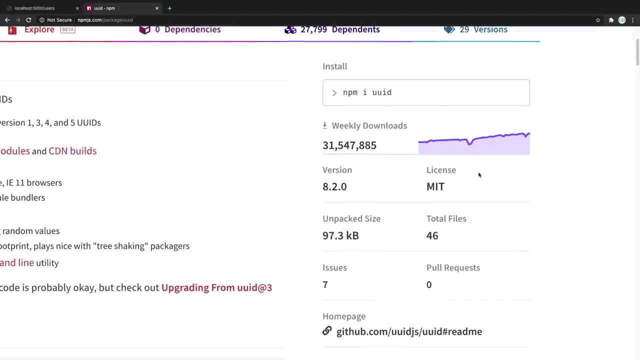 so we could search by that, But of course there are going to be many other people named John in our big application, So for that it's good to use some kind of unique ID. There is a package on MPM called UUID And, as you can see, it has 31 million weekly downloads, which means that it is a really 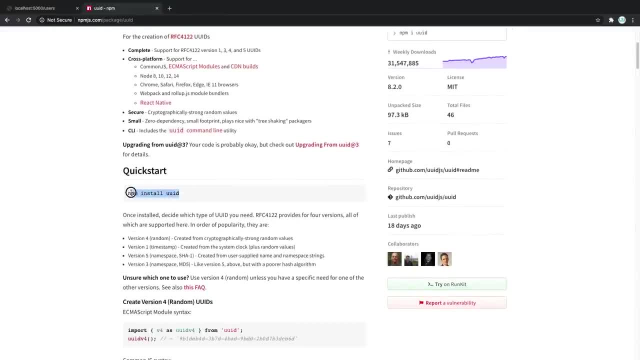 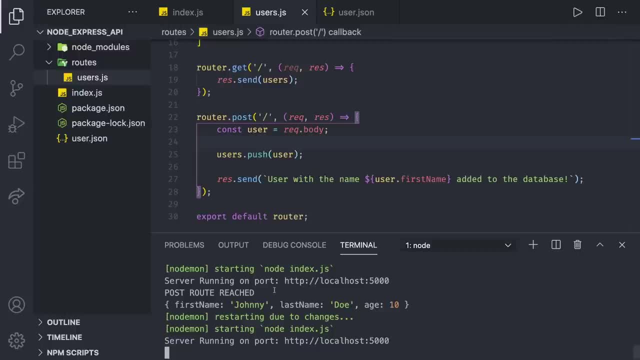 popular package. So what does it do? We can install it, of course, by just typing: MPM, install UUID. Let's do that right away. To close this terminal, you need to press control C to close it, And then we can run this command. 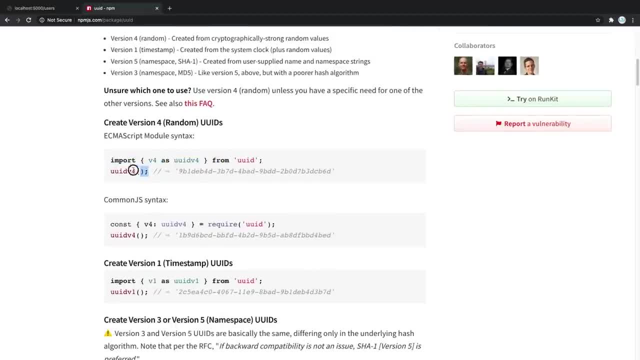 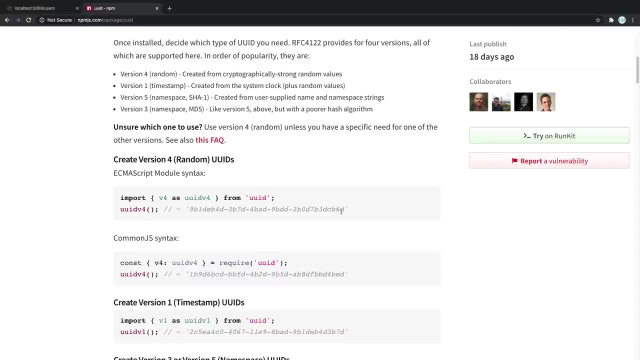 In here you can see that we just imported and we just call it as a function. Once we do call it, it gives us this huge string with unique numbers. This string is never going to be the same as any other string created. It uses different timestamp. 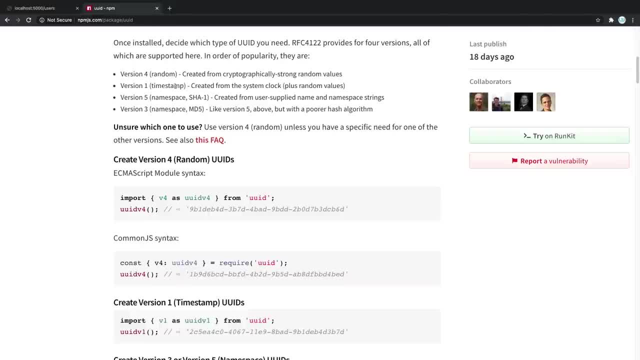 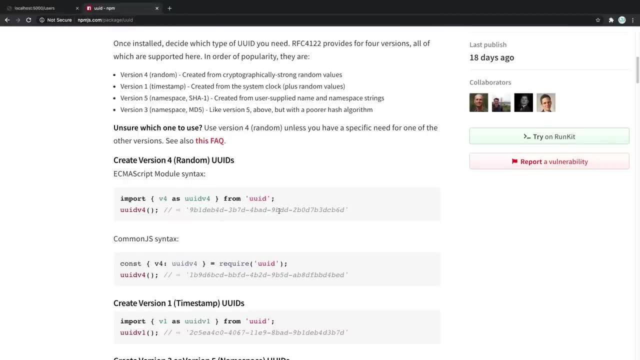 It uses different timestamps, namespaces, random cryptography and a lot of different things to make sure that this is never going to occur again. That way, we can guarantee that no two users in the database are going to have the same ID. Great, Now that we installed it, we can copy this. 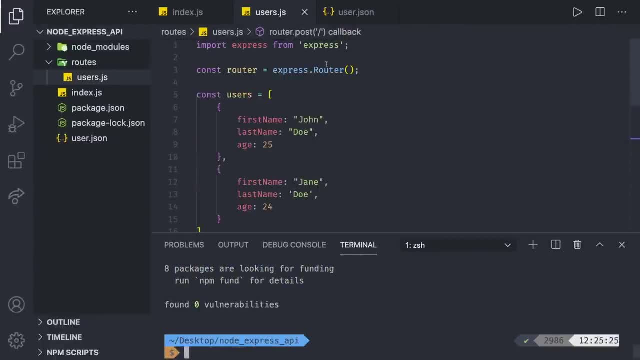 go back to our application. and now go back to the top Import version 4 as UUID version 4.. And, as you can see, we can. And now go back to the top import version 4 as UUID version 4.. And, as you can see, we can just copy and paste the. 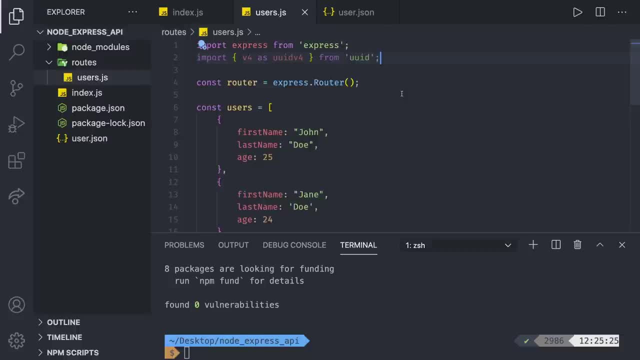 And now go back to the top import version 4 as UUID version 4.. And, as you can see, we can just copy and paste the. just call it like this. so let's copy that. and now the question is: where do we actually want to add? 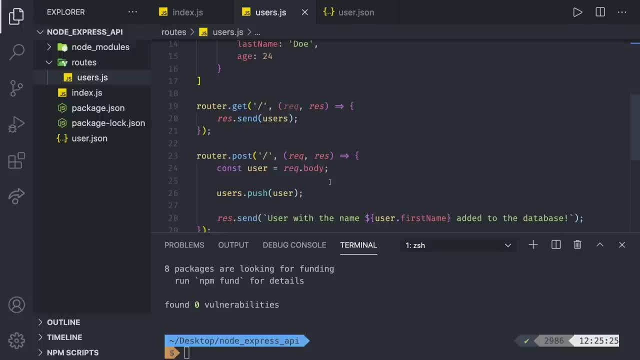 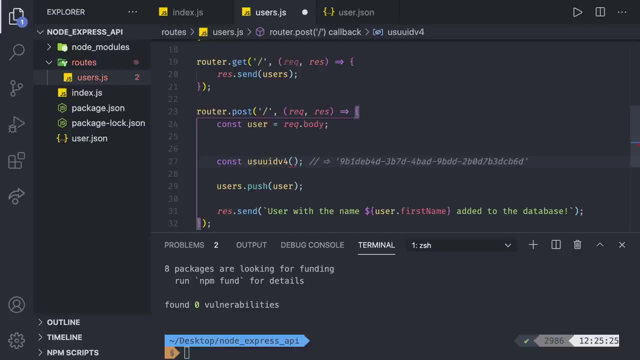 that id. well, of course, when creating the user. so we need to use that right here, and this thing actually is the user id. and now the question is how we can add this to the current user we are getting from the recbody. well, we can create a new object- let's call it user- with id, and then 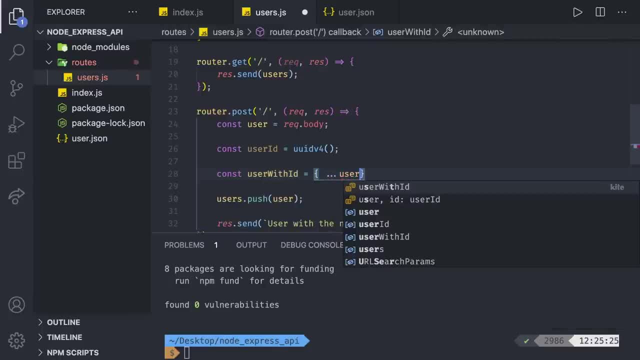 in there. we need to spread all the properties from our current user and also add the property of id equal to user id. this may be a bit complex depending on how well do you know the spread operator and creation of objects, but, as you can see, we just created a new. 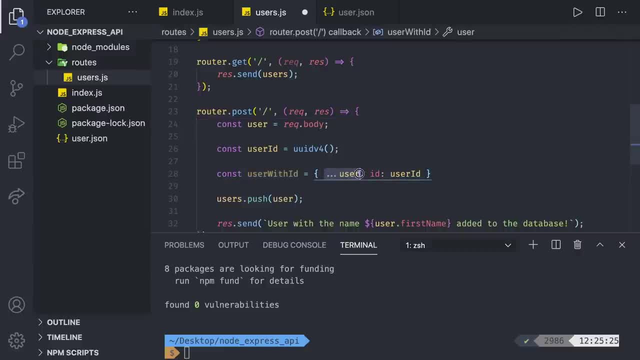 object and we're going to create a new object. and we're going to create a new object and we're object, which now represents the user, and then we spread all the properties of the user, meaning the name, the age, and then we just added one more value on top of it, and now, instead of returning user or 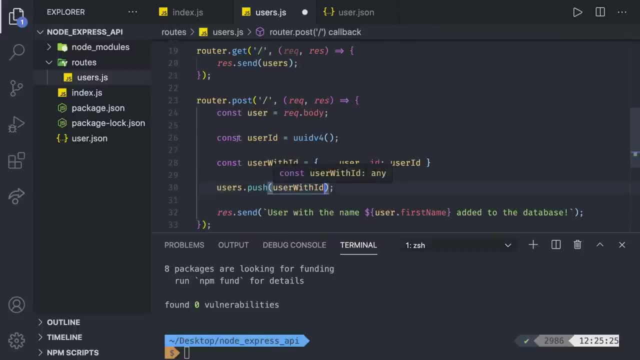 pushing user. we can now push user with id. of course, we can even simplify that. as you can see, user id is a variable only mentioned once, so we can just take the value and paste it here, immediately getting rid of this. and, as you can see, user with id is also mentioned only once, so we can just take 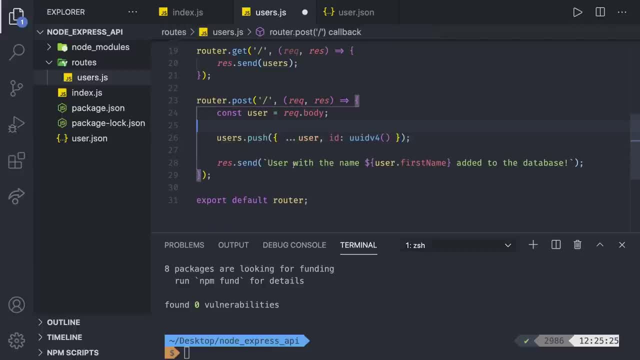 the value and immediately have it right here. this way we have almost the same thing as before: having the user, but this time we are also adding the id to it- great. so can we somehow see this in action or not? well, of course we can. if we save this and now run npm, start again considering we. 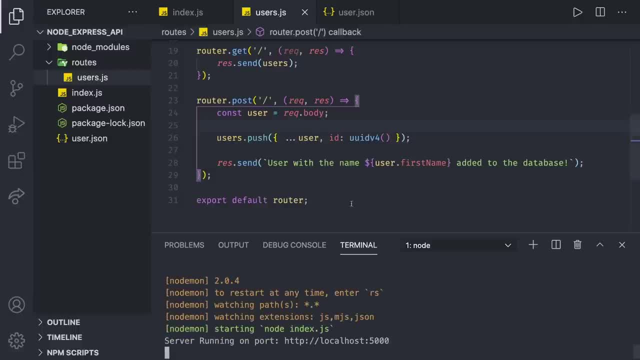 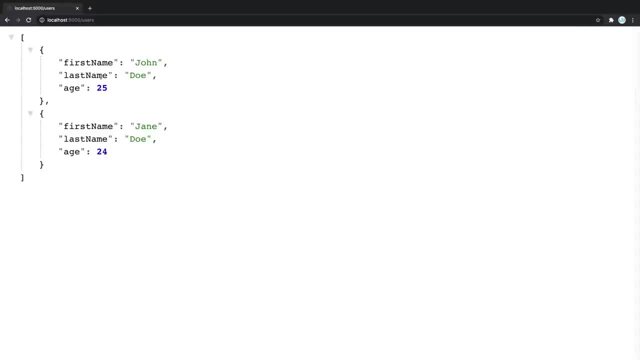 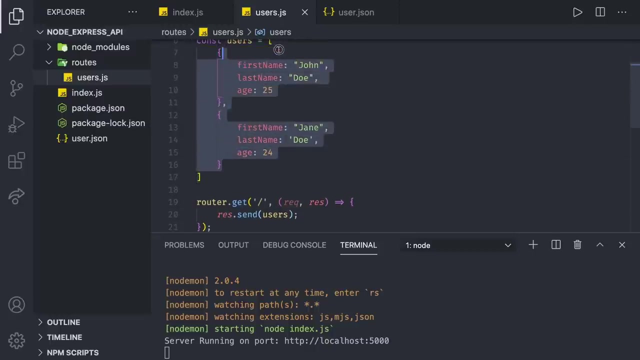 close in our server. as you can see server running. we go back to our localhost 5000 and now refresh the page. these two users do not have an id and that's because we created them. we just created a mock database here. we don't want to have any users here. let's let's just leave it empty for, for starting right, the 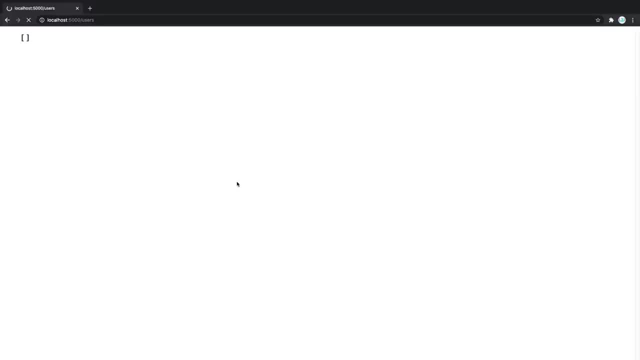 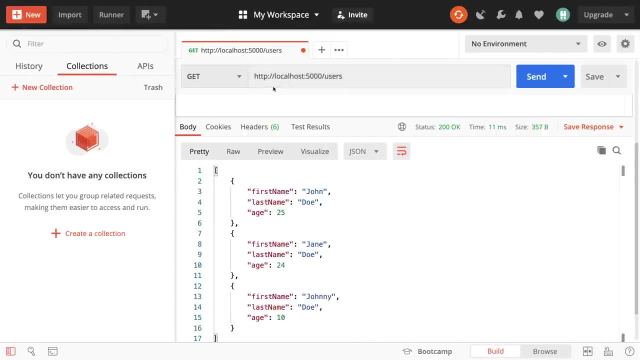 database is empty at the start and then if we go back and refresh now we have no users. good, but now how can we push new users? we already tested that out. so if we go here to the post request and we try adding one user, let's always keep adding the john. 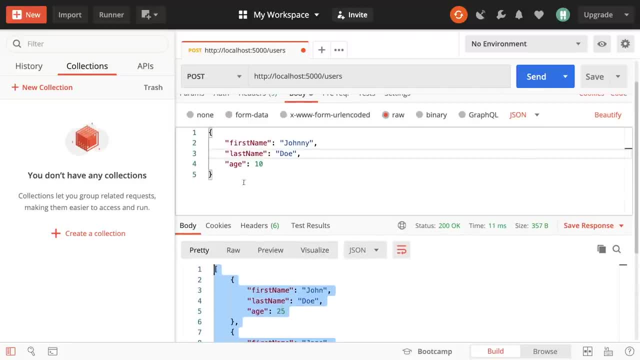 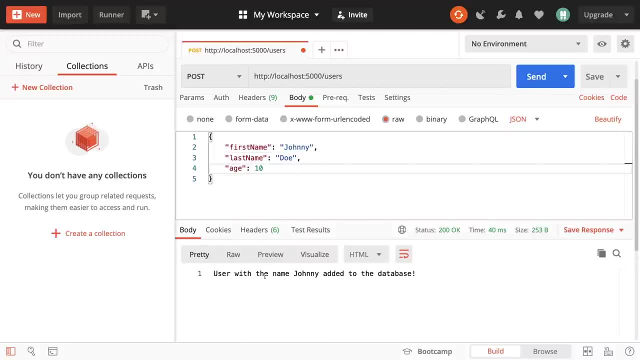 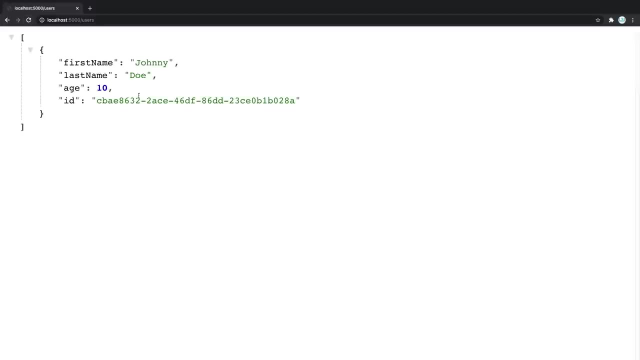 so i'll delete this and i'll just push the. oh, we already have it here, so we'll just push johnny, for example in here, click send okay. user with the name johnny added to the database. and now, if we go back to the browser, refresh. you see we do have johnny doe with the id of some random gibberish. 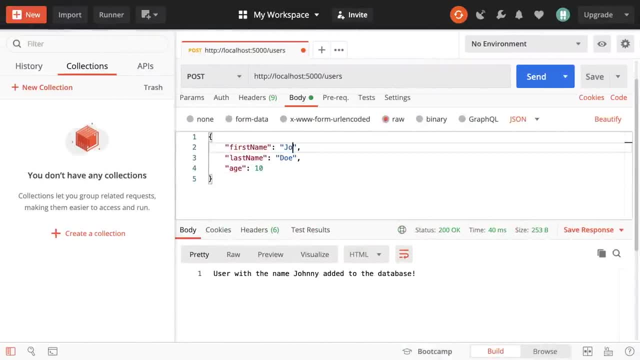 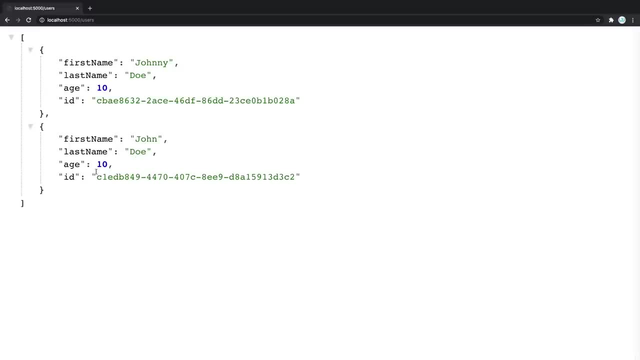 numbers: great, let's try to add one more, for example john doe. save it. and, as you can see if you refresh, now we have john doe as well, but this is completely different: c, c, b, here we have cl and of course everything else is different. you can see for the ending letters: great, now we know that each 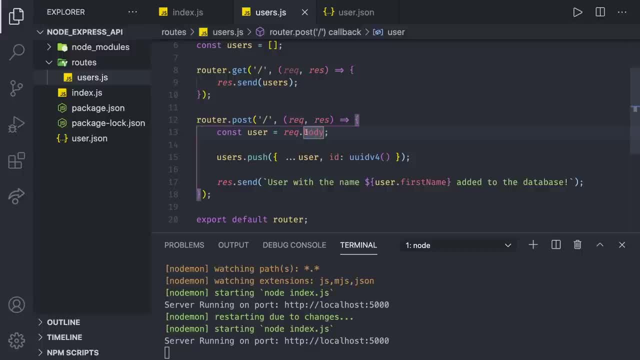 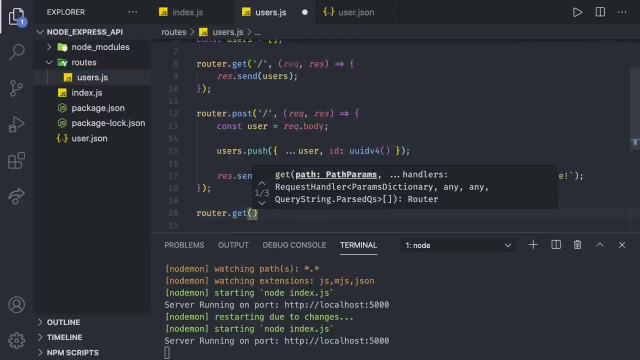 user is different. in a way, we have something that we can differentiate it by, so now we can create a new route: routerdoe get. this one is also going to be get, but this time the path is going to be to slash users and then slash id. in a moment i'm going to show you why i put this colon sign right there, but for now let's. 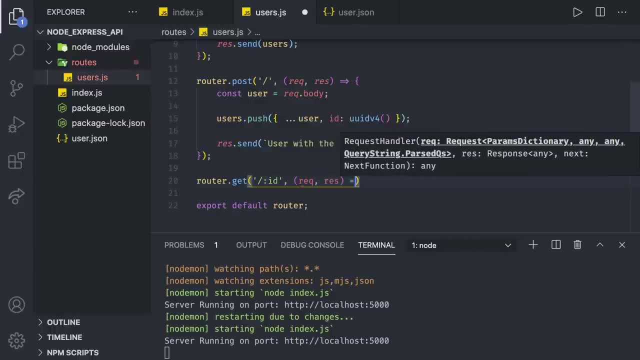 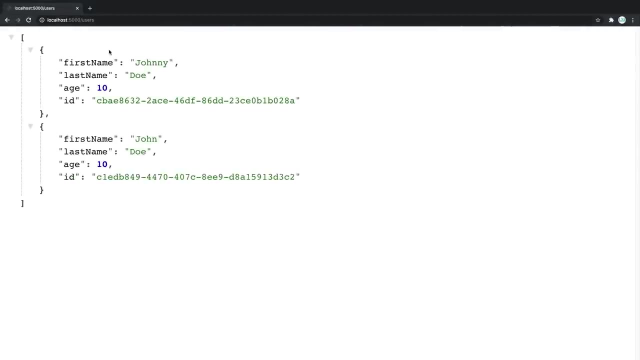 just test it out. let's create rec res, as we always do- you can see the pattern now- and let's just return ressend the get id route, just like that. now you can either test it with browser or the postman, because you know that when we have a get request, 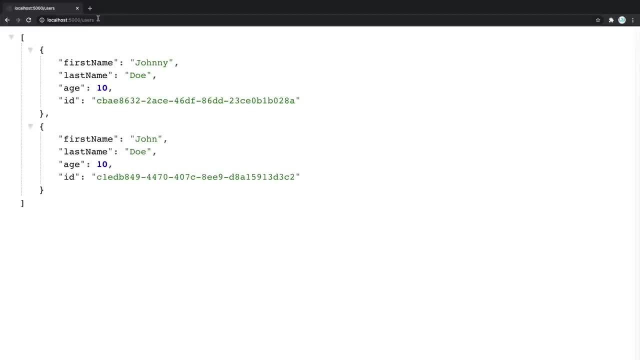 you can make the get request from the browser as well. so if we now go to slash users and then slash id, as we specified, right, we should be able to get the the get id route, and we do. that's great. so what if we do something like slash users, slash test? oh, that also works. 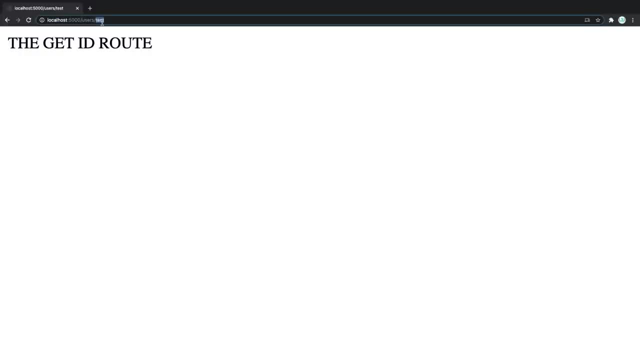 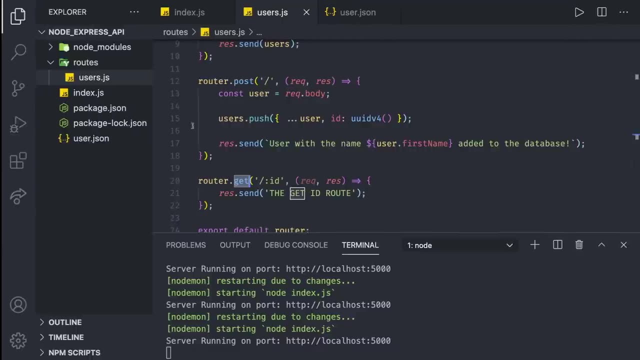 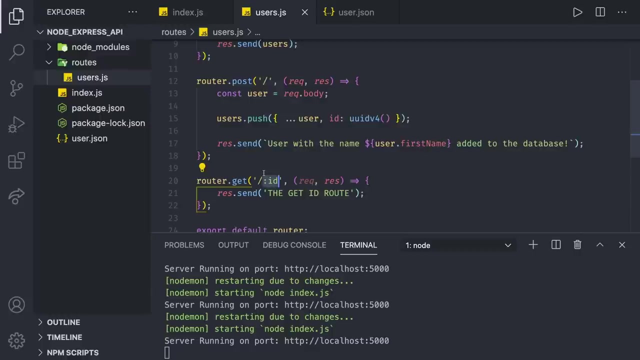 what if we do something like slash users and then put the id of some random numbers and then do that? that also works. that's because when you put the colon sign here, you're expecting anything after the user's path, so we can put anything and this route is gonna hit. so can we somehow get this id? 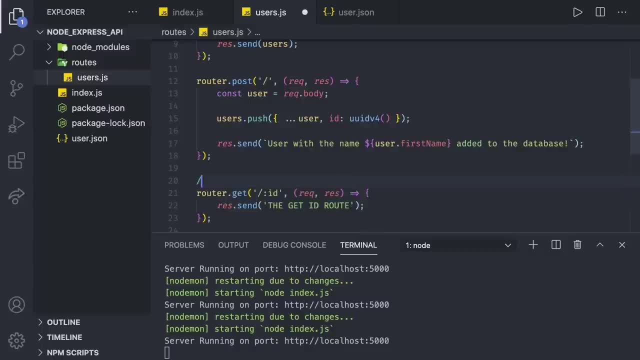 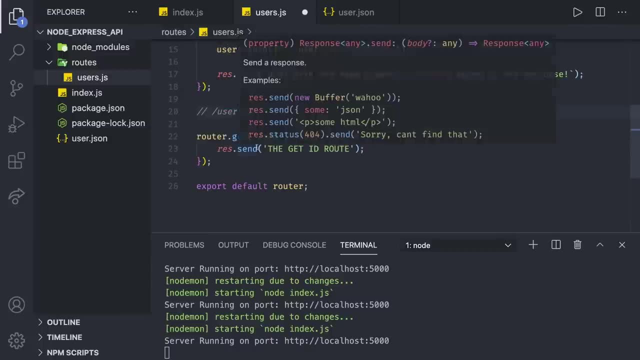 which the user sends, for example, if he does the route to the slash users and then slash two, two being the id. can we somehow retrieve the value of two in this callback function? we can. it's stored in the request that params, params being the parameters to our function, in this case the only param that we do. 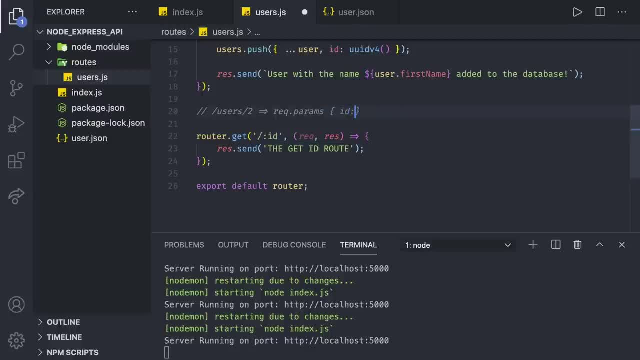 have is the id. so we're going to have an object and the id is going to be two. of course we don't only want to see comments. let me show you that in action. in here i'm going to do console log, request that params if we save that, or you know what. we can also show that if we do in here. 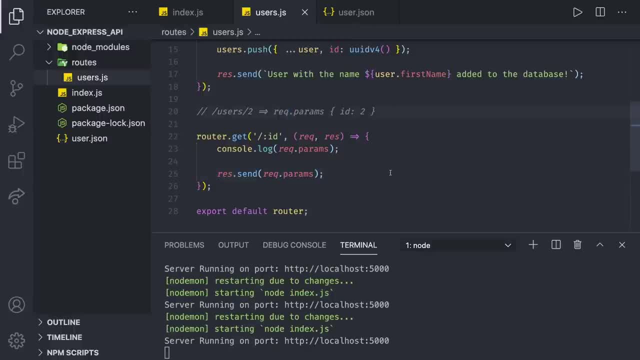 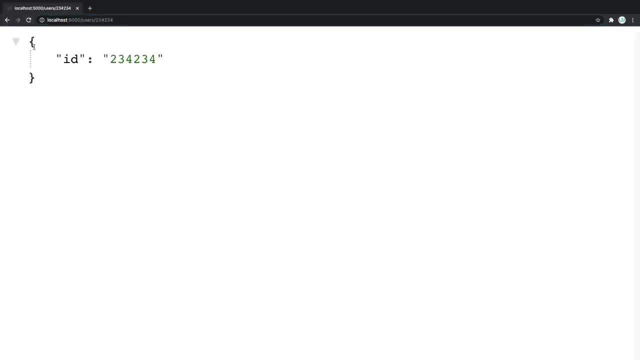 reg that params. now it's going to show in the browser as well, so let's go back, do one more request to, let's say, this url, and now, as you can see, we do get an object that has the value of our id. why do we need that? well, because we want to access the data of the user's id. 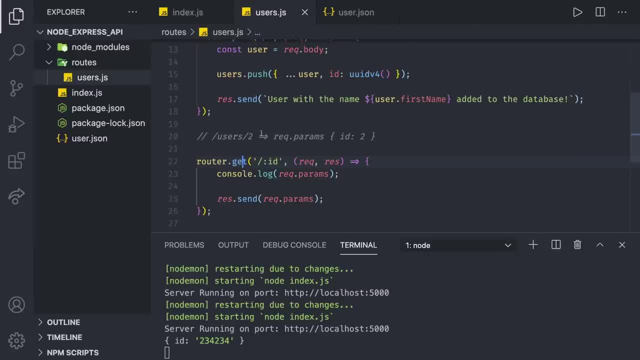 specified right in here. great, now we know that we get the id to direct that params. so let's do: const. id is equal to reg, that params, that id, and you can also use destruction here. so we just take the id value from the regular params- great. but we don't only want to send the id. that doesn't make any. 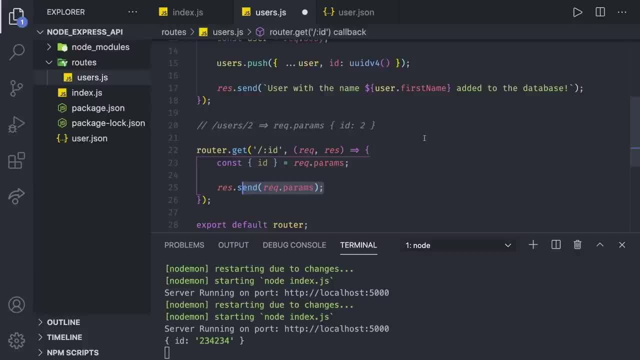 sense we want to send the user data for a specific id. for that to work, we need to find a user in our user's database that has the same id, so we can do users that find in here. we get each user. and what are we searching for? well, we are searching for if the user, that id, is equal to the id right there. 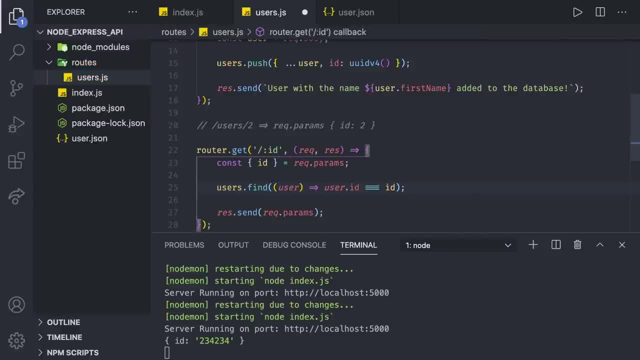 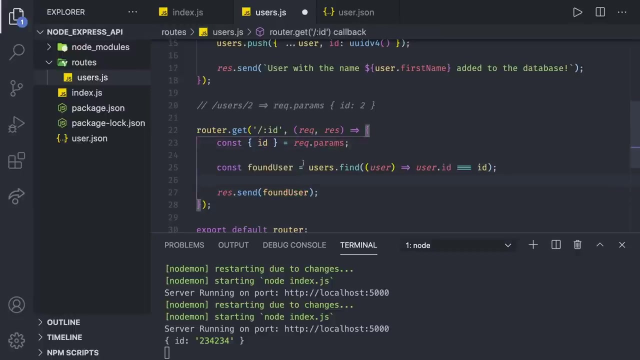 if that's the case, then we're going to get the user. let's try putting that into a new variable, const found user- and let's try doing a. let's just. let's just try to return it. so instead of returning regparams, we'll return the found user. let's see if that's gonna work. now, of course, if 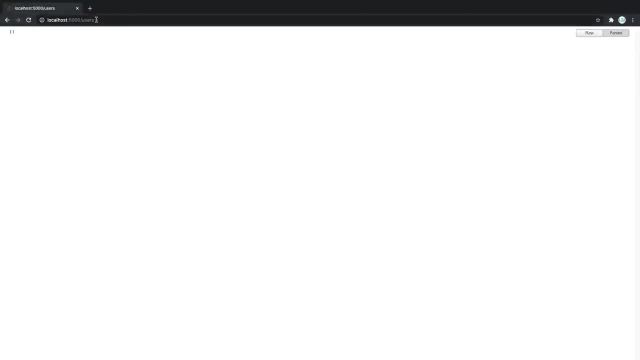 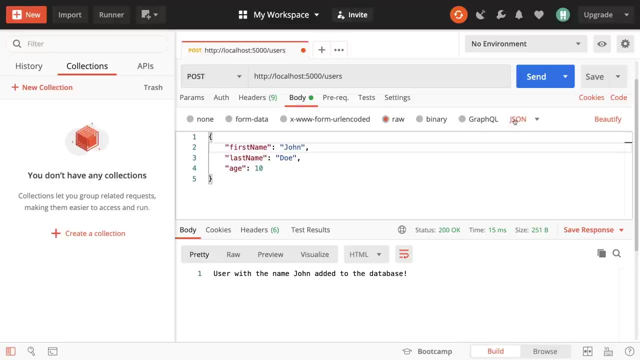 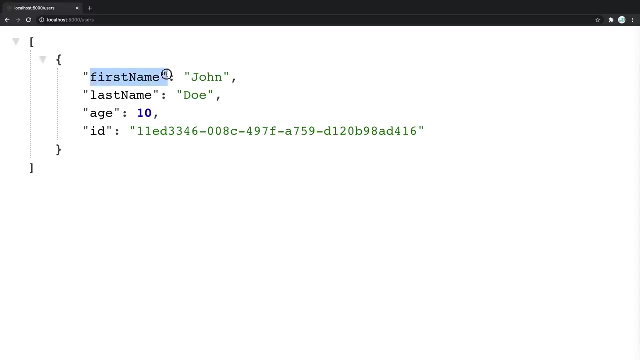 we go back just to slash users. we don't have any users right now because we need to add them, so let's go to postman make another post request with the john doe. great, we just populated the array. if we refresh, we now see the john doe with the id. that's nothing special. let's add one more person. 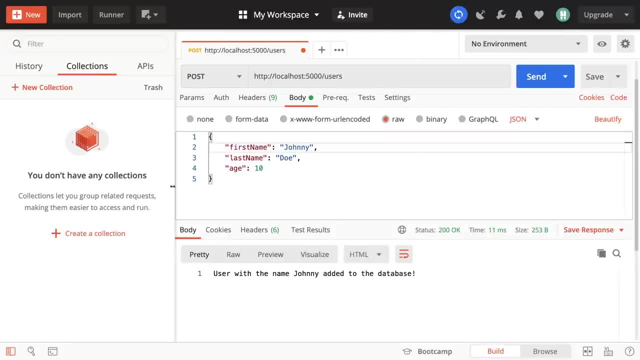 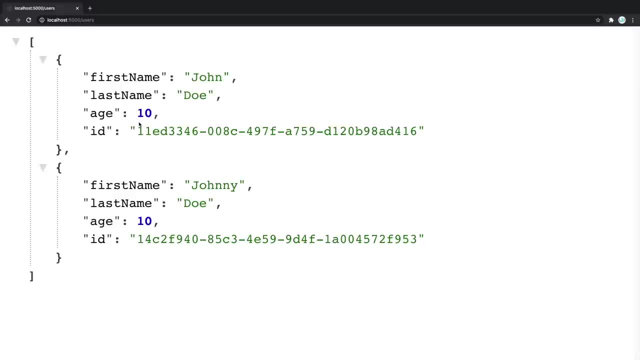 there, johnny, for example. okay, if you refresh one more time, we do get another object. but what's special now is that each user can look at his own profile, or right now, everyone can look at everyone's profile because we don't have any authentication. but if we take this id here, 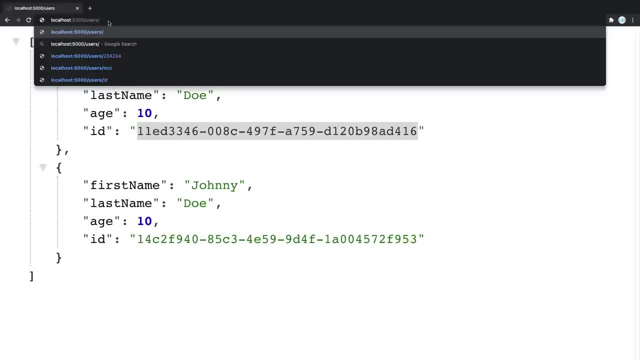 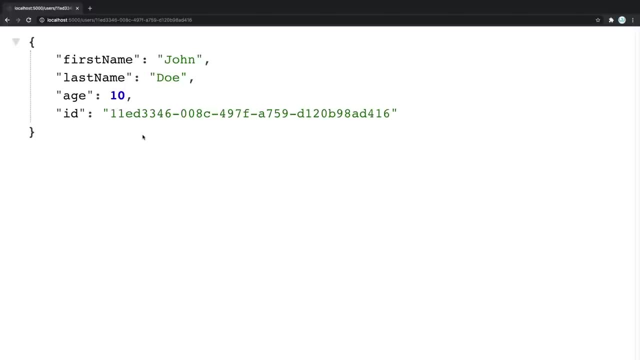 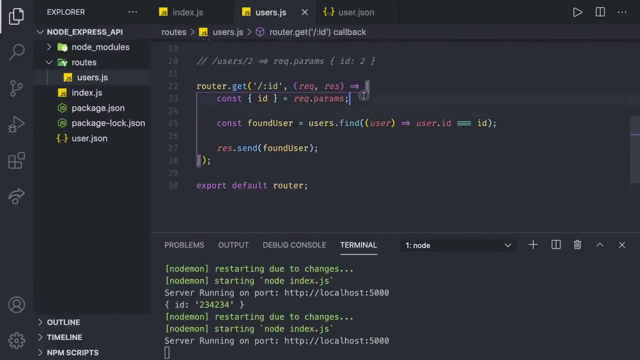 and then go to slash users, slash and put that id in. now we get the data only for that specific profile. that's great. the advancement to this would be for the user to be able to edit some of things only under the id of this user, or also that we can delete the user by certain id. so let's implement these routes now we know. 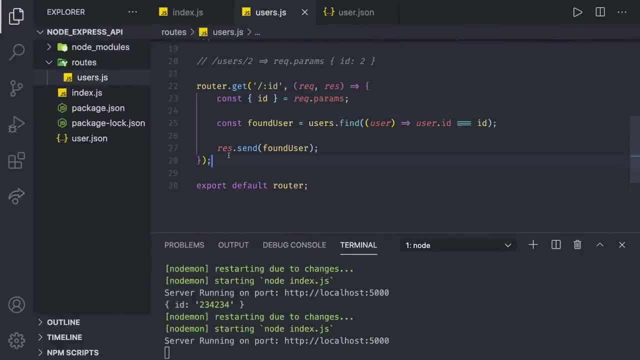 how we need to use the route parameters to make this work. so let's create another route. the route we are going to add next is going to be routerdata delete. so this route is going to be for deleting users. which users do we want to delete? well, only. 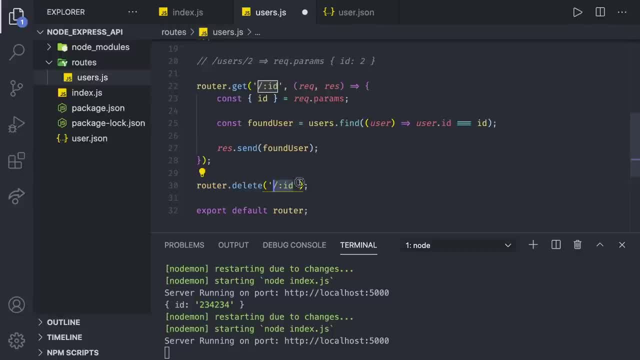 the user specified in the query parameters. then again we do a callback function where we have the request and the response and afterwards of course we need to get the id one more time from the requestparams. and now we want to remove that element from the array. for that we can use the. 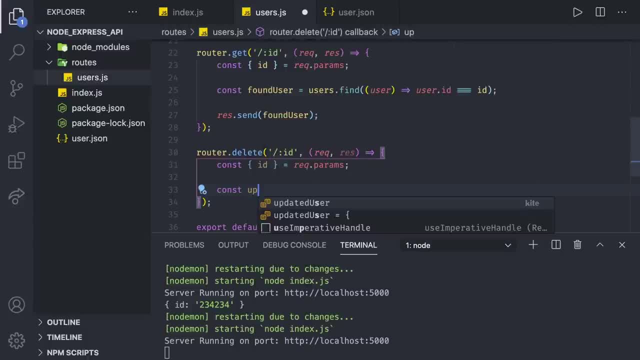 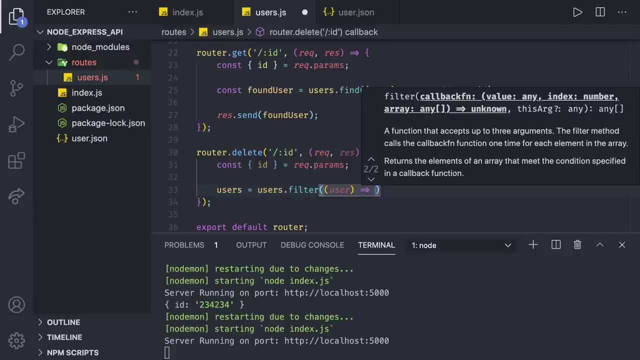 filter function. let's say, let's say users is equal to, and now we need to filter out the user's array. so users that filter in here we get an each user for each iteration and then filter function works so that if whatever is here returned is equal to true, it keeps that user in the array, but if it is false, 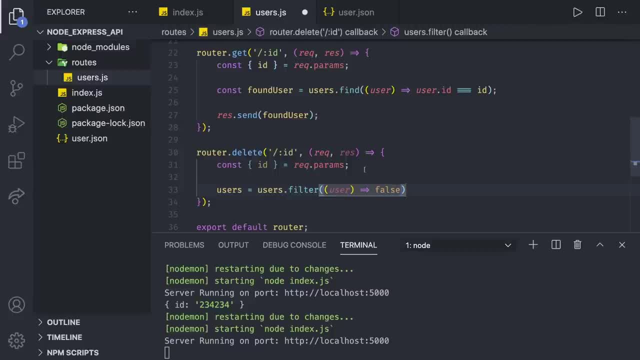 then it removes it from the array. so we want to keep all the users except the one whose id is equal to the id we have here. with that said, how are we going to make the logic of this work? well, let's say that we have john- john has an id of one to three and we also have johnny. or let's say: 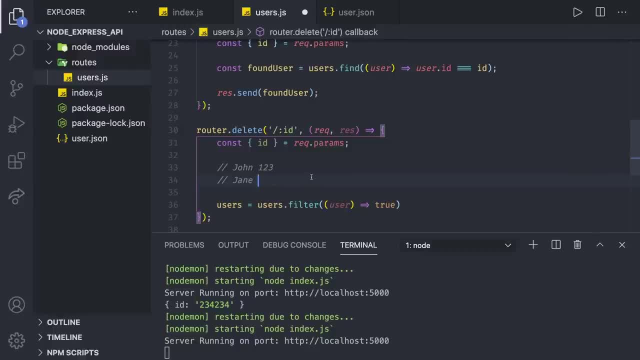 jay. now, uh, we, we mentioned johnny too many times. uh, jane has the id of three to one and the id we specified id to delete is equal to one to three, for example. great, so now we go into this function user the first time. the user is john and the user that id is equal to one to three. so we want to do. 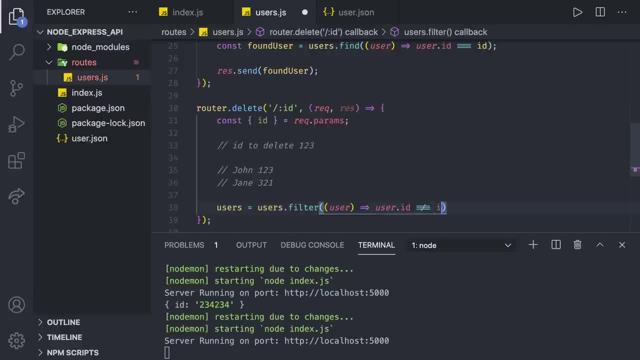 false for that. so we do not equal to id, and that's it. so let's explain one more time. how does this work? for the first iteration, the user is going to be john and his id is going to be one to three. the id we want to delete is also going to be one to three. 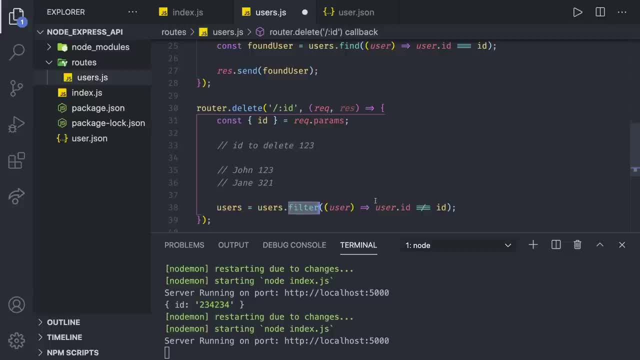 so we set that the filter function works so that it removes the elements for those that the function returned false. since we have an inequality operator here and these two are equal, this is going to return false and therefore user john is going to be deleted from the array. i know it might. 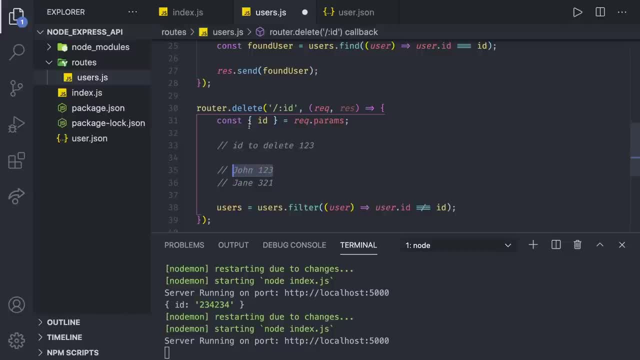 be a bit confusing, but once you go through it a few times it's going to start making sense. now, if we go for the jane, jane's id is 321 and the filter function works so that it removes the elements for those that the function returned false. 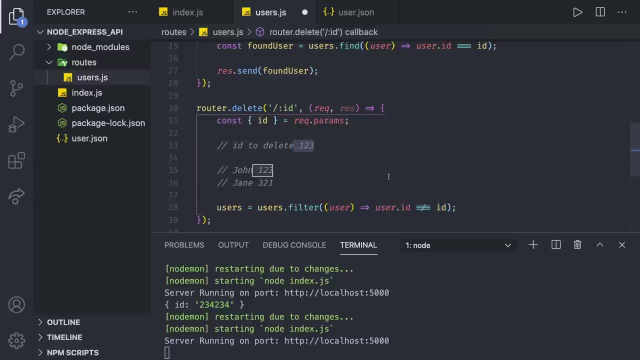 and 321 is indeed not equal to 1 to 3, which is true, so we keep jane in the array. if we do this now, our delete route should work. but let's also send some information to the user, ressend user with the id and then we can use the template strings id. 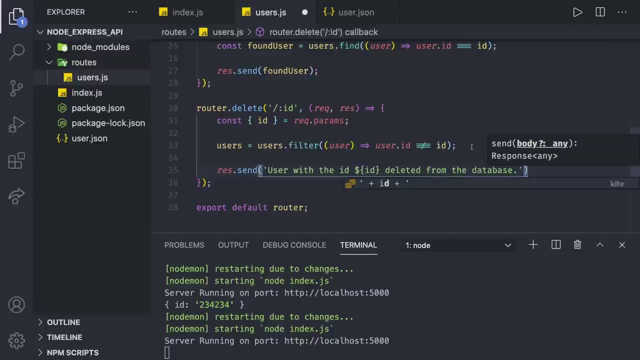 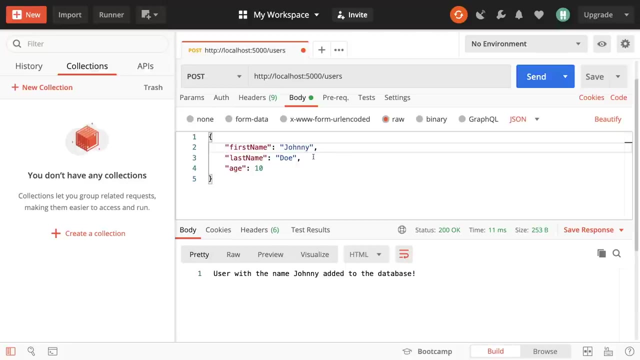 deleted from the database just like that, and we need to change this to be template strings. okay, so now, if we test that out, let's go back to the postman. remember we cannot make delete requests or any other requests other than get requests from the browser. so we need to go back. 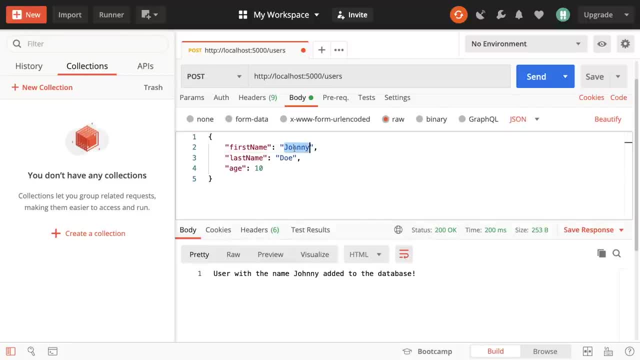 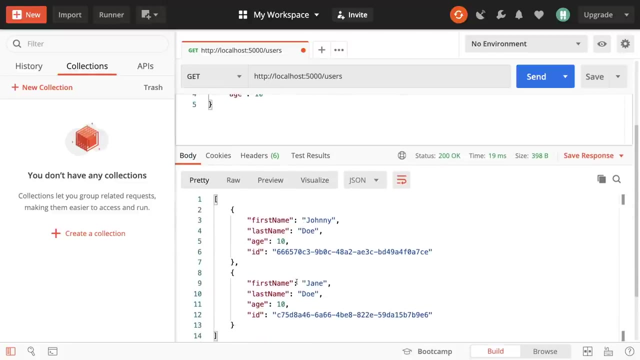 here. let's create johnny. let's also create jane. you can see jane added to the database and now, if you make a get request, we should be able to see all the users and you can see them right here. first name johnny and first name jane, with their own crisp. 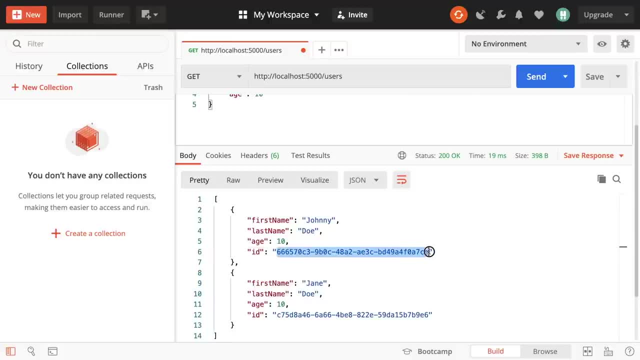 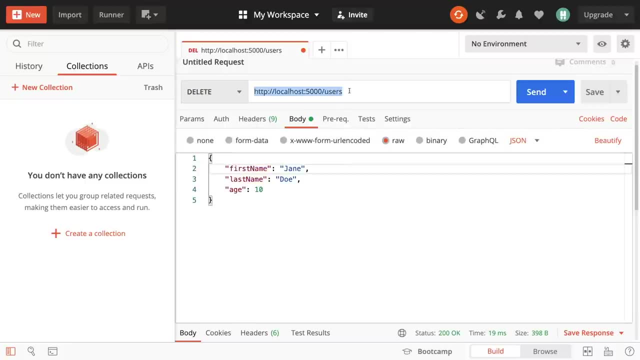 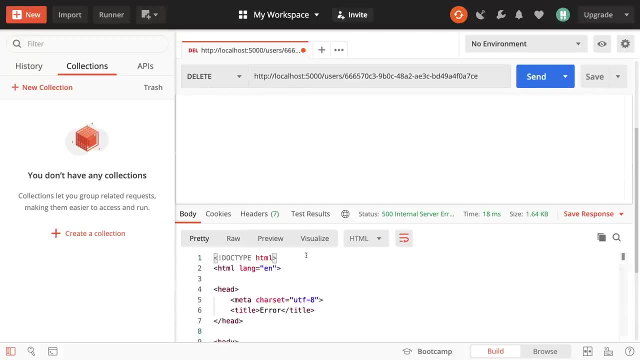 corresponding id. now, if we want to remove johnny, we take his id, go here, change this to be a delete request and just do slash users slash his id with that. if, if we send it, we should be able to get request. in this case we get assignment to const that. 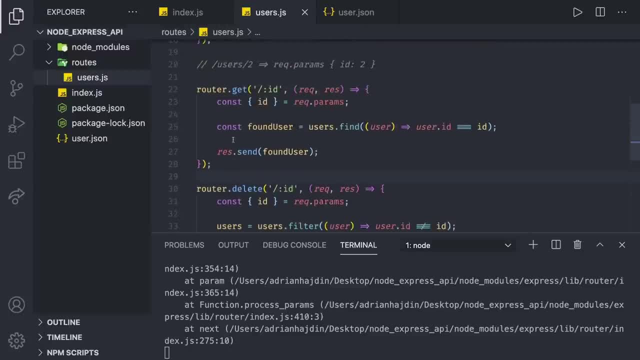 variable. that's, of course, not good. i forgot to change this from const to let because in this case, theants verbal is analyst, so we should also be able to apply const to len JavaScript in this example, adding constant with E word like that. we'll have a lesson for that, so that it's okay with it, because in an example you could give us a Flynn case: if we use const 20, stem Android. i forgot to change this from const to let. 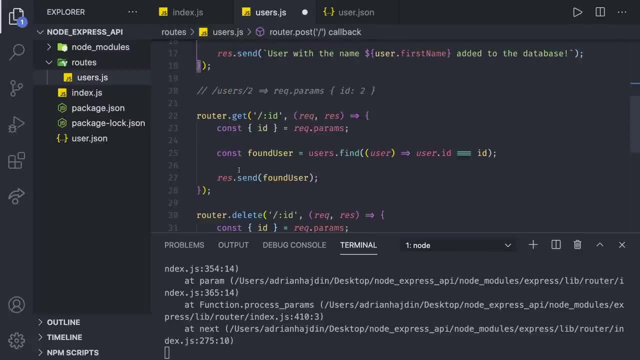 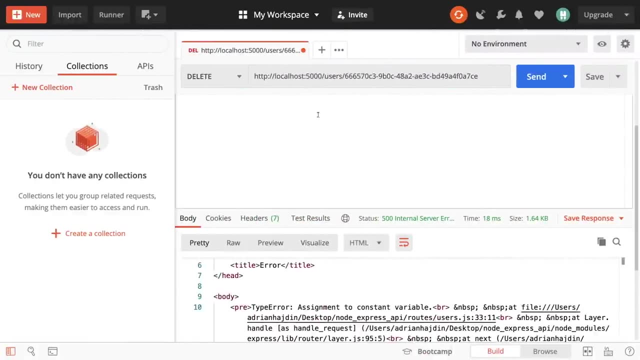 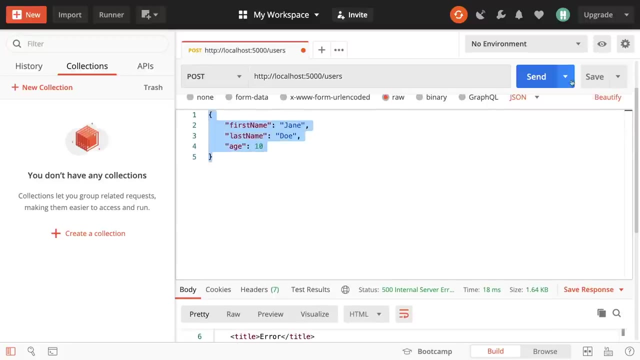 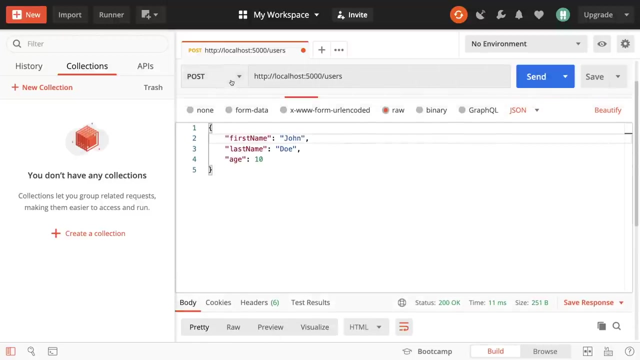 because in this case, we are changing the users array, as you can see right here. so let's save that. let's add two users one more time. so we go to the post, delete this and do we have? yeah, we have our jane. create that, create john. and then we go to the get just to make sure that users are. 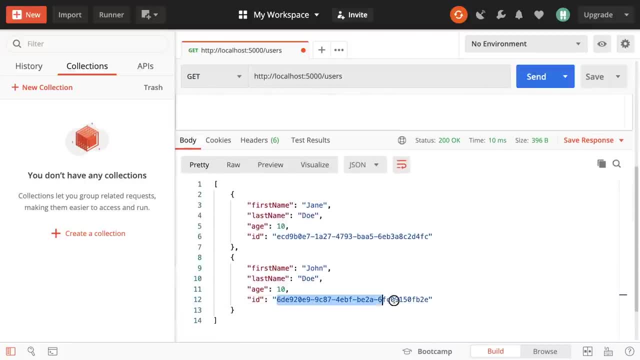 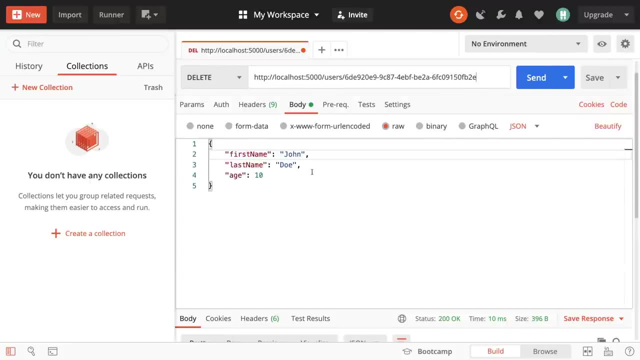 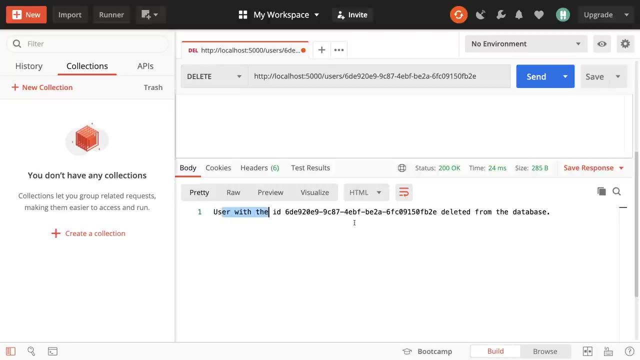 there they are. we take john's id, we go to delete request and then append that to the url: append his id. if we send that, the user should be deleted and we see user with the id deleted from the database. but now when we go to the get of the users, we should see that john is no longer there. we only 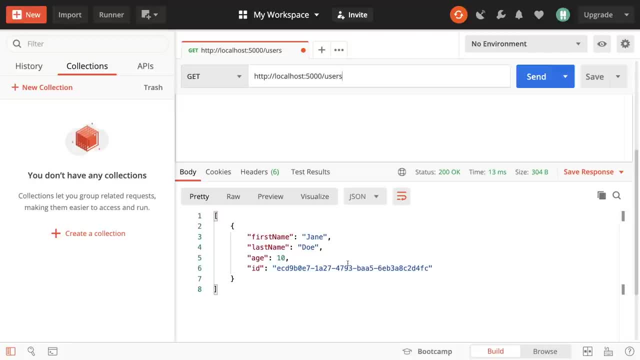 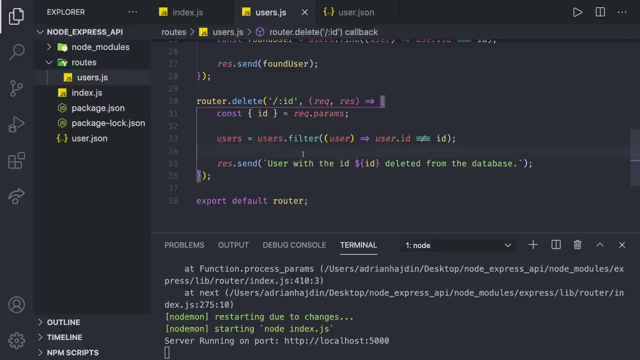 have jane, which means that our delete request will be deleted from the database and we can see that the user is no longer there. works completely great. again in here we are just using the users array, but in the real database, in the mongo db, for example- you'd be using real methods to access the user from the database. 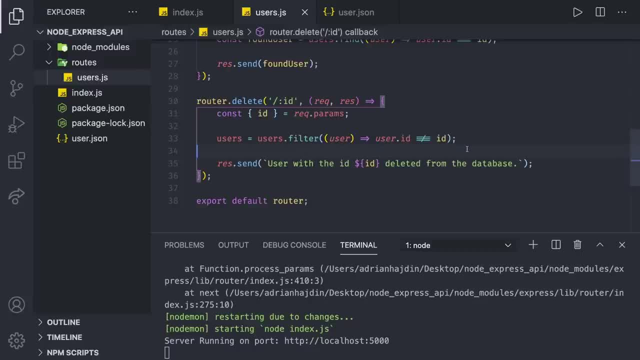 and also to change or delete users from the database again. if you'd like that, just let me know. i'm going to create a video on that as well. great, with that out of the way, we only have one thing left to do, and that is to change the user details. for example, if john wants to change his 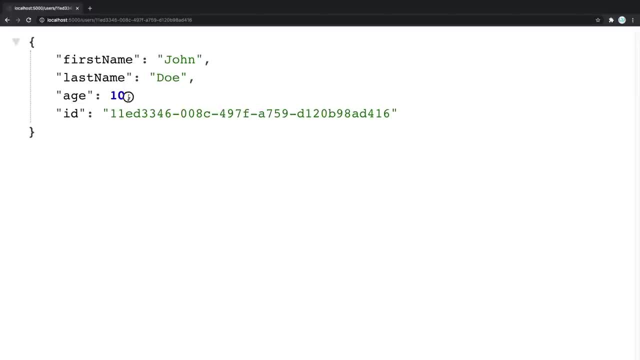 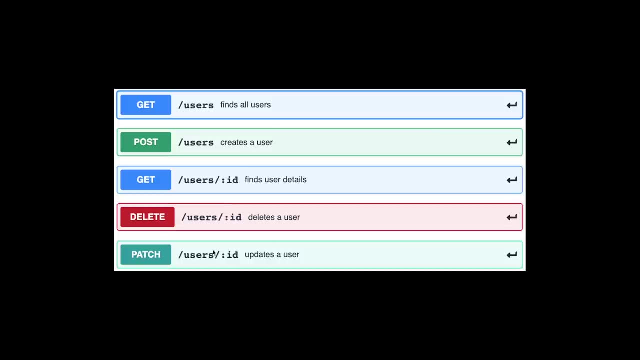 first name or the last name. he should be able to do that. so we're going to create a new user link and we should be able to do that. or maybe age- each year he can update his age. great, to update the user. you can see here we'll be using a patch request. patch is used when we want. 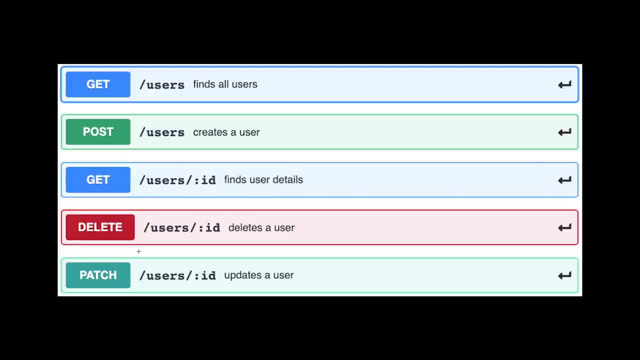 to partially modify something. when you want to create something completely new, then you use post. when you want to get something, you just get, of course. when you want to delete, you use the lead. but with update it's a bit confusing. we have a patch method and we also have a put method. put is used when you want to completely overwrite something. so 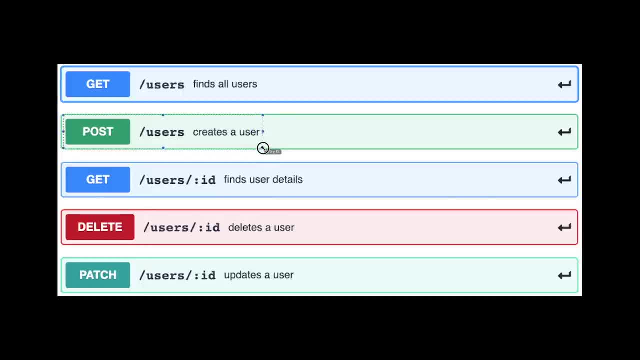 if you want to change everything there is in the user, in that case you would use a so-called put method, but to apply a partial modification- meaning if you just want to change the age or just the name or the name and the age doesn't really matter, then we use a patch and that's a perfect method. 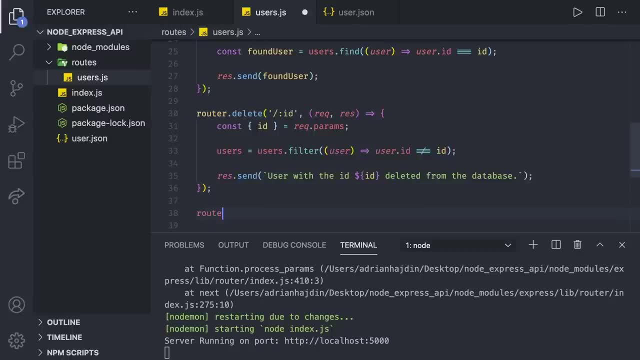 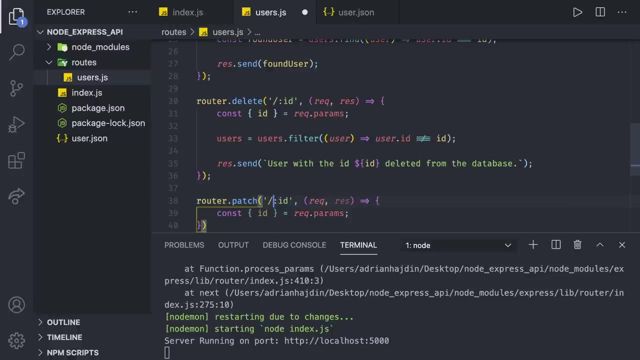 for our use case. so let's go there and we'll do router that patch and the path is again going to be the dynamic id, because we want to know which user do we want to update. then we have the request and the response. we also get the id. don't forget the forward slash. here and now, how are we going? 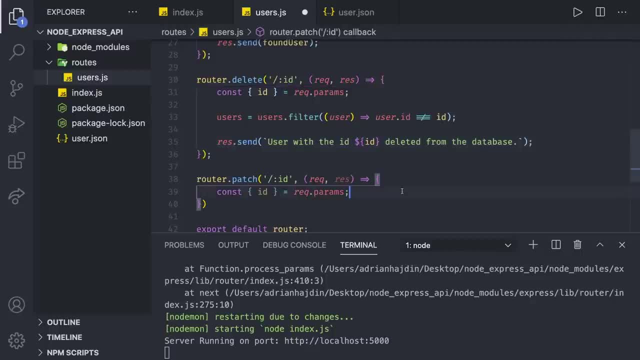 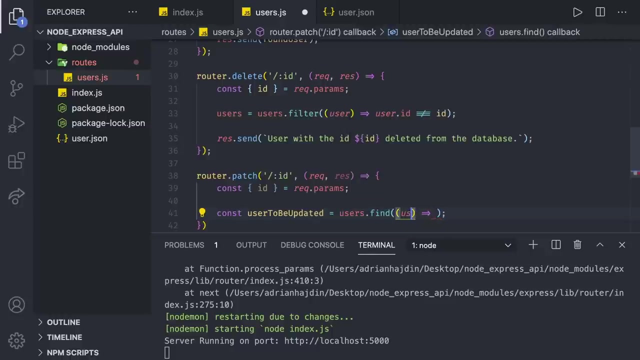 to update that specific user. well, first we need to find the user to be updated. so let's say, user to be updated, and how are we going to find him? well, using the usersfind, or rather arrayfind, method. arrayfind goes through a lot of different users or elements in the array, and then the first one. 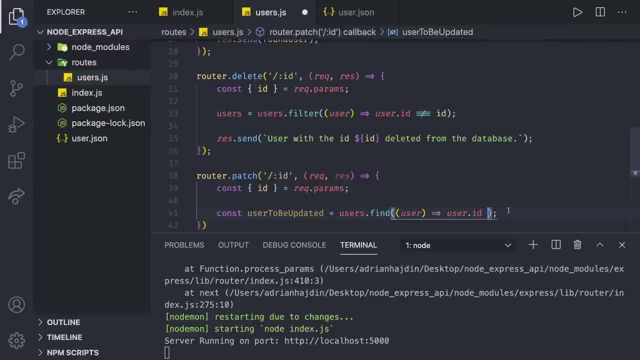 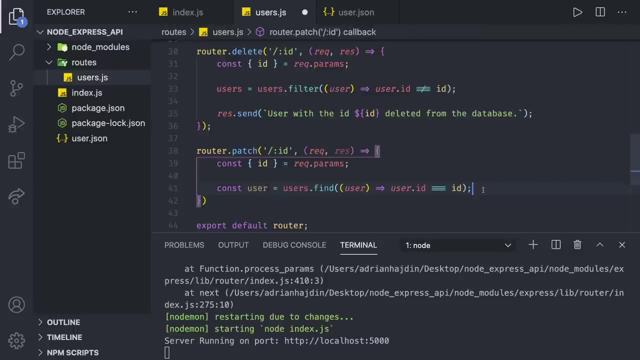 that matches it, returns it. so what do we need to match? well, we need to match the user's id, so userid, to the id coming from requestparameters, and then it's going to return the user to be updated. updated. once we have that user, let's, let's just rename it to user because, uh, user to be updated. 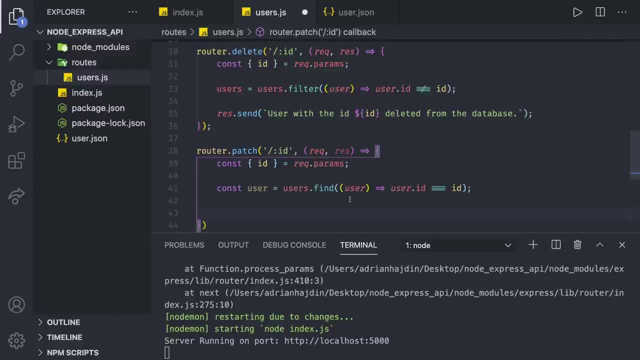 is a mouthful. so once we have that, user patch is going to be the most complicated method in here. we use, as you can see, query parameters to get the id, but also we're going to send something from the client sites for something from the postman, and what is that something going to be? 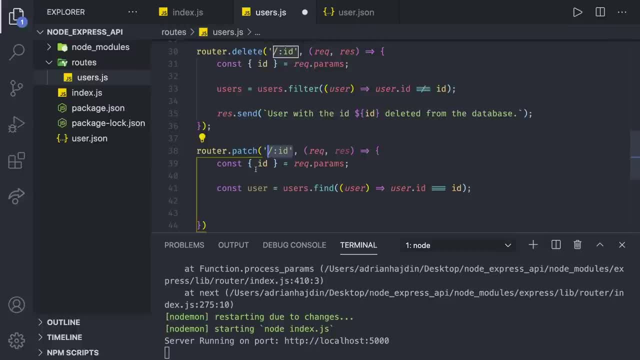 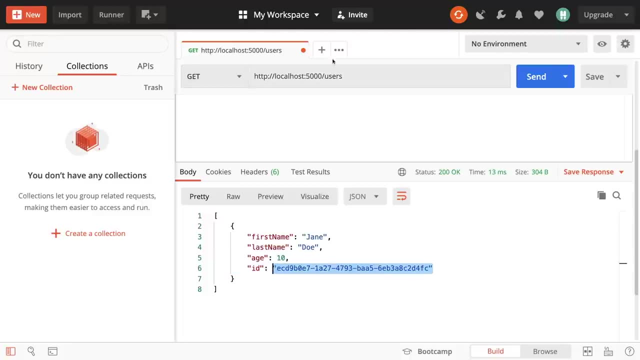 well that something is going to be, things we want to replace. so if we go back from the client site right here- and we do, let's take this id which we have right now, we put it after the users. in this case, we'll be doing a patch request, so let's go to the patch and now we're going to send. what do? 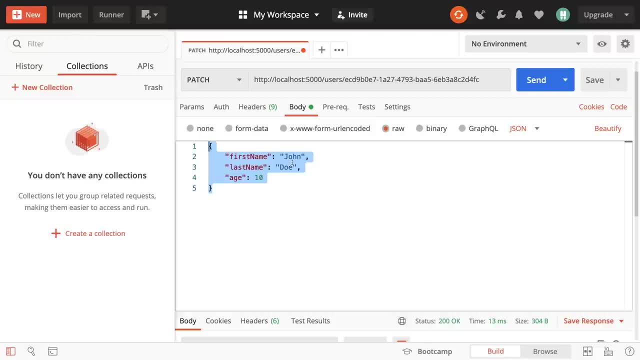 we want to update. so in this case, we want to send something like, let's say, first name equal to johnny and then that's going to update the current first name of the user with this id. now that we know that, we know that we're going to receive some data, 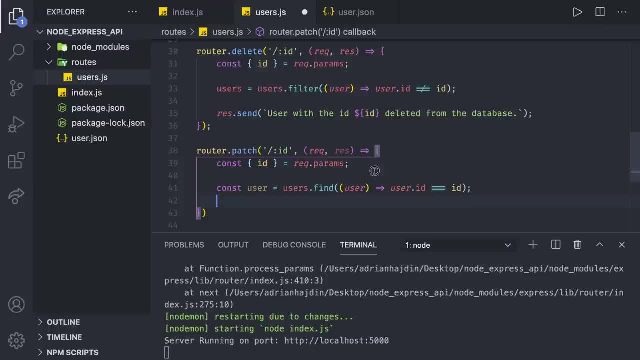 through the requestbody. so let's take these things out. what can we receive? we can receive the first name. we can also receive the last name and the age. of course, user shouldn't be able to change his id. we take that from requestbody and then we can change those things. just a simple if. 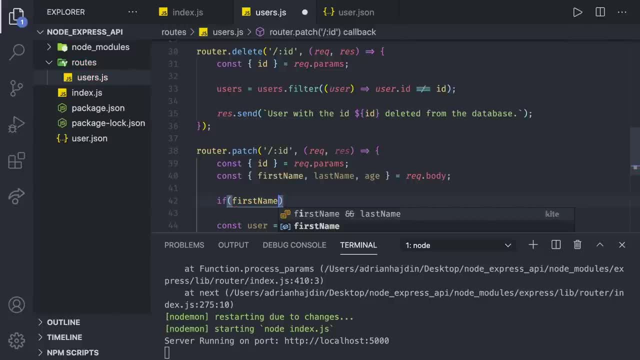 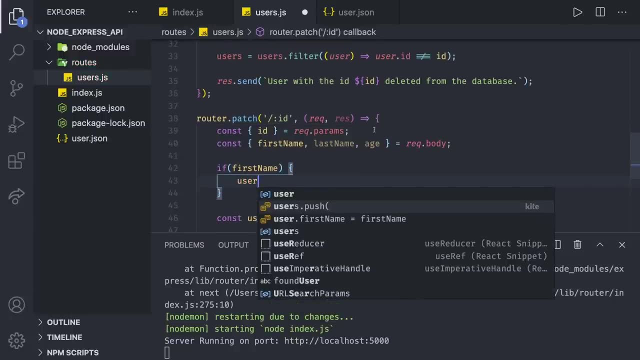 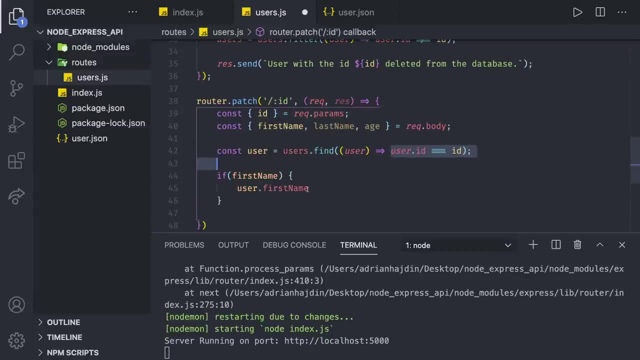 statement to check if there is a first name. if there is a first name, then we're going to set the user- that first name user, of course being this user here which we found, which we want to update, to be simply first name- and then we can repeat this for everything, for example: 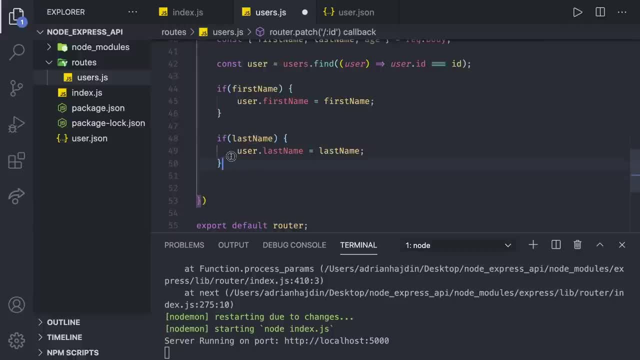 in here for the last name and also- we can repeat this one more time- for the age. so if there is age, then userage is equal to age. with this, we can now change one or many different properties of the user. just to go through this one more time, because patch, indeed, is the most. 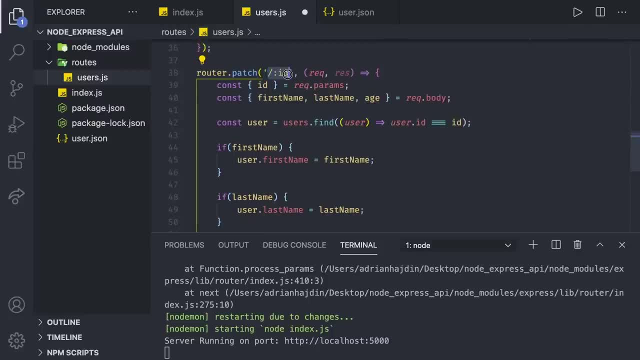 complicated function. here we are receiving a request parameter, as you can see here, which is the id. that id specifies which user do we want to update. we find it here using the find method and then we take all the things coming from the request of the body. remember we send these. 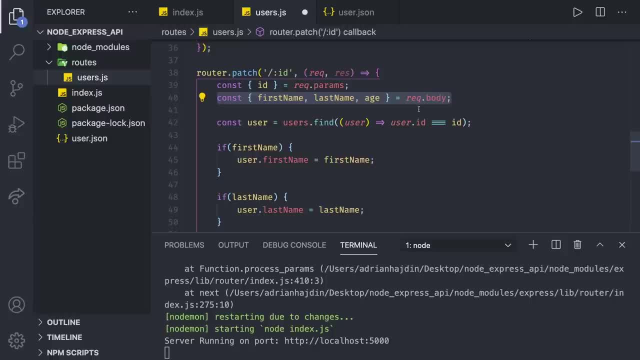 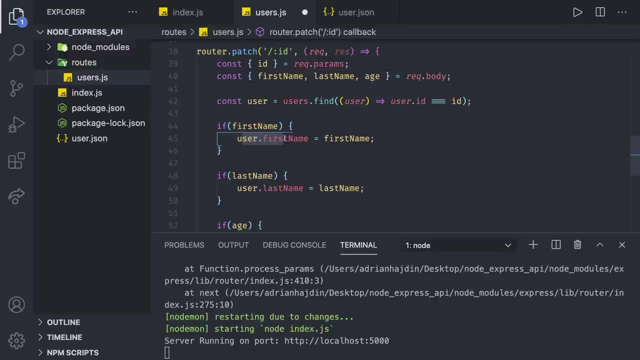 ourselves from the front end or the client, in this case postman, and then, if we have the values which we want to replace something with, then we change the user that first name with the first name, users that last name with the last name and users that age with the age. we can also write this: 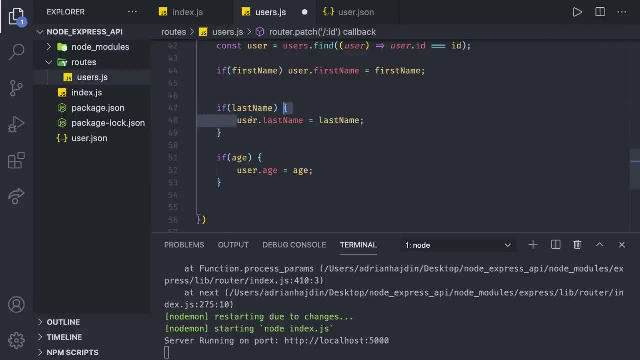 in single line by removing the curly braces, because this is a single line if statement, and then it's going to look a bit cleaner. so let's leave it like this. and also now we can do a console log or just ressend user with the id, and then, of course, we can specify the id. 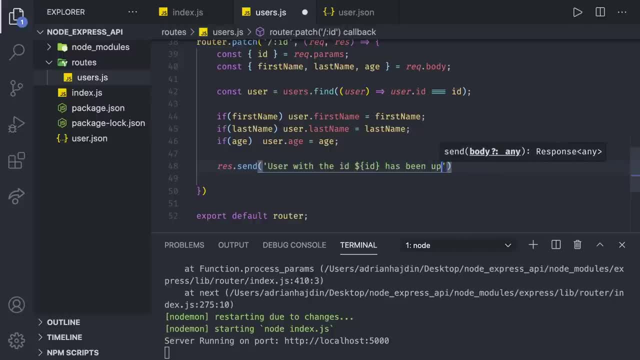 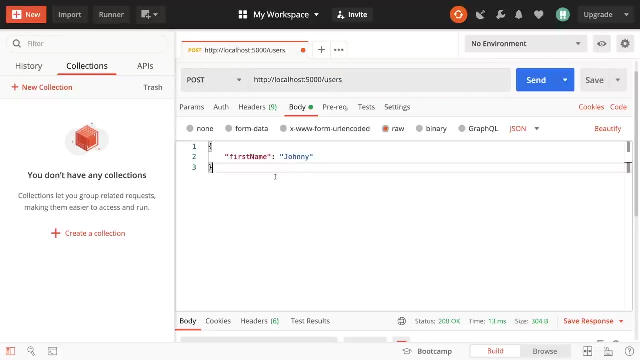 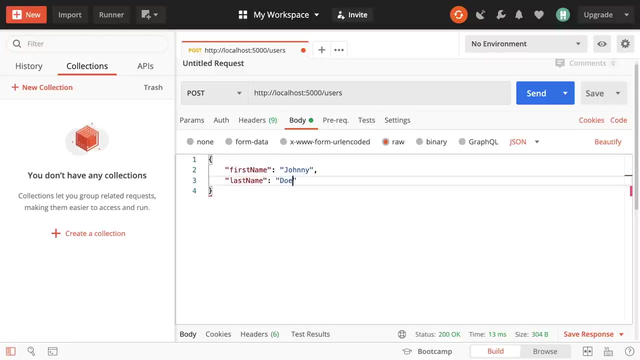 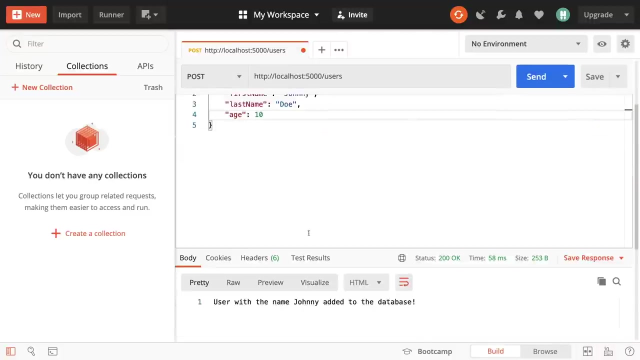 has been updated. that's it. okay. if we test that out, we should be able to go back to the postman, create one user first, so post to these slash users, and we need to have everything in the post. so, first name, johnny, last name, though, and the age is equal to 10. okay, we send that. we should get a response saying user with. 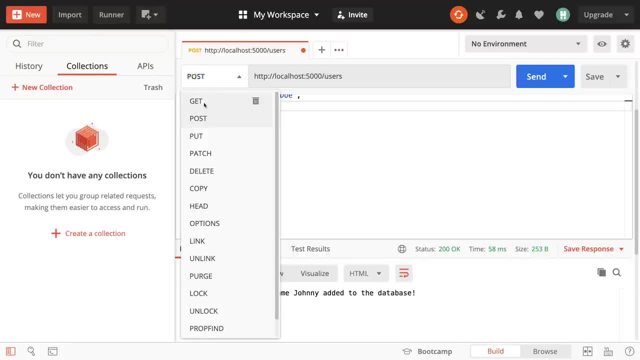 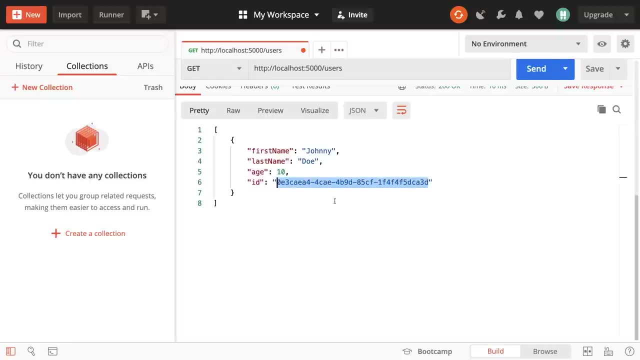 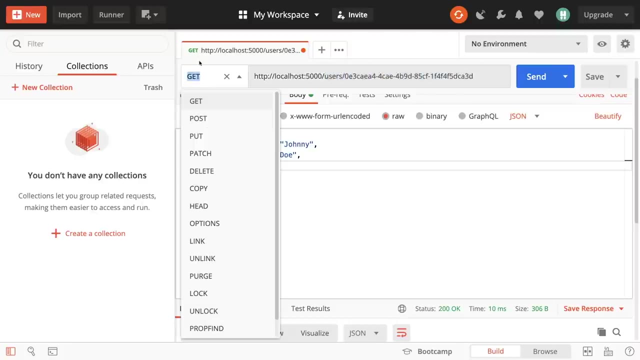 the name johnny added to the database. let's make a get request, just to be 100% sure. okay, we do get it. and now we have this id, now we can add that id to the url so that we know about which user are we talking about, and then we can make a patch request to that. but this time 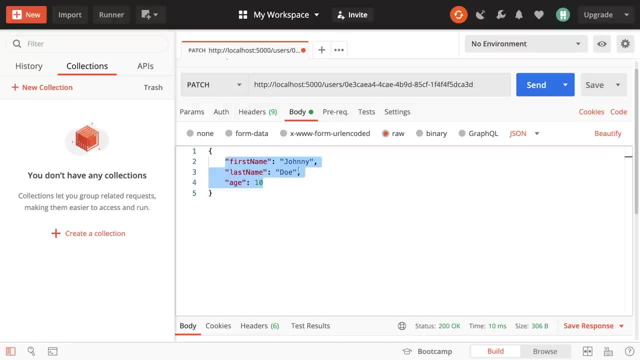 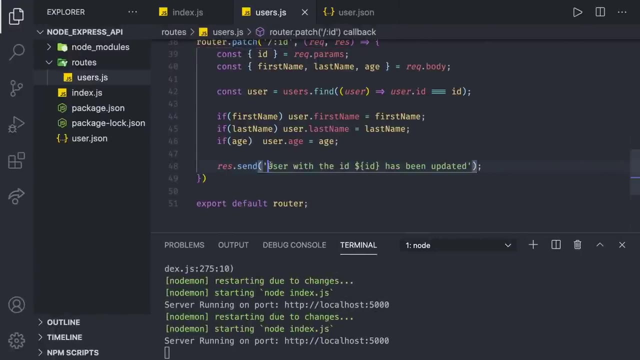 we can include only the things we want to change regarding johnny. so let's say that he just had his birthday and that we just want to change the age. everything else should be left unchanged, and in here you can see user with the id. oh, my bad, there i forgot to make this into a template string. okay, just like that has been. 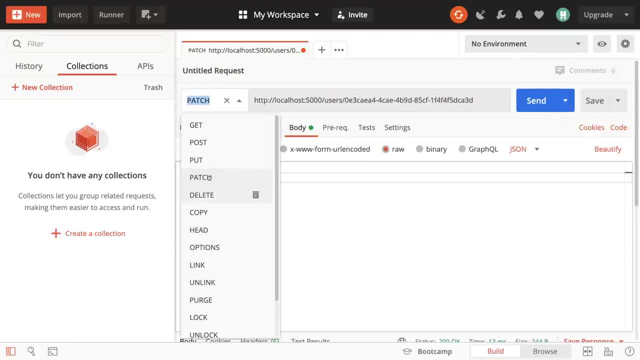 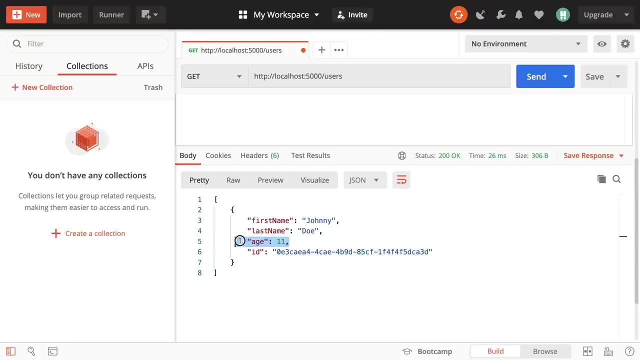 updated. great. now, if we go to the get request to get all the users, we should get the johnny with the age of 11 and all of his other. first name and last name and the id have been left unchanged. amazing, that's exactly what we try to accomplish. our application. 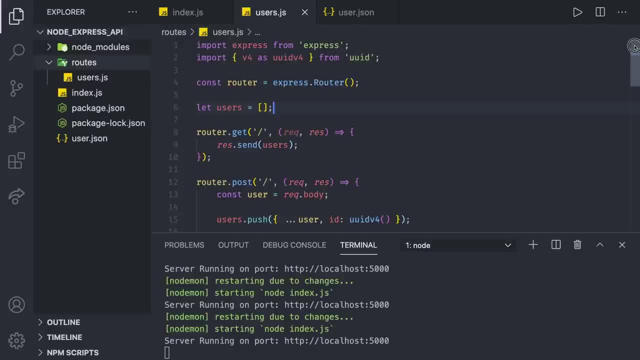 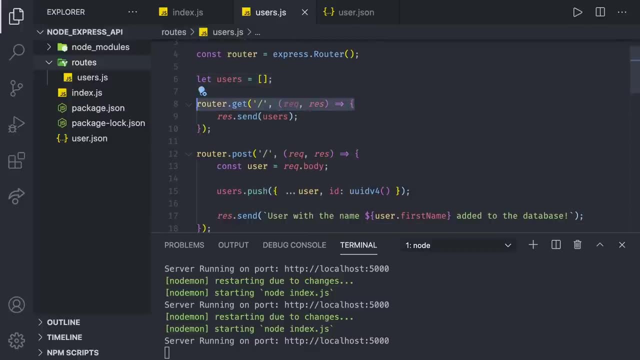 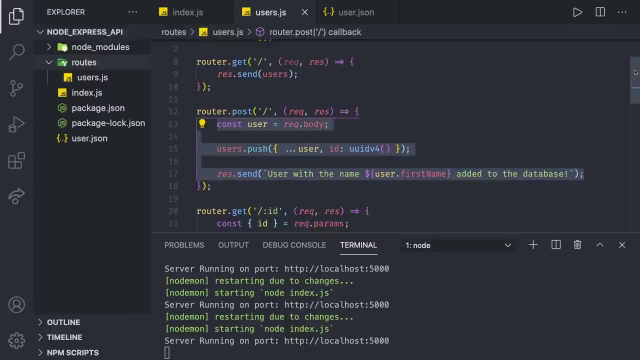 is almost done. i would like to just get your attention to one thing. notice how this user's routes file is not only routes. of course we do have the routes, but these routes have a lot of logic in them and we should try to separate the logic from the routing. if you just keep scrolling, 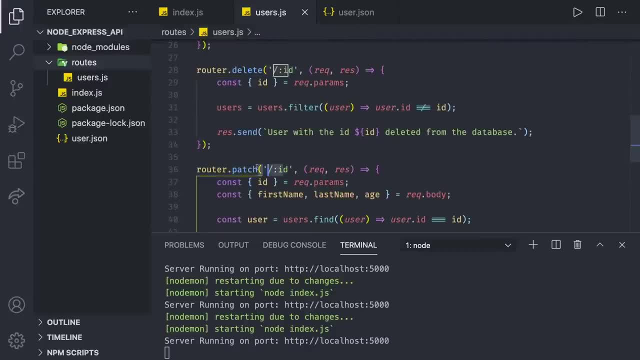 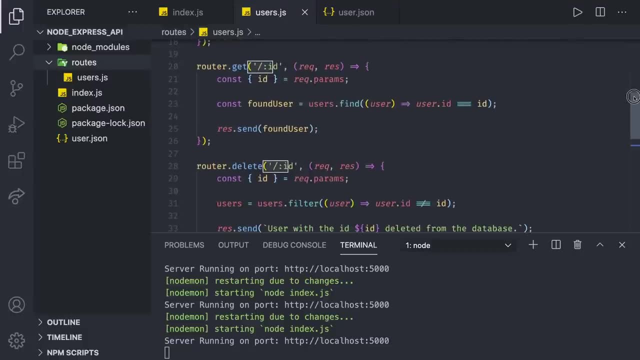 you can easily get lost. we have the delete route, the patch route, then we have two different get routes. you can get lost and maybe not know which route is doing what. so what's the difference between the two routes? we have the get route and the get route. 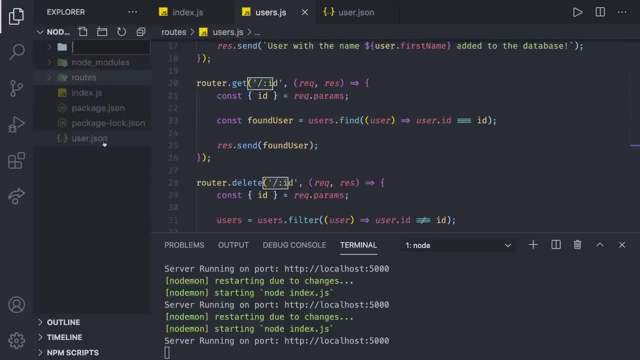 what people usually do is that they create a folder called controllers- controllers. just like this. we created the routes and we created the controllers. inside of the controllers, you can create file with the same name- usersjs. and then what are we going to put into it? well, let me give. 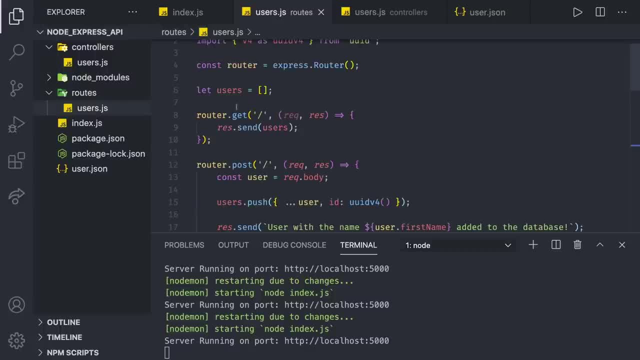 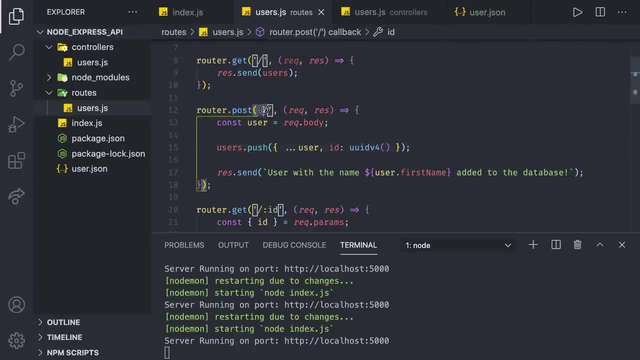 you an example. our first get route is really simple, so let's do something with the post route. the post route has to be the same as the get route. the get route has to be the same as the post route, the first one being the slash route- just slash users- and the second one being callback function. 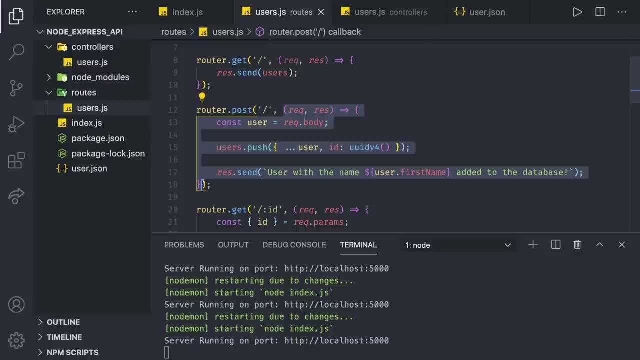 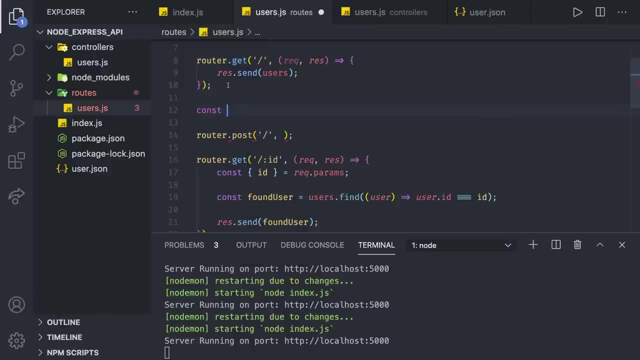 which is going to be executed once someone visits that route. so we can take that and we can separate that into a new function const and that's going to be create user and that's going to be a function. but we don't actually have to create this function block. we just did, we copied it right here. so if i 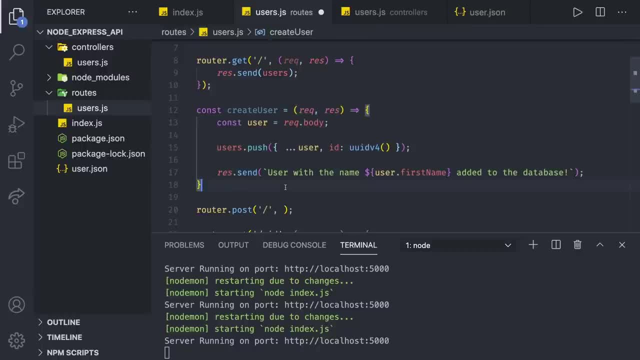 paste this, you can see that it's going to be a function block and then we're going to create a. we can see this is now a separate function, create user function- and it does exactly that: it creates a user. so right now we can just put that here instead of having it immediately in the route. 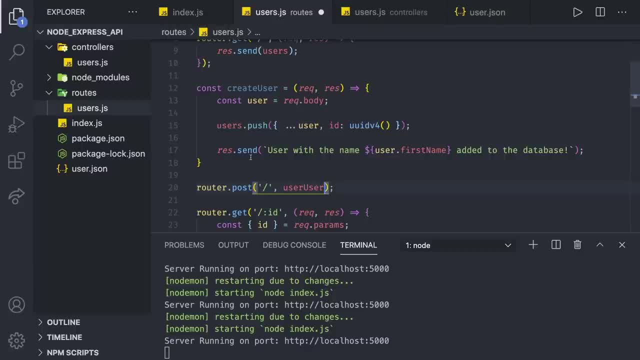 we now took it out into a new function and are using it right there. you may say that this doesn't make a lot of sense, and some may agree. but now we're going to take this function and extract it into a separate file and that file is going to be a user and that's going to be a function block. 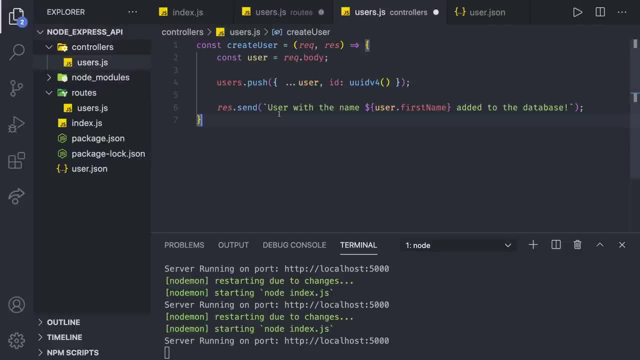 and that's going to be a user and that file is usersjs of the controllers section. in here we have the create user. the only thing we have to do is export it. so export const- create user. once you do that, save the file, head back to the routes and then at the top, make sure to import it. so in here. 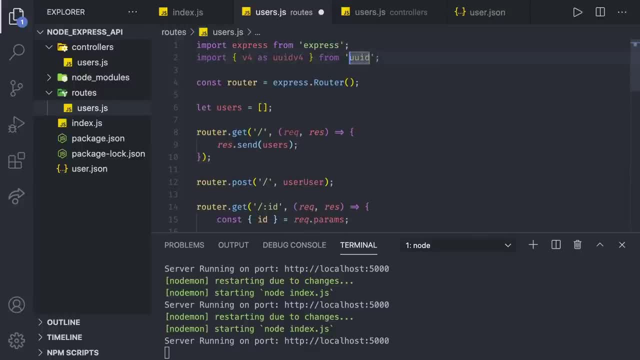 we're going to do import, let's do it after this one: import: curly braces. create user from dot. dot. slash controllers, slash users, dot js. and now, as you can see, we are using this function. i would like you to do the same thing for all the other routes. let me show you how to. 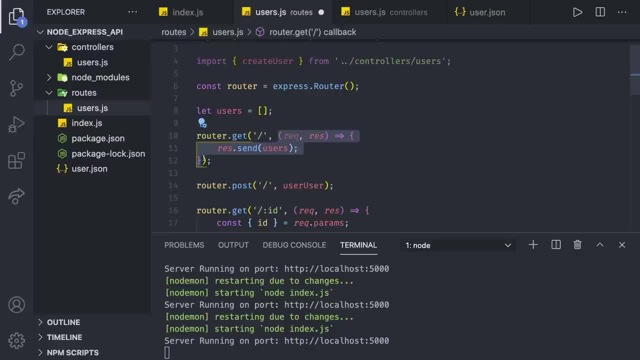 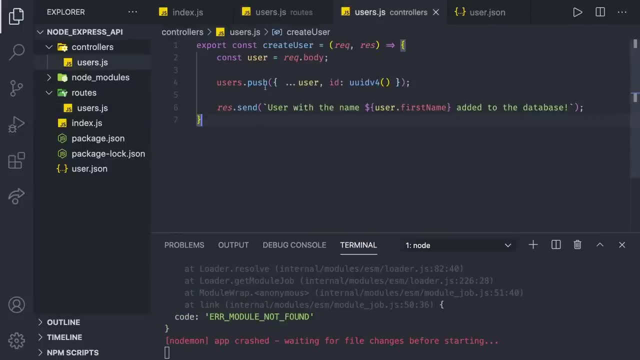 do it for for a few more in here. we're going to take this function, call it get user, and now we can also go to the controllers: export const get user is equal to the get user function, and now we can also go to the controllers: export const get user. and now we can. 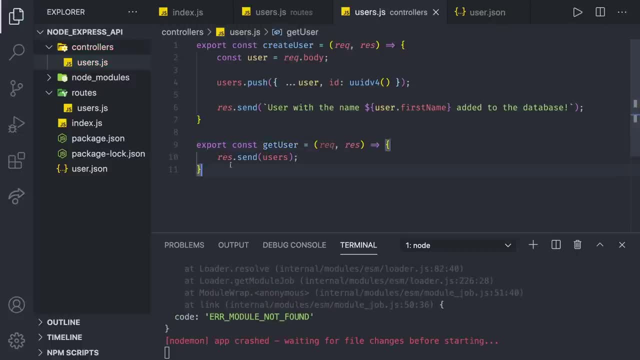 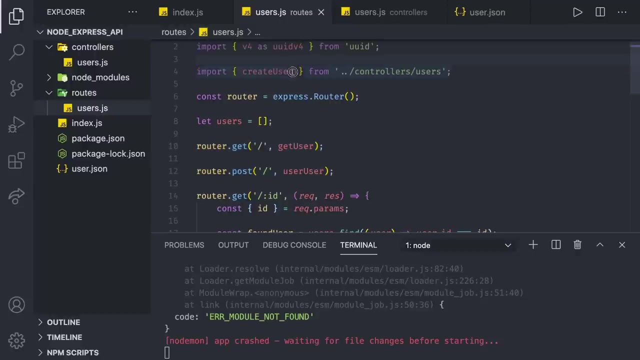 just paste it and that's it. we just transferred the get user function as well as the create user function, so now the functions are in a separate window or a separate file, and all the routes are nicely tucked in here. that's great. we also need to import it, so let's do import get user as well. 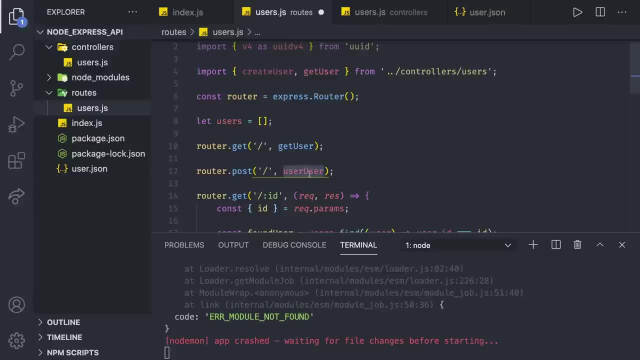 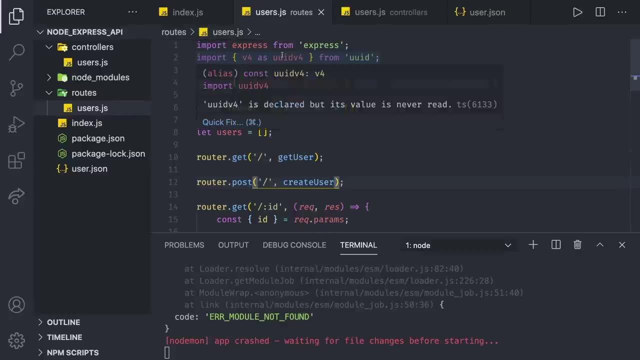 now we have those two and in here, for some reason, i have user. user. it should be create user, so let's do import, get user as well. now we have those two and in here, for some reason, i have user. of course, okay, notice how in here we have this, but it's being unused. it isn't used, so we. 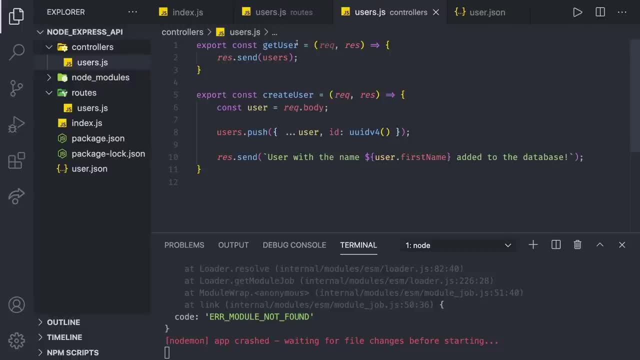 need to take it and move it back to the controllers, because we are using the uuid right in here in the create user, and that's also one way to show you we want to deal with the logic right there in here. we add the ids, we do something different, we import different modules, we return some things, but in 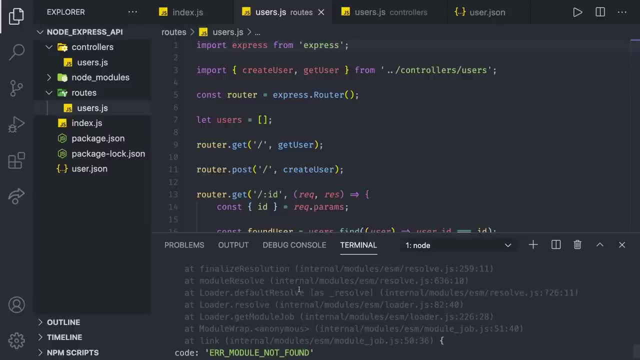 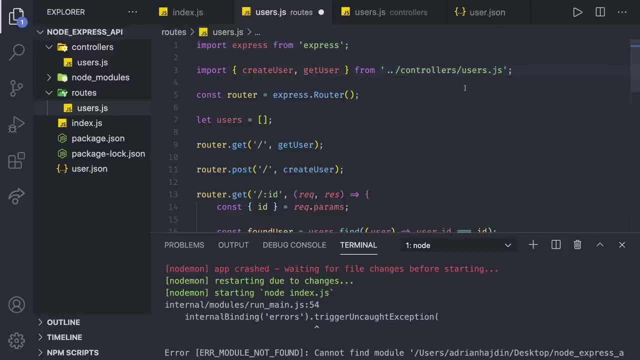 the raw. we only want to have routes. looks like we have an error right now and let's see why is that happening. oh, we are missing the dot js extension right here in the routes. if we add that, we should be fine. server running on port local host http 5000. great. now let's do the same thing for all the 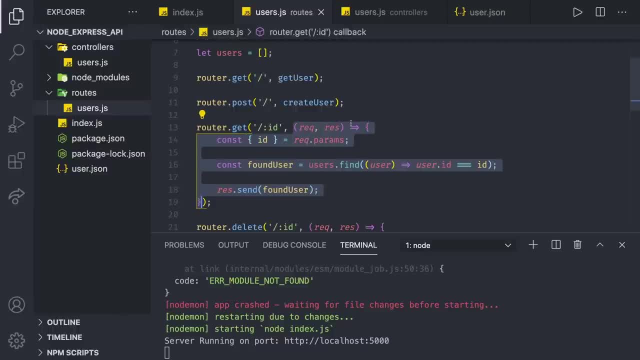 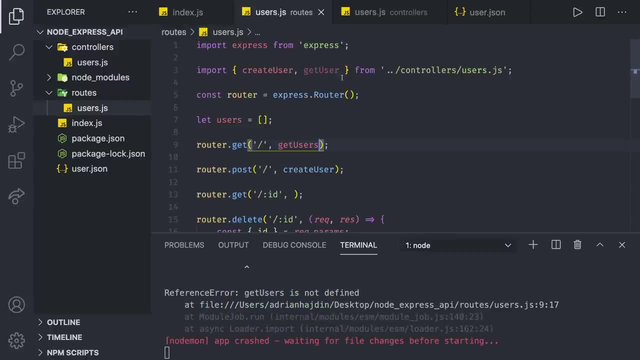 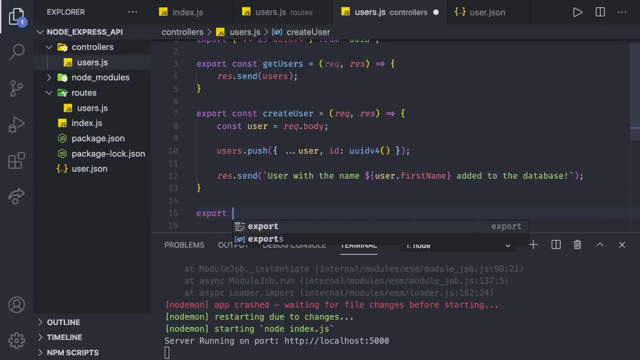 other routes. this one is going to be get user, and again i made an error in here. we have the get users plural because it's getting multiple users, so i'm going to just change that, move to controllers, change it here as well and keep adding more functions. so export, const, get user singular this time and make it. 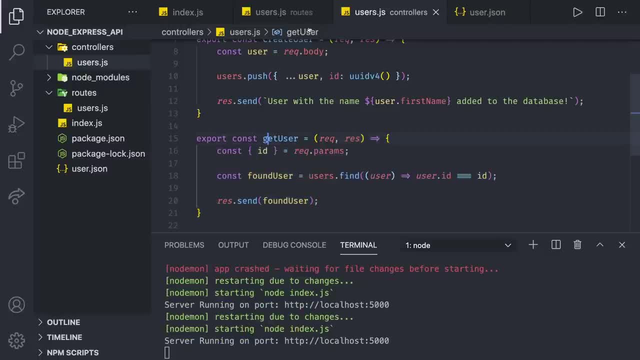 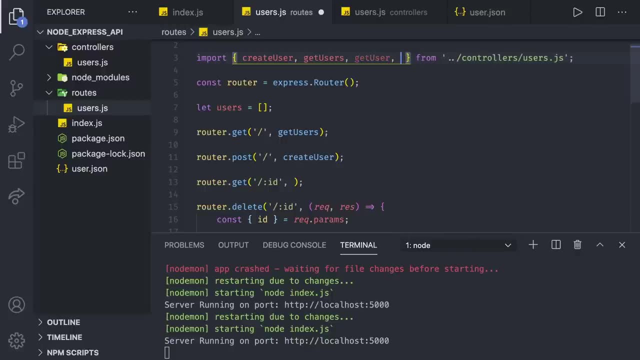 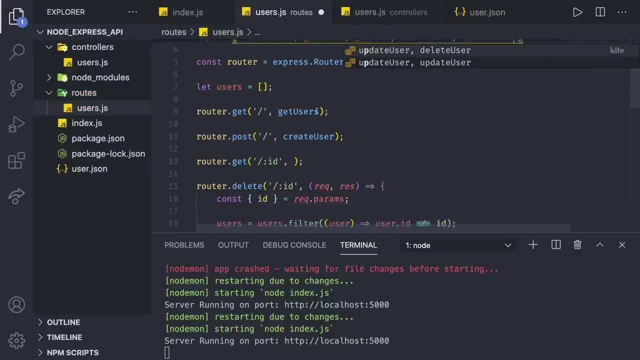 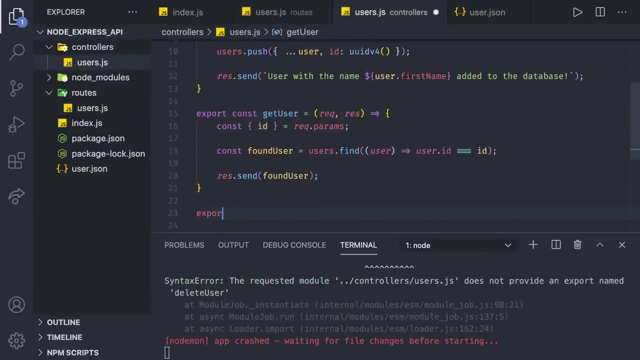 equal to what we just copied there. okay, gonna keep doing that for a few more functions. let's just add all the names here. so get user. then we're gonna have delete user and also update user. okay, let me take the code for the delete user and move to the controllers to add it: export const. delete user is equal to this function, right there. 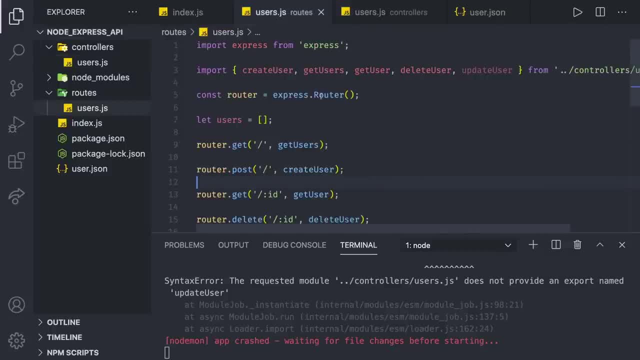 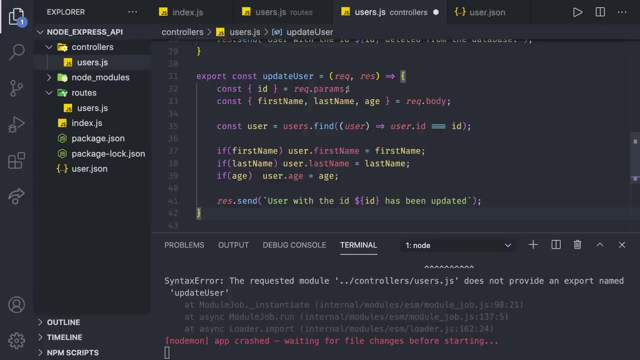 and finally we have one more left, which is the update user, or the patch. i'm gonna take this code, call it update user, and then i'm gonna add the update user, and then i'm gonna add the update user, update user, and then in the controllers, export, const- update user is equal to this whole function. 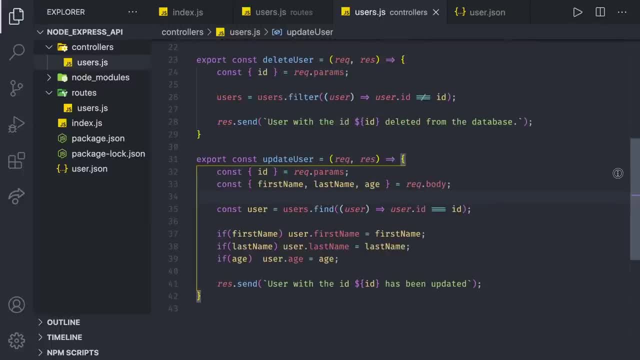 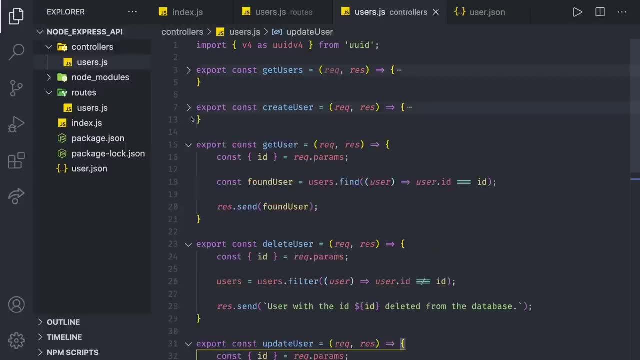 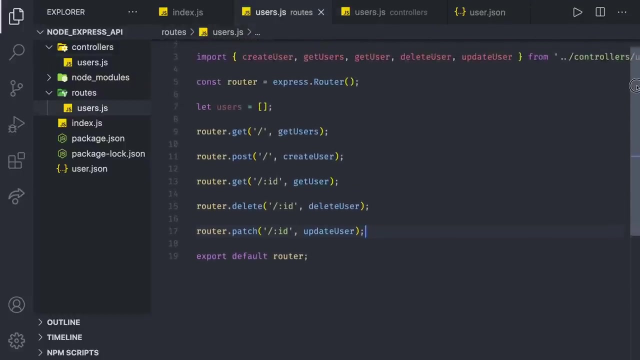 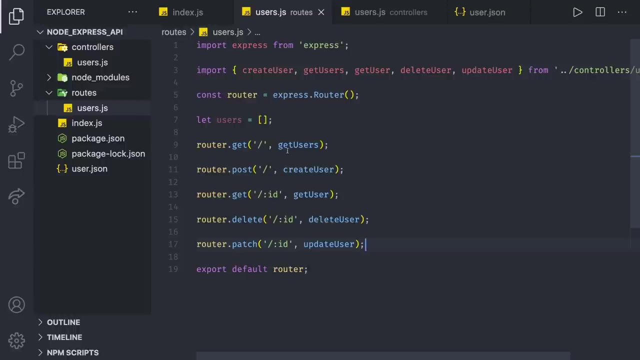 which we just copied right there. now you can see we have all the logic for our handlers right there, all the functions. you can even collapse them like this. and now in the routes, see how simple this looks. now we only have the routes here, but here, just so you can see, we also. this is a very simple method of getting. 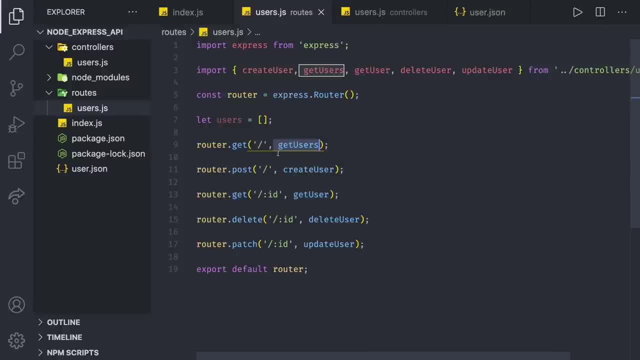 users recognized of the first function right here. so we have our hunting user and then we also have the delete user function, and then we do repeat the same operations in the command function, because by default the syntax of this function doesn't work that much. but you can set the neder dimension. if you think, guys, some of the many things we are going to cover. 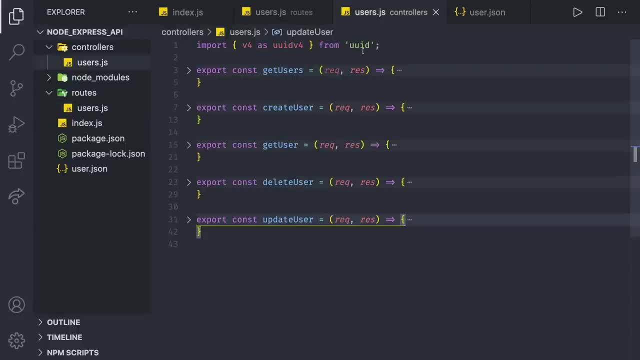 are already here, we also need to set some compliment to it. so let's just drag all these values right now and pass cookies. we'll pull a few. that comes to mind. space, that i've already written down here. so let's. and also move it to the controllers just at the top. Great, That's it. Now let's give our 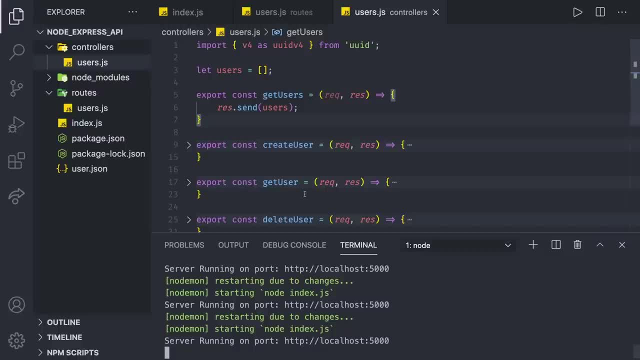 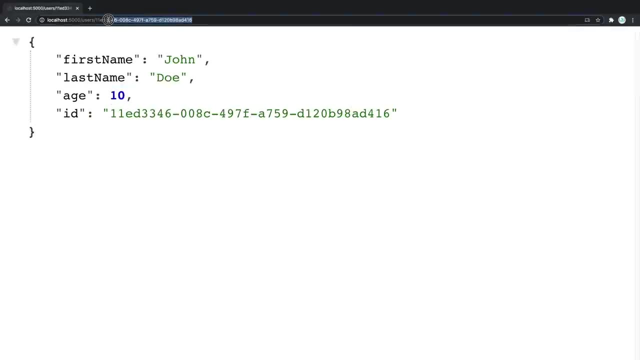 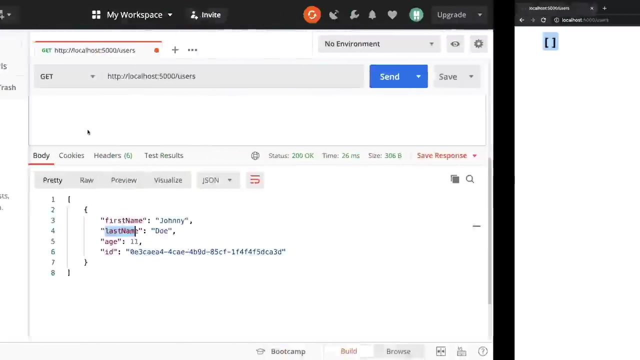 application. one last test: Let's go to our local host and see if everything works perfectly, because we did change a lot of things. Okay, starting with the browser, if we do make a get request to slash users, we do see an empty array. Now in the postman, let's make a post request to create. 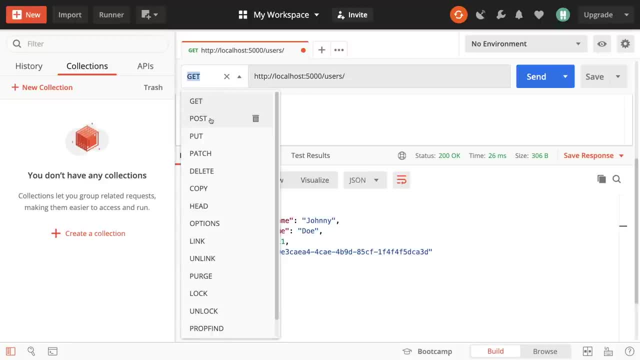 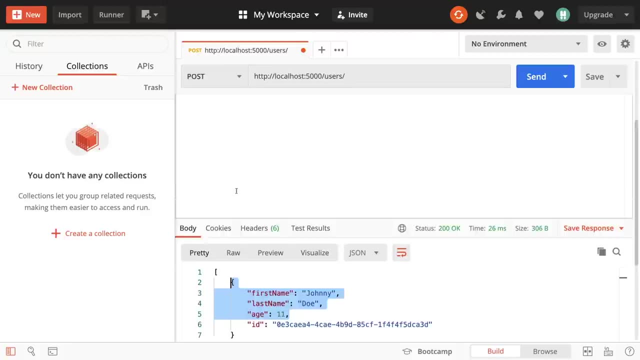 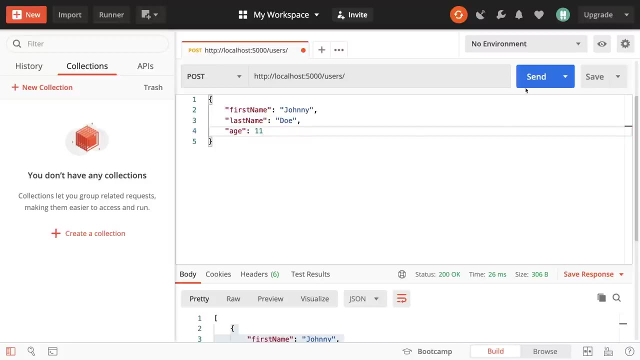 a few users. So, inside of the postman, make a post request and let's take the data for one specific user. In this case, I'm just going to copy this Johnny one and have it like this: There we have the Johnny and let's add him. So I do post request. send user Johnny. added to the 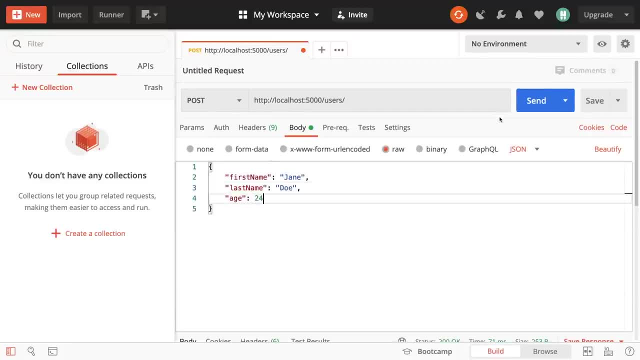 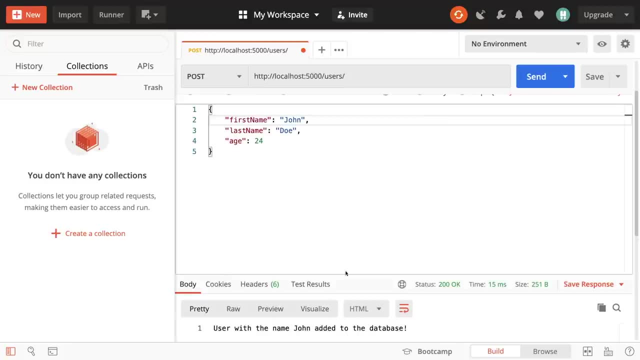 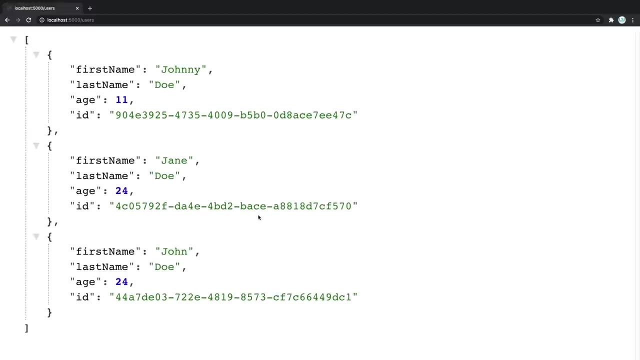 database. Let's add Jane as well and finally we can add John. Okay, user John added. Now we can go back to the browser refresh and we indeed do see all three users in the database. Great, So what can? 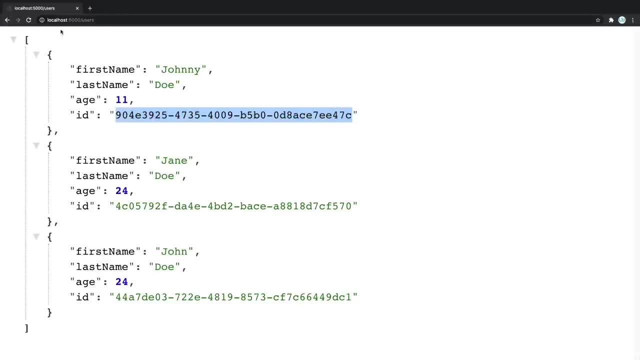 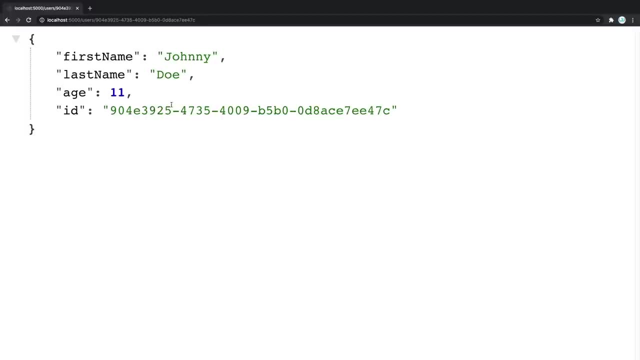 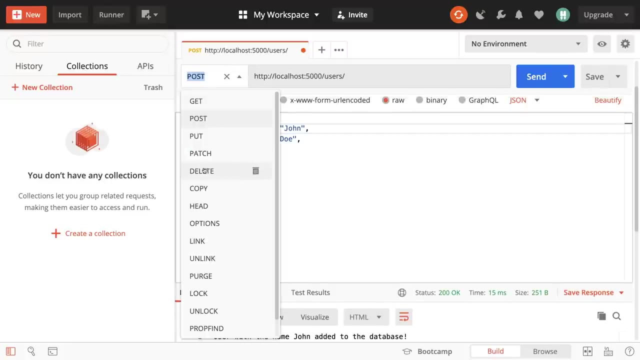 we do with them. Let's take the ID and let's go to slash users. slash that ID. Then we get the information only for that specific user. What else can we do? Well, if we go here and now try to delete a user, I'm going to do the delete. 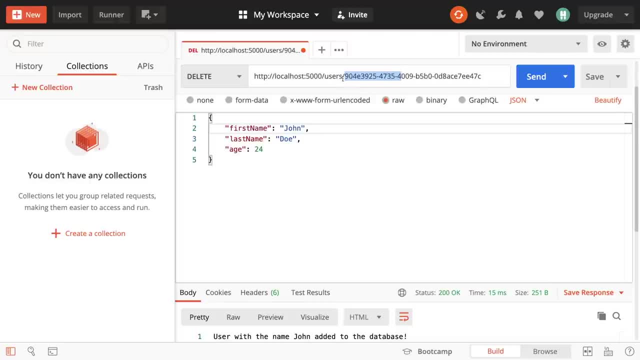 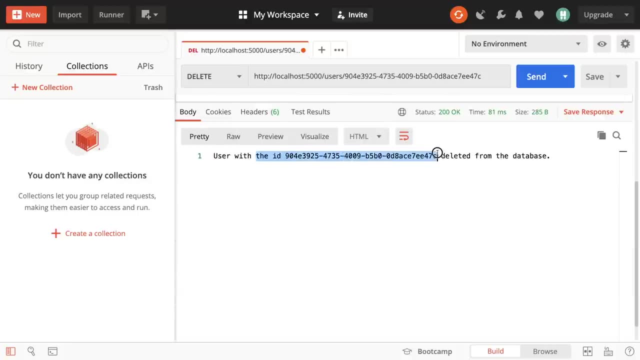 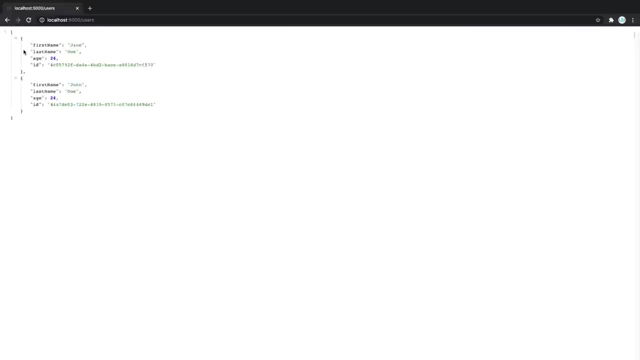 route and then add the ID after the users in the path run the function and, as you can see, user with the ID deleted from the database. How can we be sure that that happened? We go back here to slash, users make a get request and you can see we only have Jane and John and the last thing to 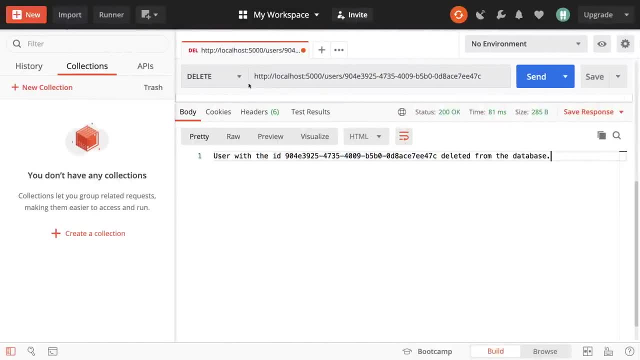 test out would be if we can actually modify a user. To do that, we're going to make a patch request to a specific user's ID. We cannot do this one because we just deleted it, So we need to take a new one. Let's do Jane, for example, and modify it here and now. we need to send some data. Let's. 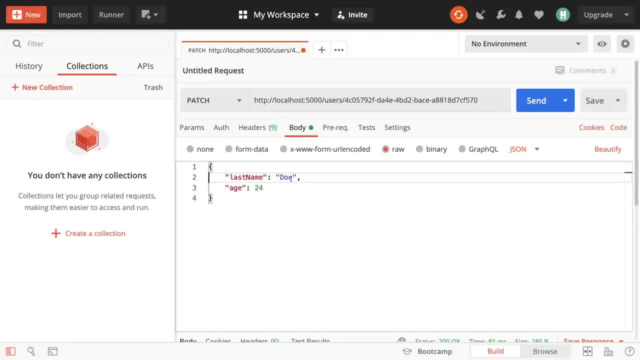 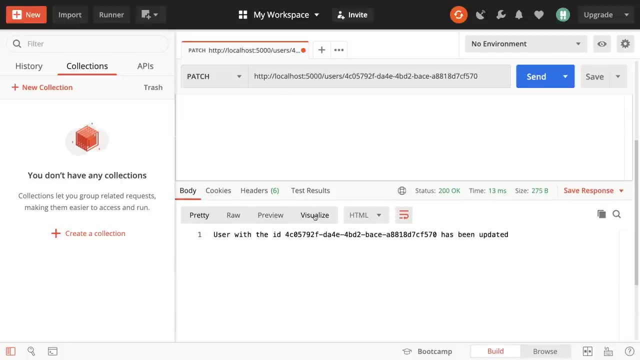 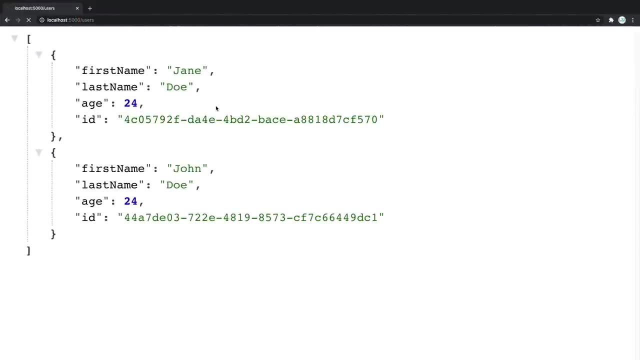 say that Jane remarried and now she's married to John, with two Es at the end of the surname. Let's do that and let's save it. As you can see, user with the ID has been updated and now, if we go back to the users, save it. you can. 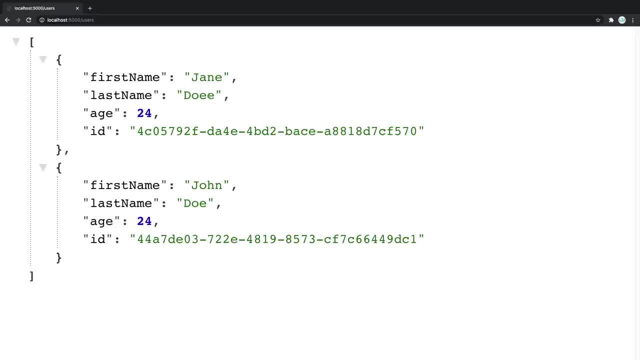 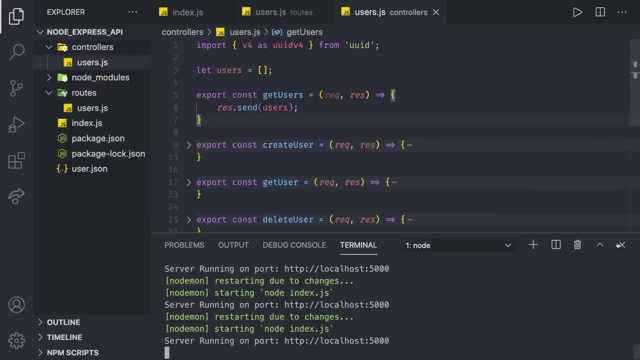 see, it's still Jane, the age is still 24, but now the last name has changed, which means that our update function works perfectly. And there you have it. This is the full application. As you can see, the file structure is not that bad. We have the indexjs file with the setup of the server.